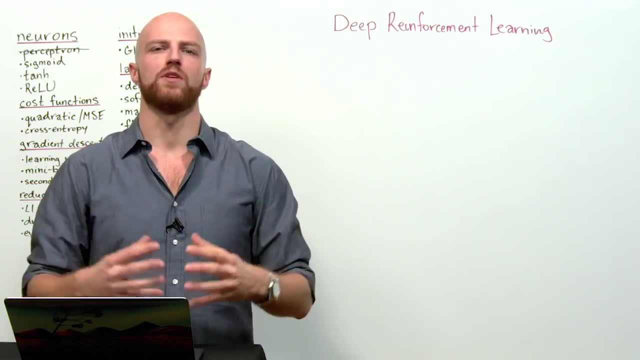 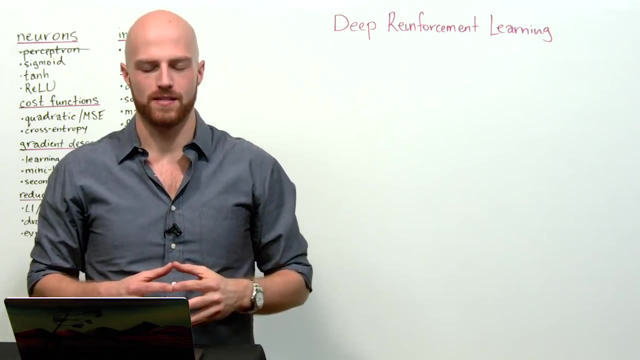 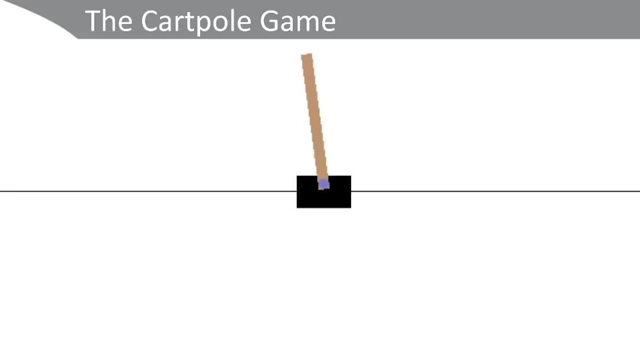 game that we're going to be training our deep reinforcement learning algorithms to play. It's a super simple game. It was invented in the 80s out of Richard Sutton's group at the University of Alberta And it's called the Cart Pole Game. So the Cart Pole Game is really simple. It involves 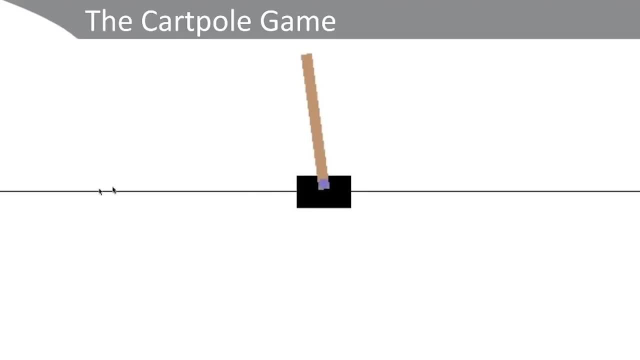 this cart moving in one dimension back and forth on this line And this cart is supporting a pole. They're connected at this blue dot. I'll show it in action in a moment. But the idea here, the way that you win the Cart Pole Game, is that you're going to be playing a. 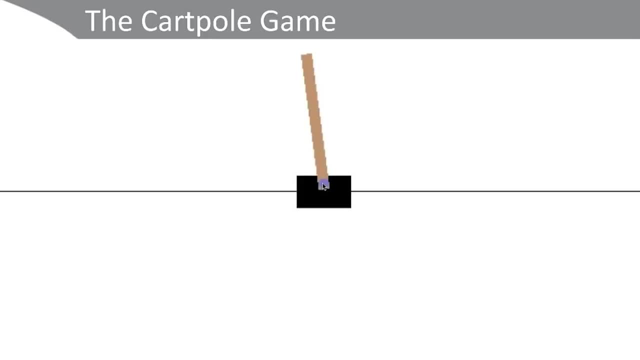 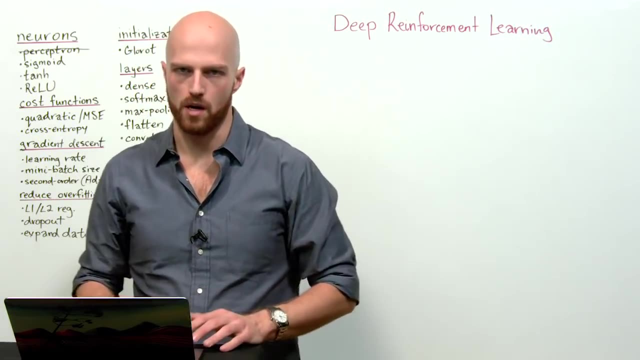 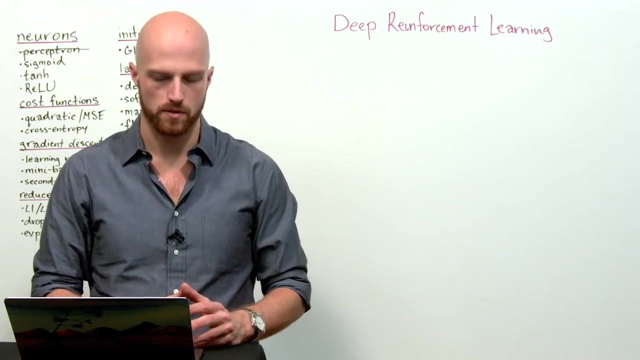 cart And what you're going to do is by balancing the pole on top of the cart so that it doesn't fall down. The target number of frames in version 0 of the Cart Pole Game, which we'll be playing, is to keep that pole up for 195 frames of the game. So there's two ways that. 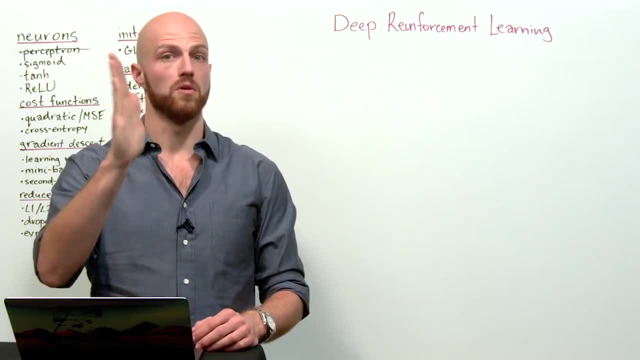 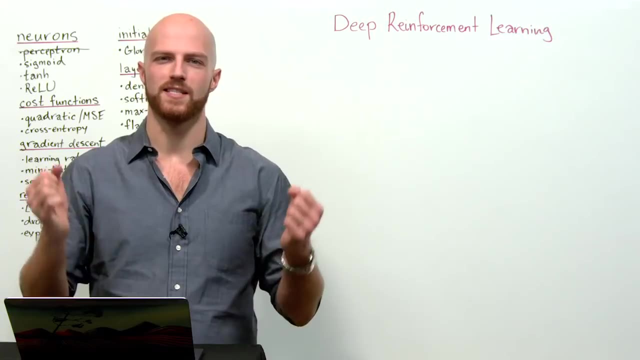 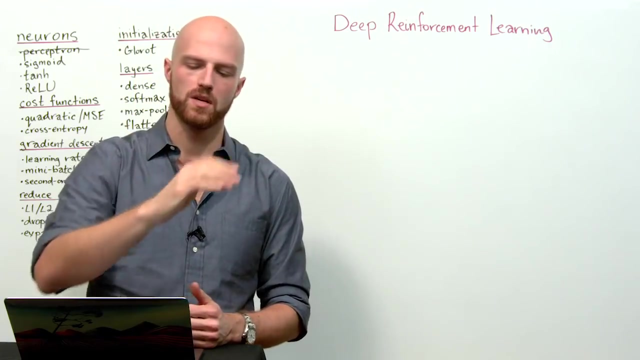 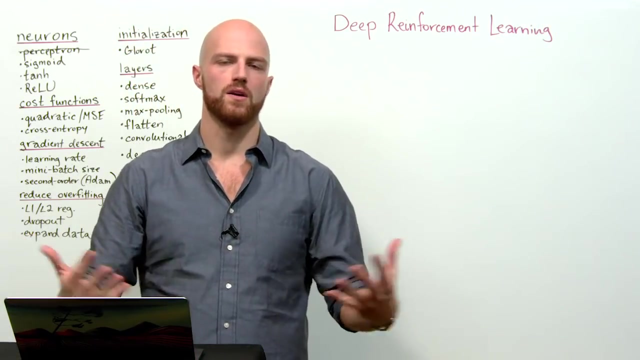 the game can end. The first way is by keeping the pole up for 195 frames, for 195 time steps. The other way that it ends is if you die, And the way that you die is by having the pole fall off. So there are four pieces of information, The reason why we use the Cart. 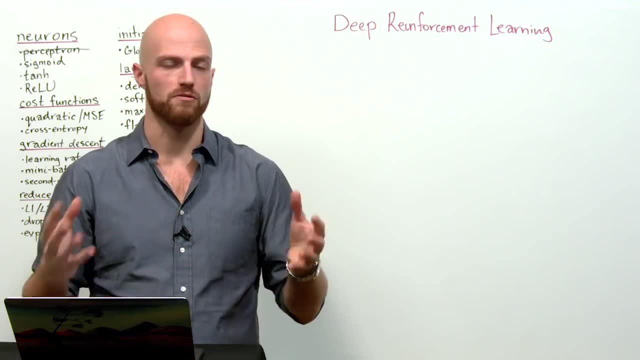 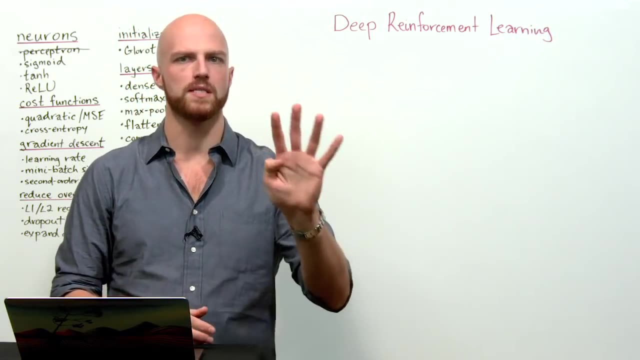 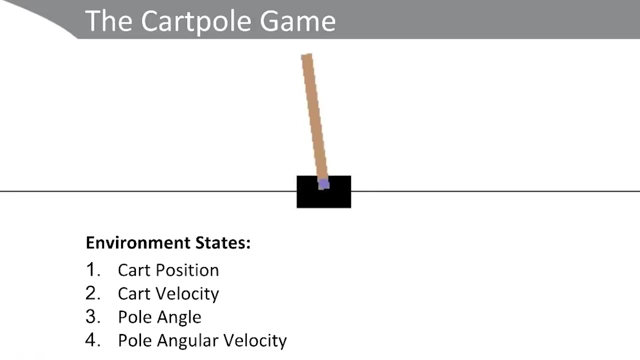 Pole Game as our game for training our deep reinforcement learning agents is that the number of states in the environment is very small. There's only four pieces of information that you need to get from the environment. There's the position of the cart, So where? 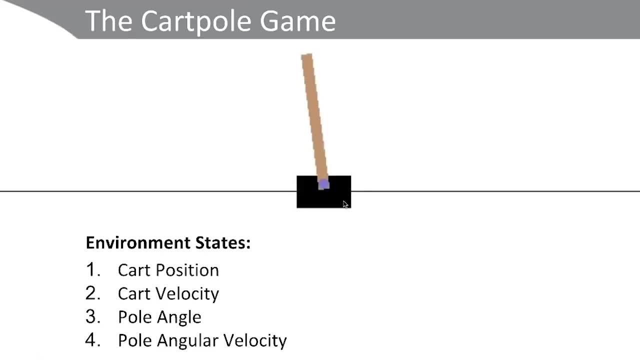 on this one-dimensional axis is the cart, What's its position, What's its velocity? So, how quickly is the cart pole moving left or right? What is the angle of the pole And what is the velocity, the angular velocity of the pole? 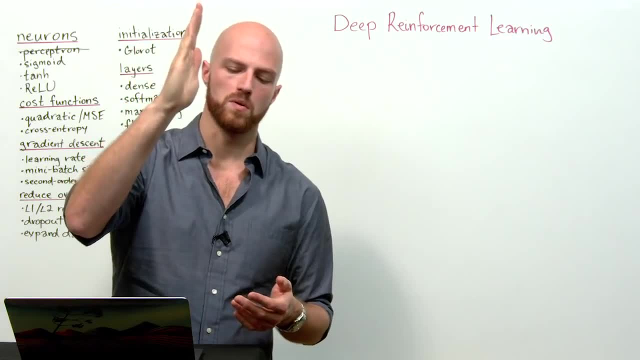 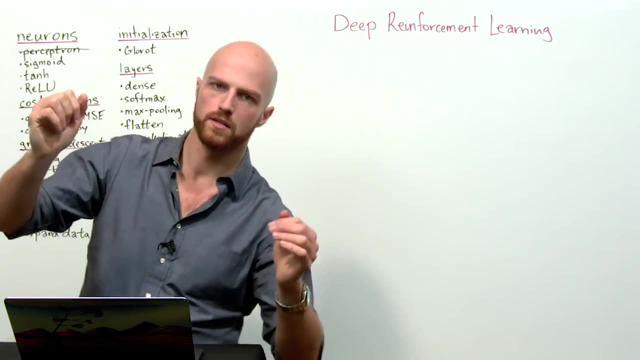 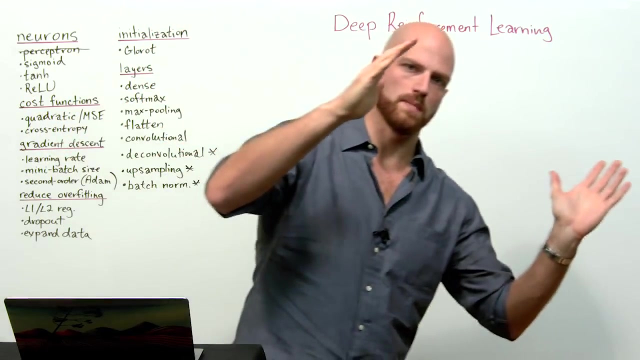 So the more, The more that the pole starts to develop an angle or angular velocity, the more likely it is that you'll lose the game and the harder it is for the cart to stay under it. So the name of the game is just kind of balancing. You can also, if you end up tipping off the 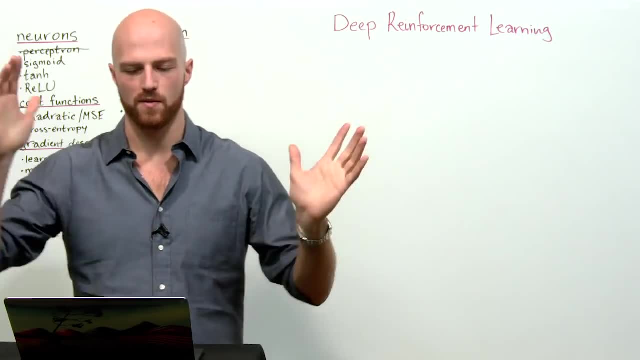 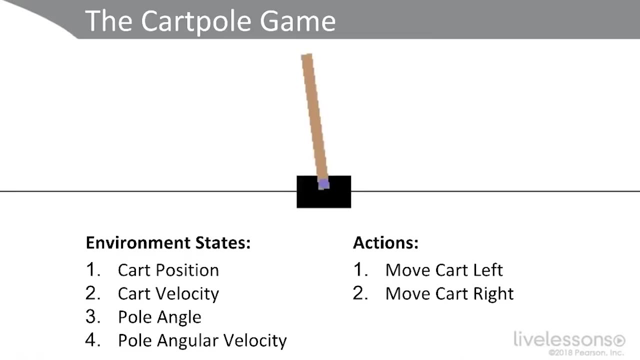 screen one way or the other- that's another way- you can die too. So you kind of want to keep the pole centered and balanced nicely there on the cart. There's only two actions that our agent can take in this game, That's to move the cart to the left or to the right. So a zero or a one is the two possible. 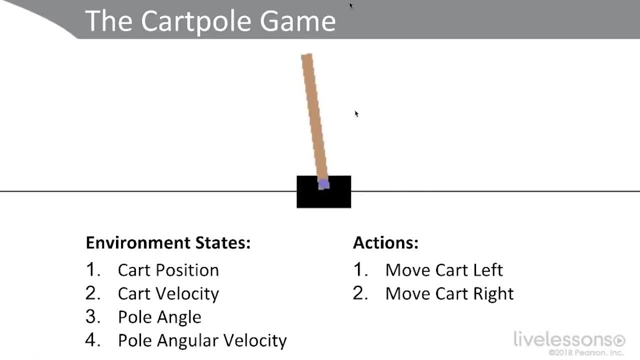 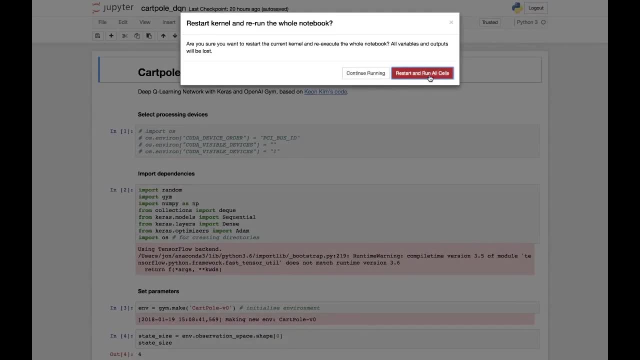 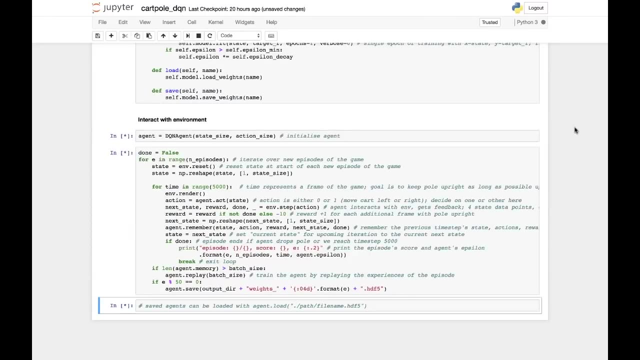 different actions. Let us have a look at this guy in action. So I'm just going to run the DQN notebook that we're going to build over the course of this lesson. I just want to show you guys how this works. So here is the game in action. 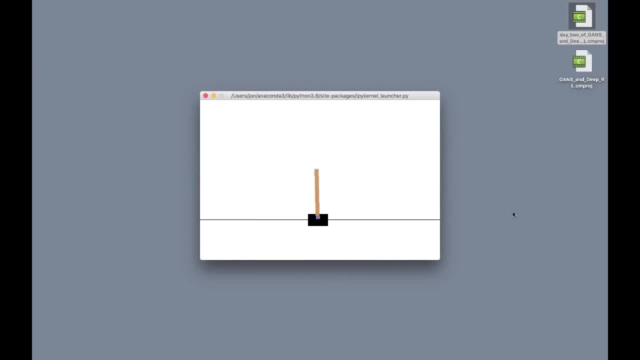 So you've got the pole, and this is just playing game after game back to back, So it's kind of difficult to tell where one game ends and the next one begins. but essentially any time the pole starts to fall, the game just stops and we're starting again with a new episode. 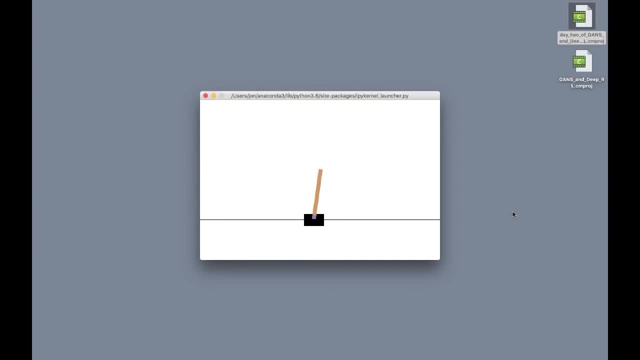 of the game. So each of these episodes provides an opportunity for the pole to train, And we can see here, even early on it's actually training from scratch. We can see already, after only a few dozen trials it's starting to, Every once in a while, manage to keep the pole upright. 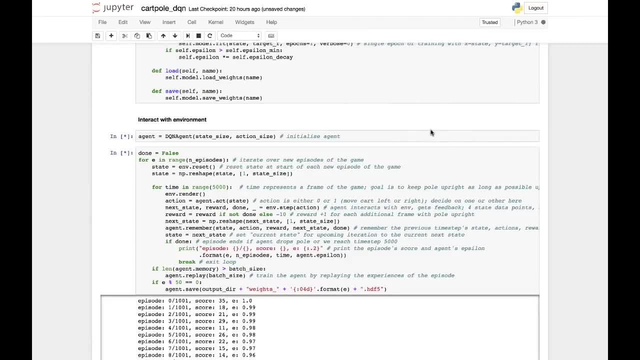 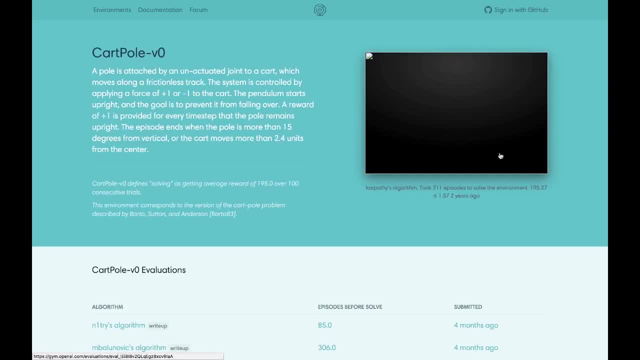 Okay, so that's our goal. That's our goal. That's what we're trying to get to over the course of this lesson. Now we have a lot of steps to get there. Let's first have a look at the OpenAI Gym website. 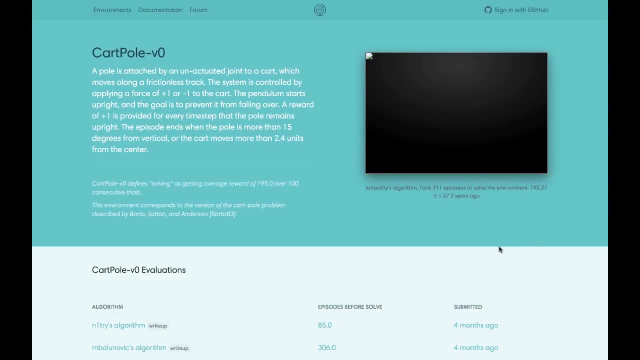 So the OpenAI Gym is the source of this environment interface for our agents. So the OpenAI Gym provides a bunch of different environments. It's a lot more complex than the Carpool game, So we're just going to start with the Carpool. 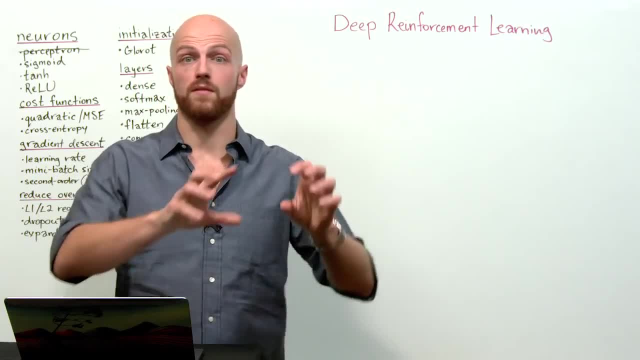 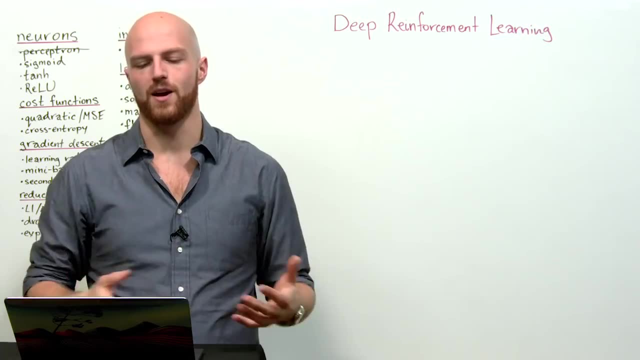 game today. Many of them are really complex, like Atari games where the environment state is all of the pixels on the video game screen. So obviously that's a lot more complex to train up an algorithm to perform well than just having these four states of the environment. 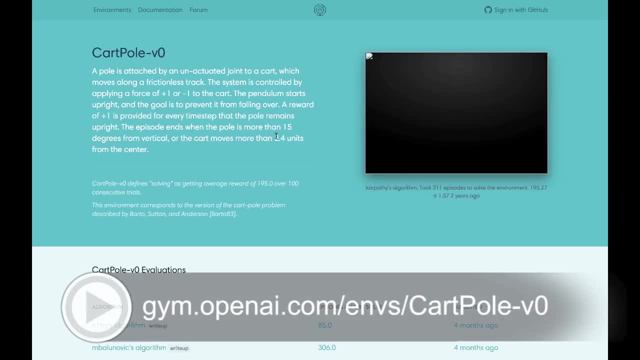 that we need to keep track of. So, as it states here, the episode ends when the pole is more than 15 degrees Okay From vertical, or if it moves more than 2.4 units from the center. So that's going off the screen. 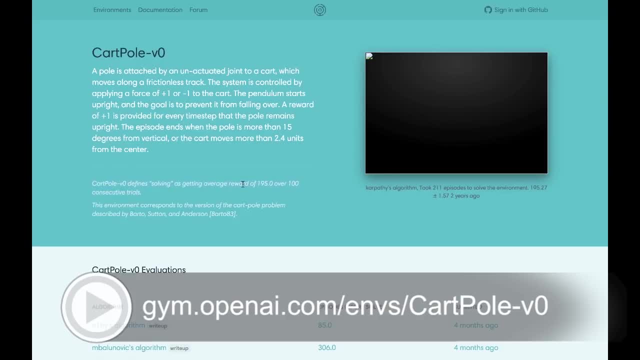 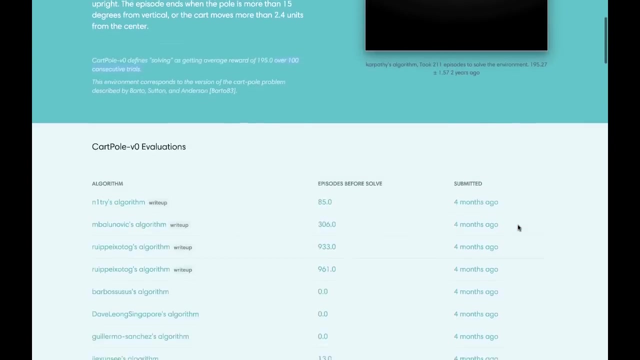 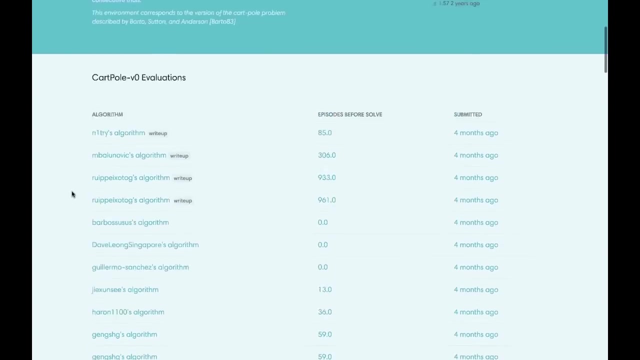 And you win the game. You solve the game by getting an average reward, so managing to keep the pole upright for 195 frames on average, over 100 consecutive trials. So you can see people's algorithms for playing this game. So some people have solved it in. it took 85 episodes for the algorithm to become proficient at. 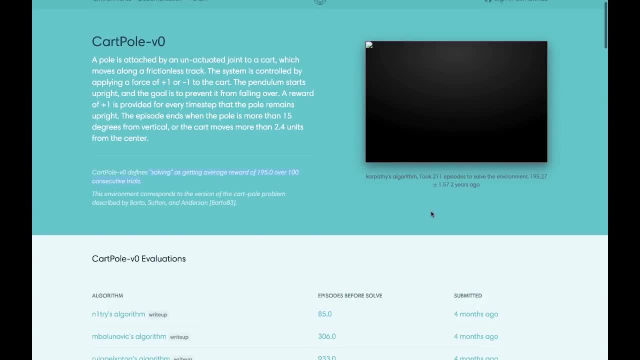 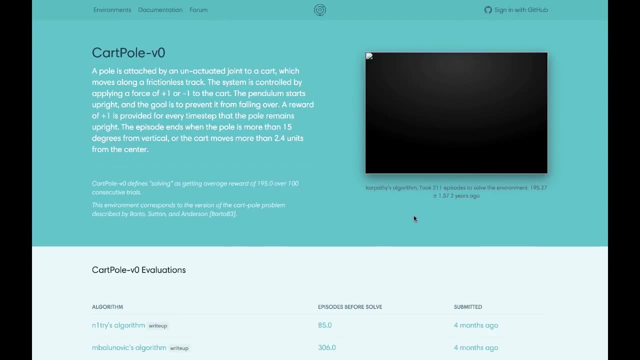 this task and be able to solve the game. Andrej Karpathy, who is a very famous deep learning researcher, he two years ago it took him 211 episodes, to average above 195.. And you can actually go: click through. 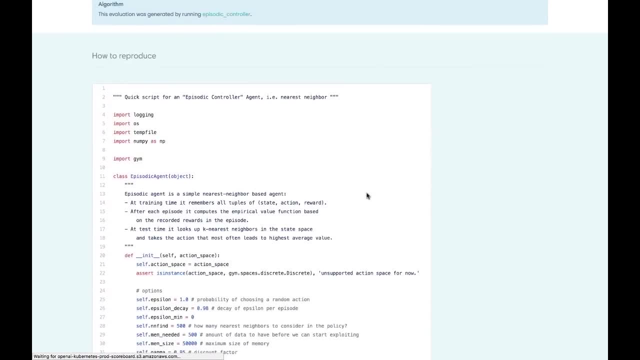 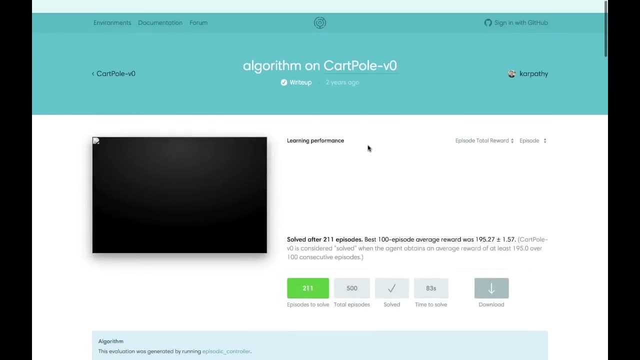 Okay, And look at his or anybody else's algorithm: their agent for playing the game. So here's a look at, you know, an agent. We're going to be making a simpler version of an agent today, But this is a fun. 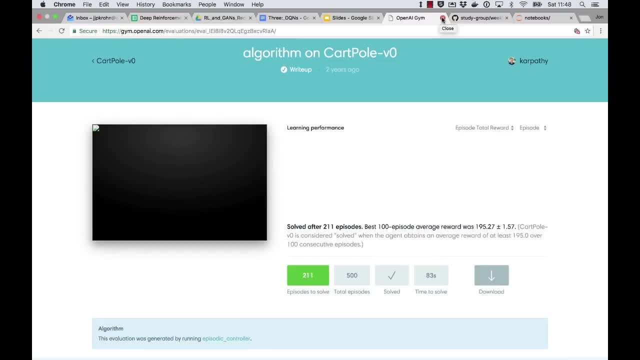 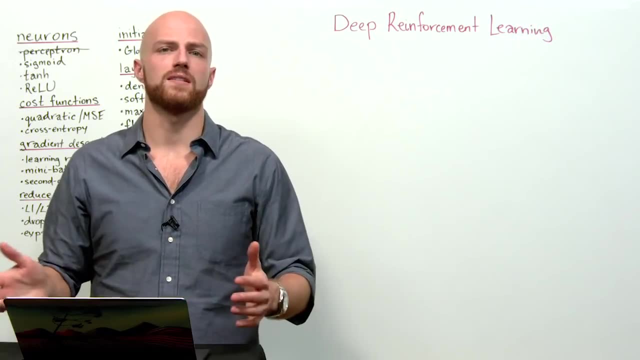 way that you can explore how various other people have set benchmarks and you know the differences between their algorithms. So that's the Card Bowl game. Now we're going to dive into some theory so that we can figure out how to build our own agent for winning. 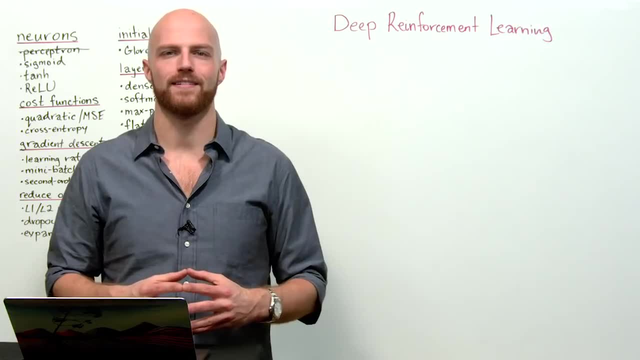 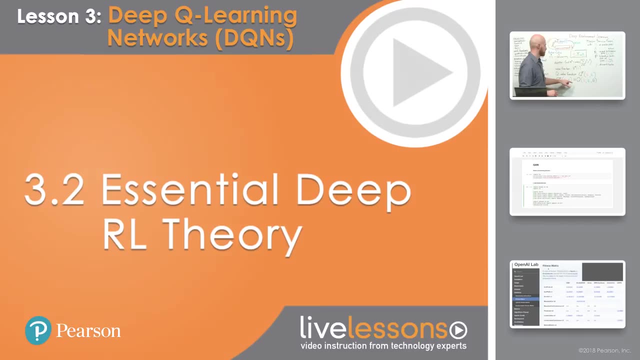 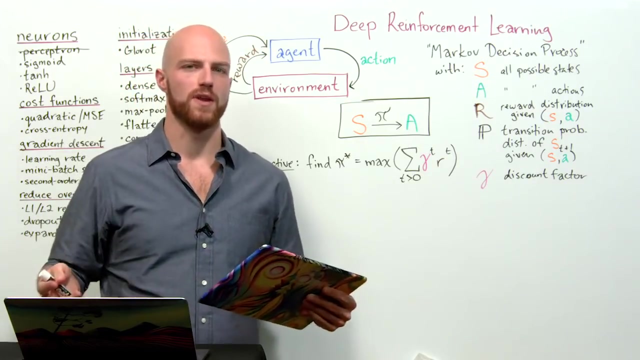 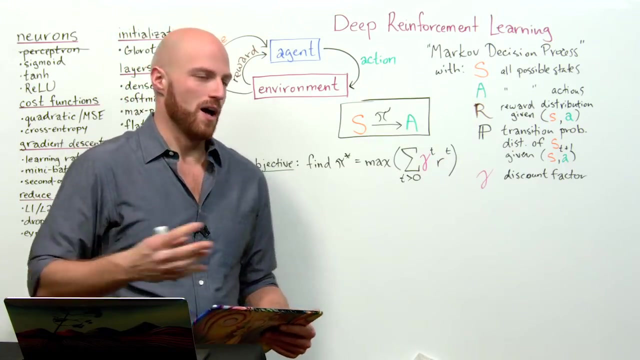 So start around the Card Bowl game. We're going to dive into the Card Bowl game. We're going to give an example of the Card Bowl game for winning the Card Bowl game ourselves. Let's get into that, All right. So we want to solve the Card Bowl game or any other kind of game that is thrown at us, any kind of. 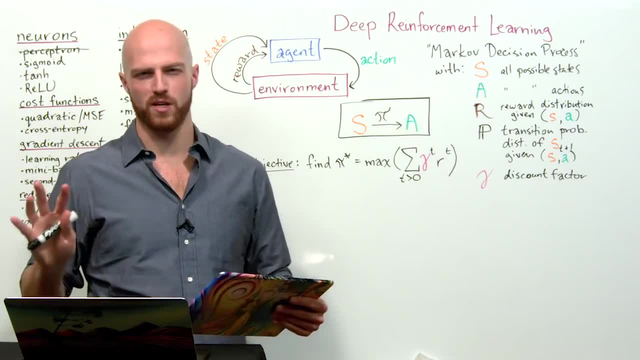 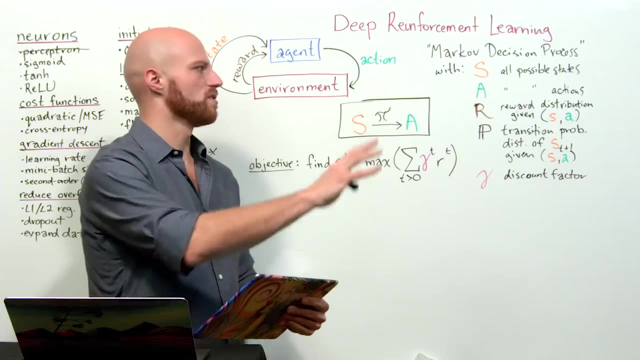 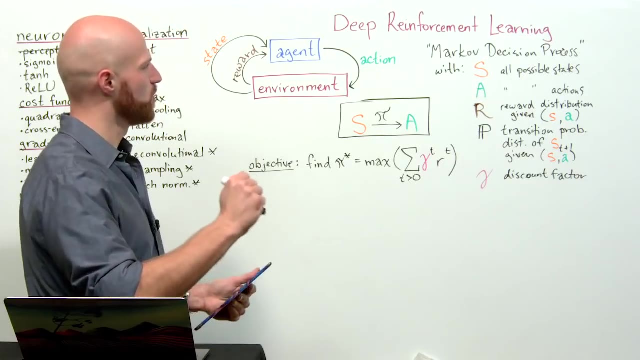 environment that we want to solve with our deep reinforcement learning algorithm. math to a minimum, So bear with me here. We just need to cover enough kinds of terms that we can start writing our code, and the code will make some sense to us as we get going. So this is a diagram. 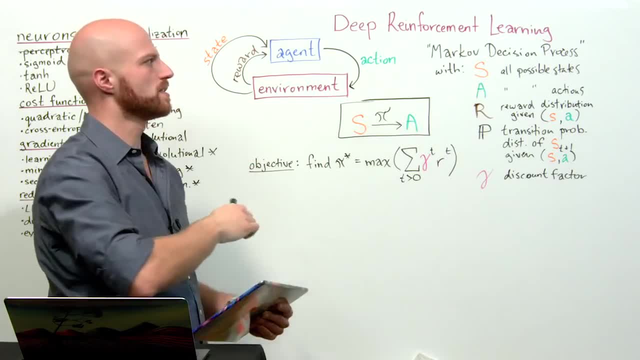 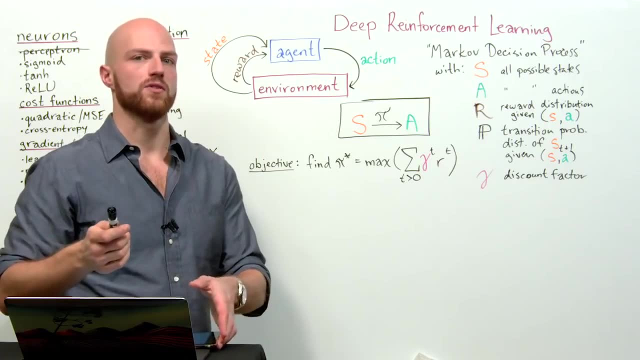 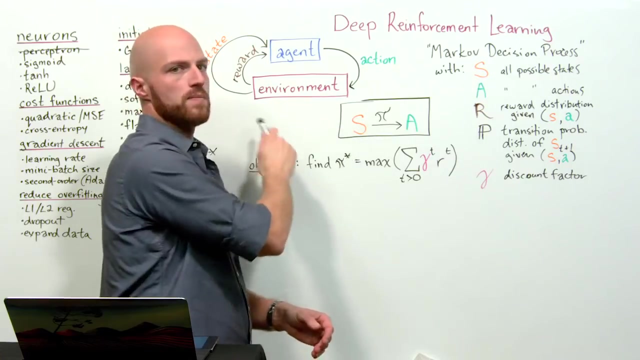 that I drew already earlier in these live lessons. This is the main concept of reinforcement learning. We have some agent which is, in our case, going to be a deep reinforcement learning algorithm. This agent takes action in an environment, which, in our case, is the carpool. 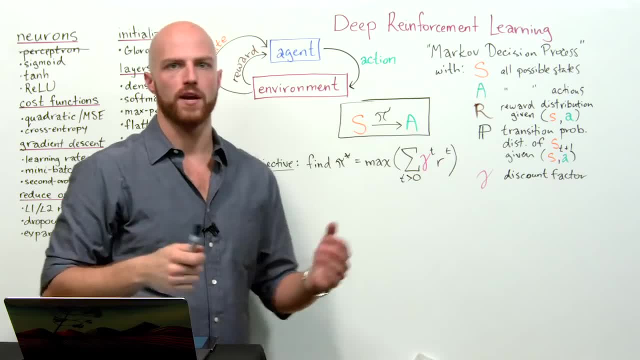 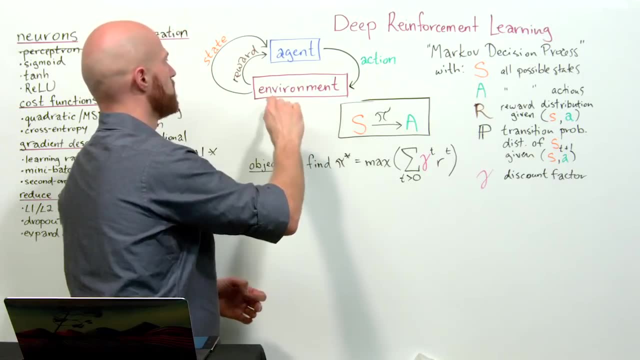 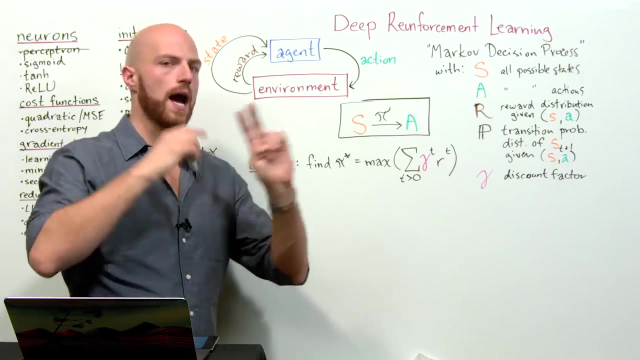 game. There's two possible actions that our agent can take, That's to move right or to move left, And then the environment provides the agent with feedback. So it provides two kinds of information as feedback. The first kind of information is the feedback that the agent is providing. So the first kind of 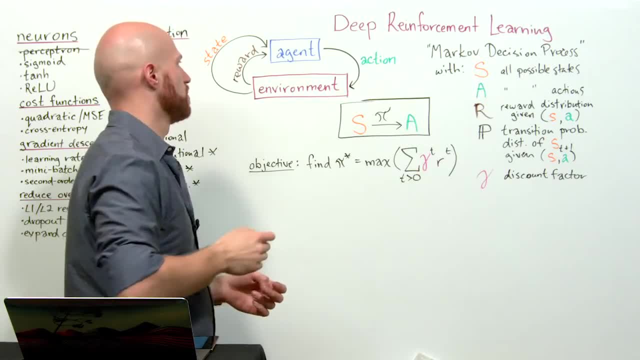 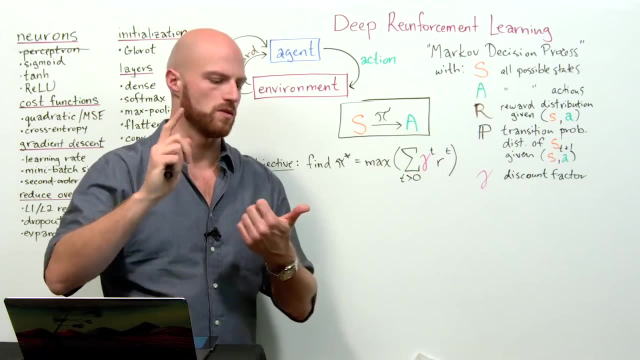 information is the feedback that the agent is providing. So the first kind of information is the state. So this is the four pieces of information about the environment, So the location of the cart, the velocity of the cart, the angle of the pole and the. 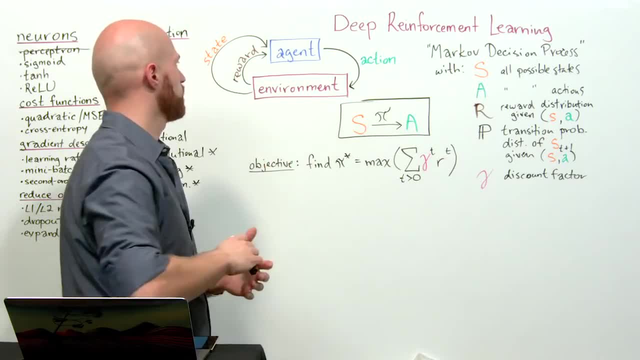 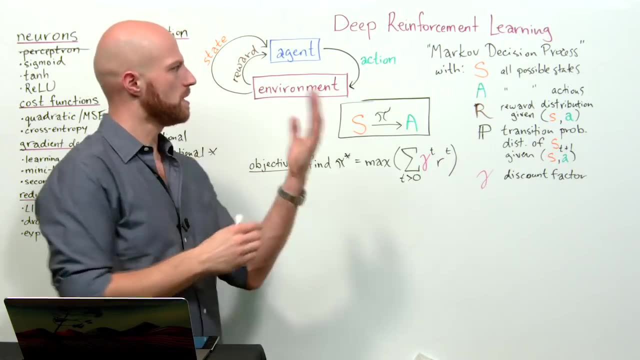 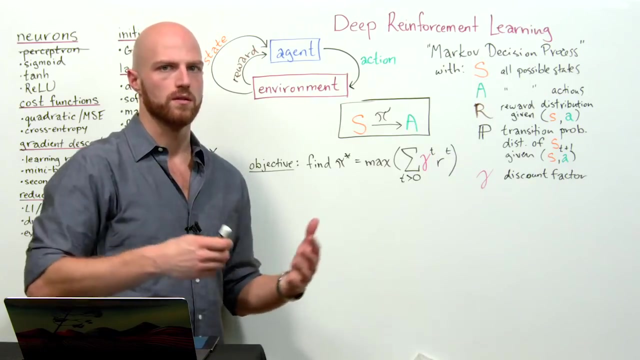 angular velocity of the pole. So these are the four states that are fed back. And then our reward- that we're trying to maximize- is to keep the pole upright for as many time steps as possible. So the more time steps we're up for, the larger the reward. 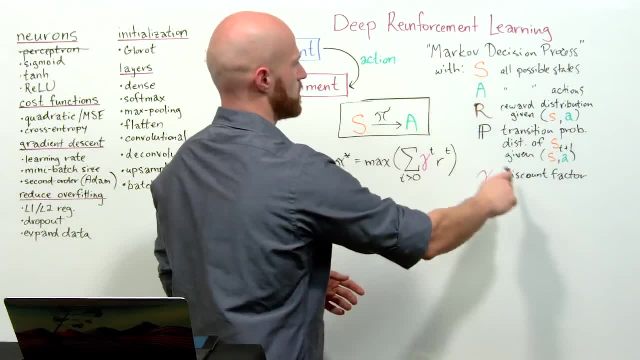 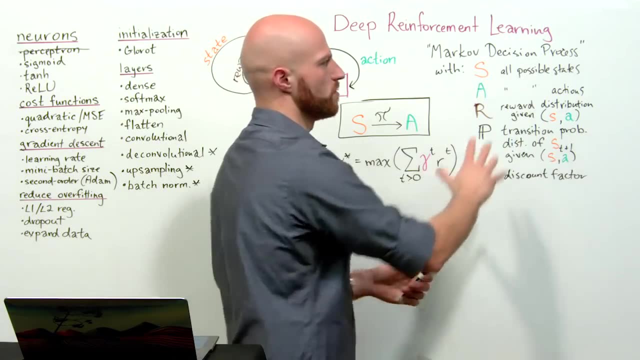 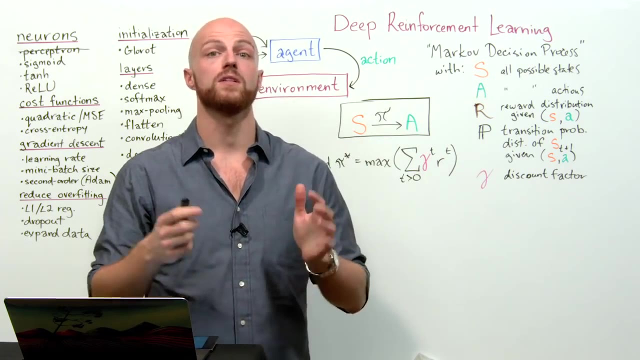 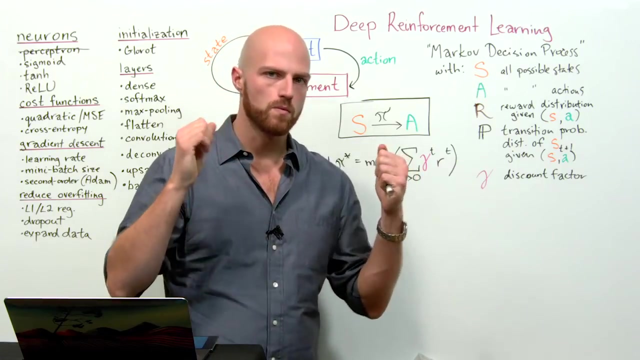 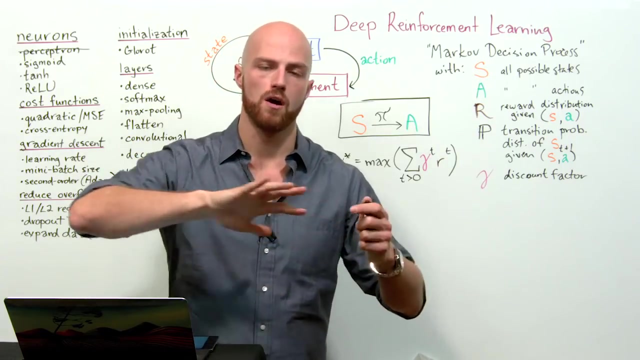 So we can define this idea, this little diagram. we can define that more formally as this set of terms over here. So this paradigm, we can call it a Markov decision process, And the trademark of any Markov decision process is that we assume that the current state of the world at any given time step is representative of 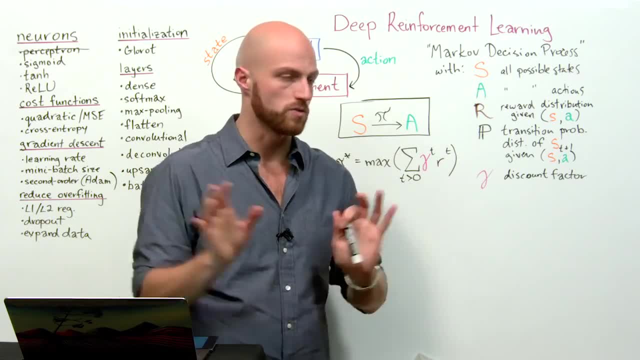 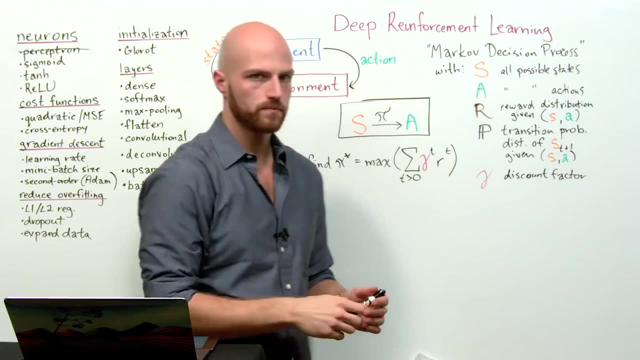 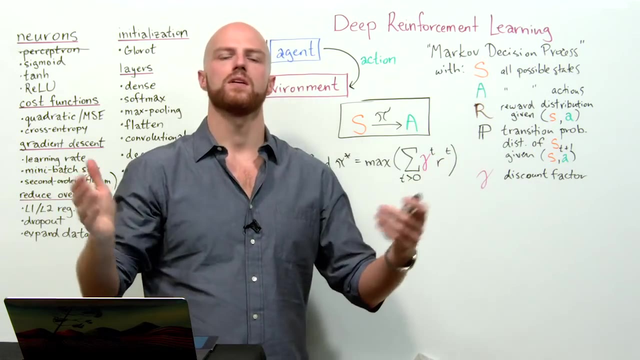 all of the time, steps that have come before. So that's what a Markov decision process is, And then within our Markov decision process we have this set of information. So this capital S represents all of the possible states. So in the card poll game, this is all of the possible. 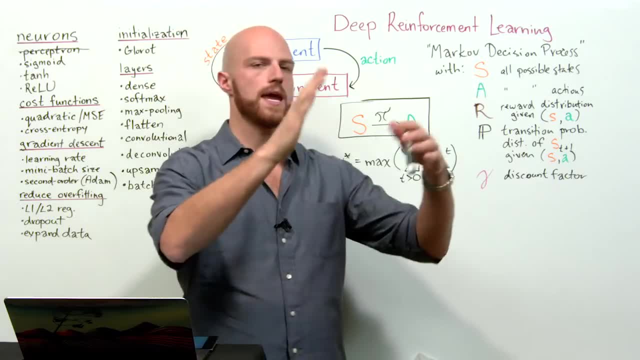 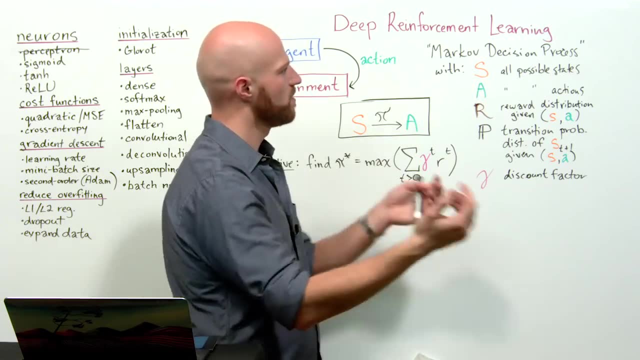 states that have come before. So this is all of the possible states that have come before. So in the card professions it's all of the possible use, CART locations and cart velocities, angular pole angles and pole angular velocity. So all of the possible states that it could have. 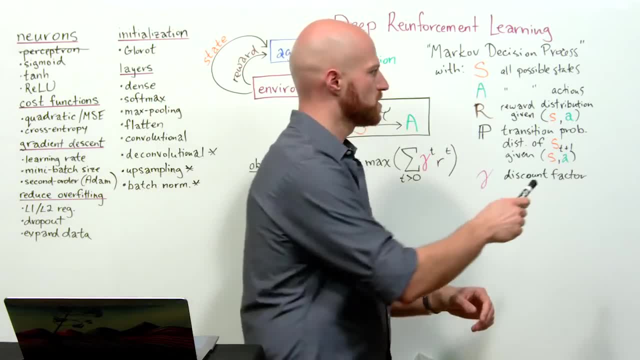 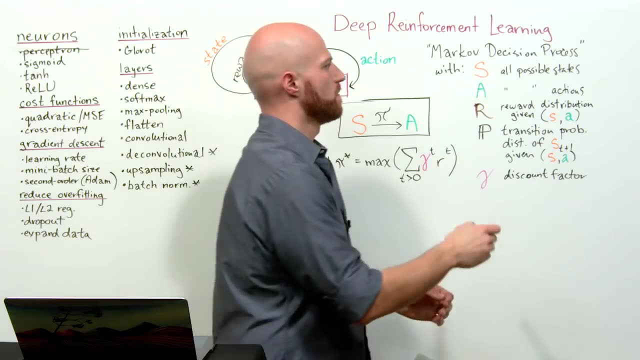 that each individual possible set of states is a lowercase s And then the upper case S is all of these states all together. Similarly, for the actions, a given specific action, so a specific move right or any particular move and any particular action or any particular action. 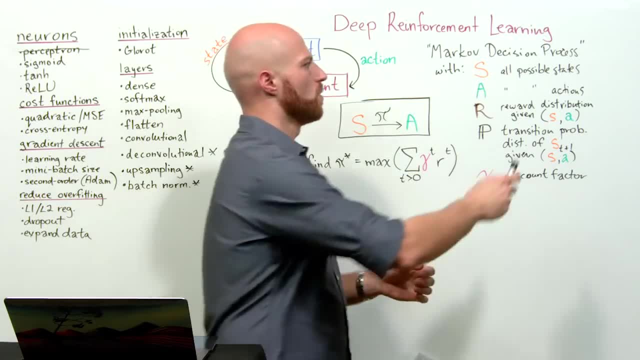 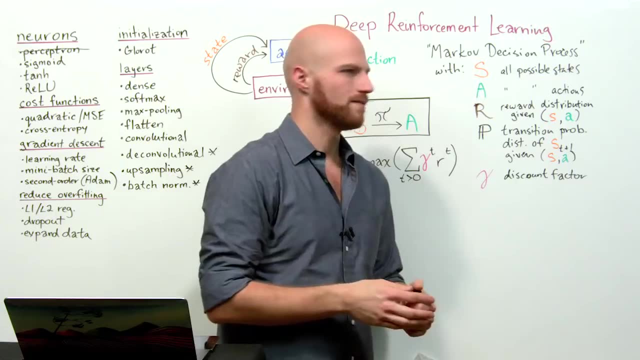 all of those are all in the same set of states. So a specific action or a specific move is a possible action move right or specific move left. This is a lowercase a and a is the set of all of our possible actions together, which in our case is just two possible actions Most games have. 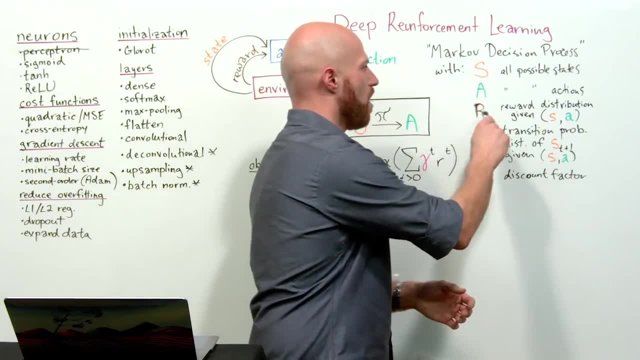 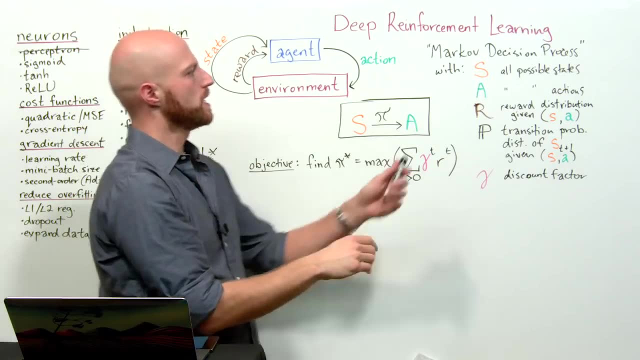 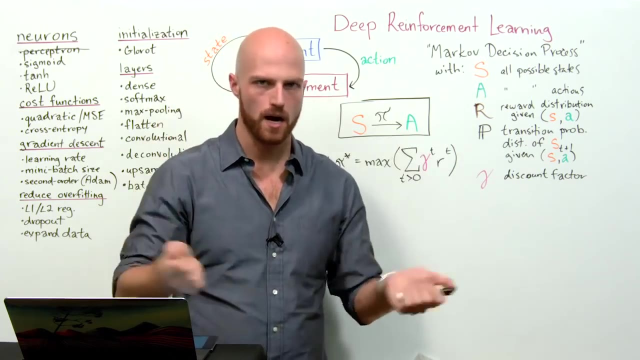 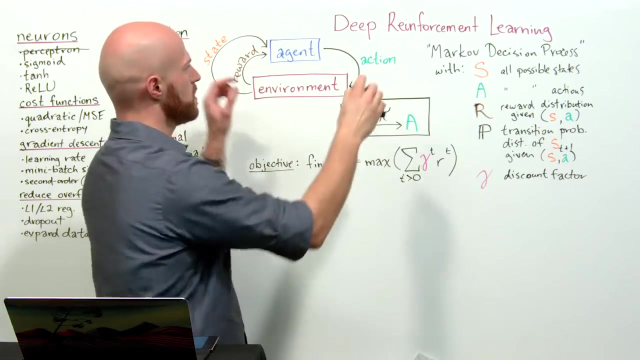 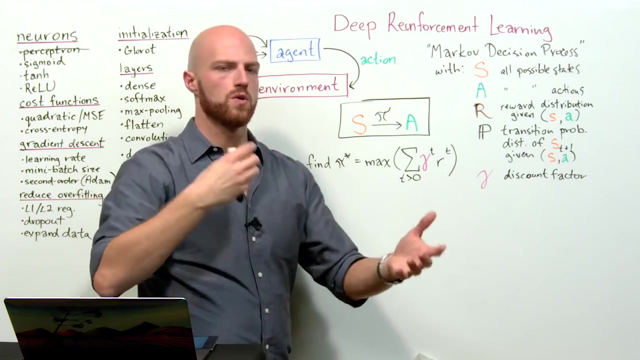 much more complexity. R is the distribution of the possible rewards that we can get back, given any single state and action. At any given time point, we can have an action that's taken and a state Given, the pair of these two states. what is the distribution of the reward? What's? 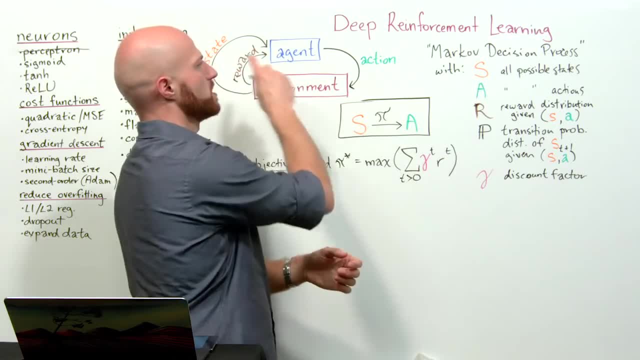 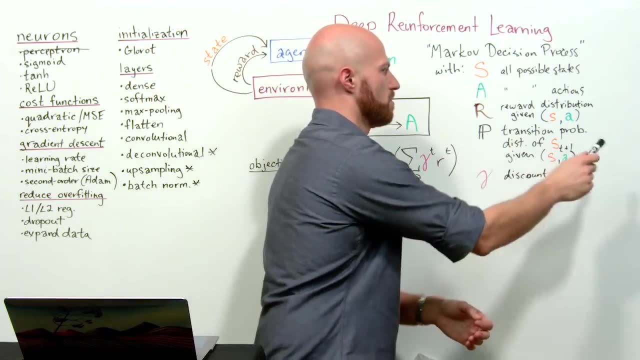 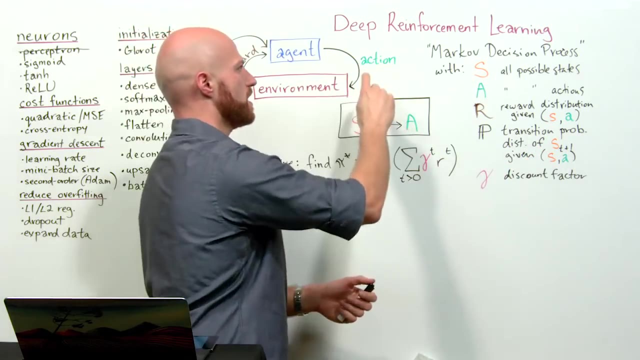 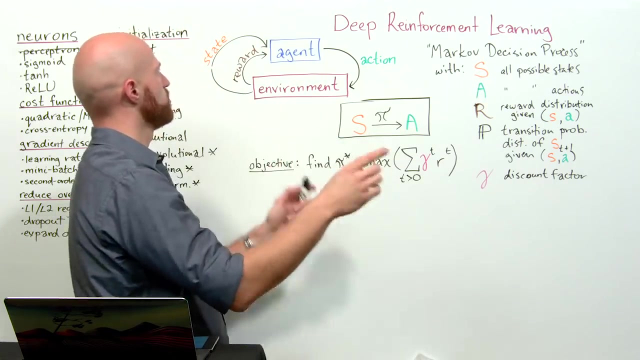 the possible rewards that we could get given a state and an action at a given time. step P is the transition probability distribution of the next state. This is given the last state and the action that we take in that state. This transition probability is the distribution of. 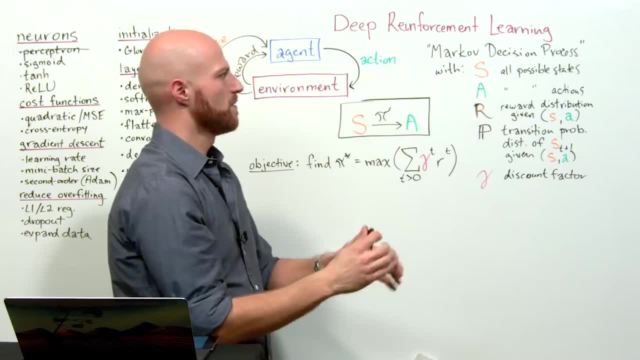 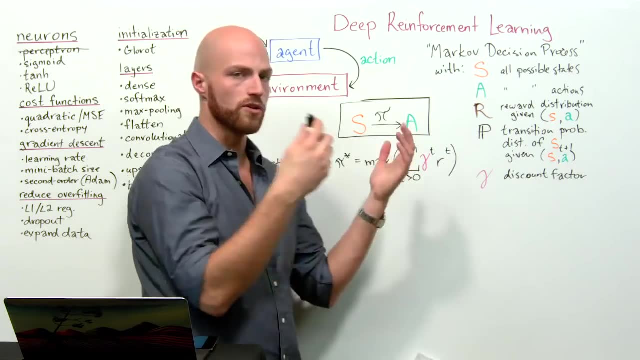 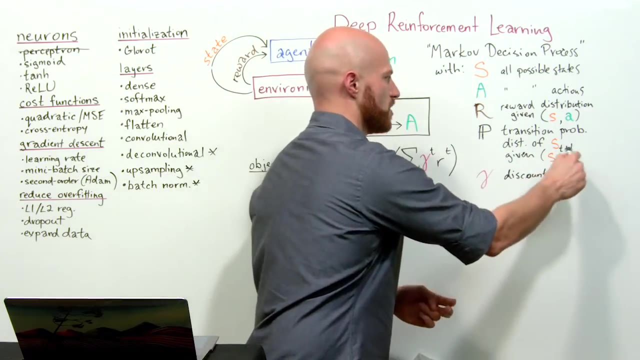 the states that we'll get. next. The algorithm, the agent: it gets a state. This would be the starting state of the environment or some state later on, after we've started playing the game, the agent takes some action and p is the. 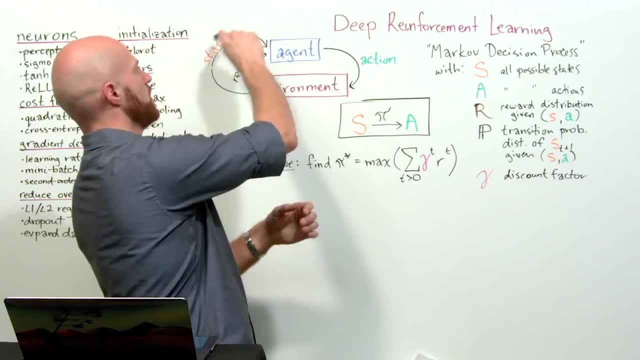 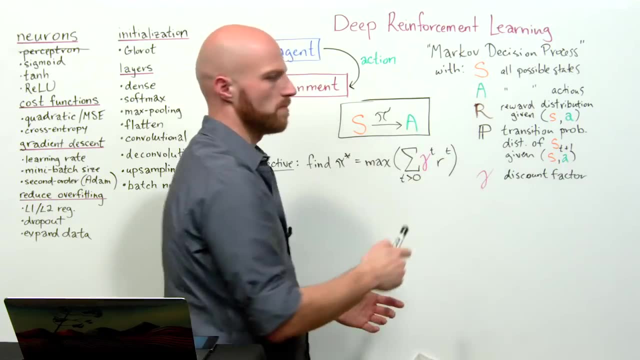 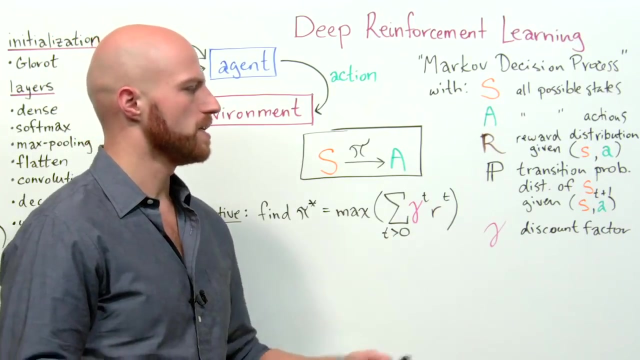 probability. it's a distribution of probabilities for the state in the next step And then, finally, the last term in this Markov decision process that we need to talk about is gamma, this discount factor. The discount factor is a hyper parameter that we set ourselves, And this is how much we 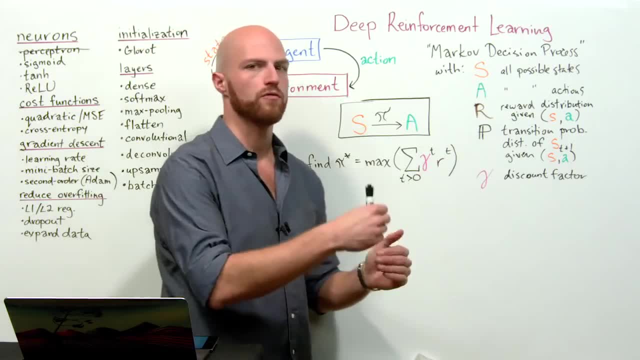 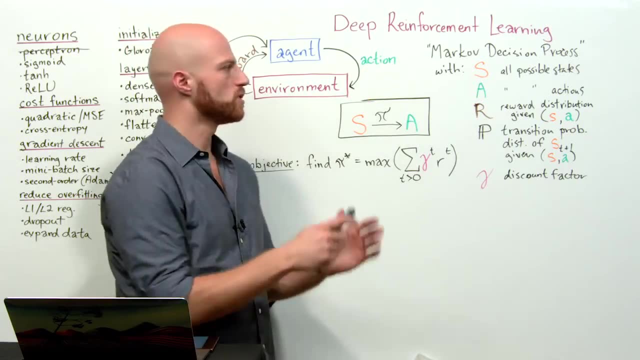 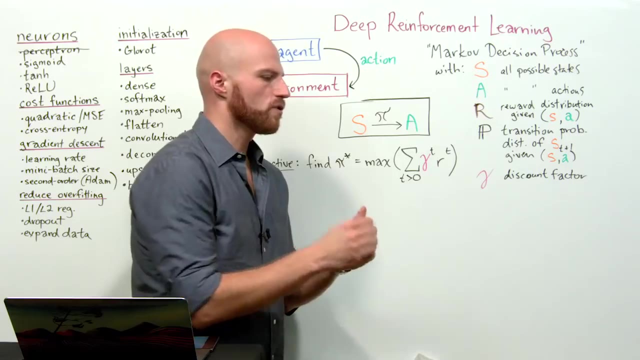 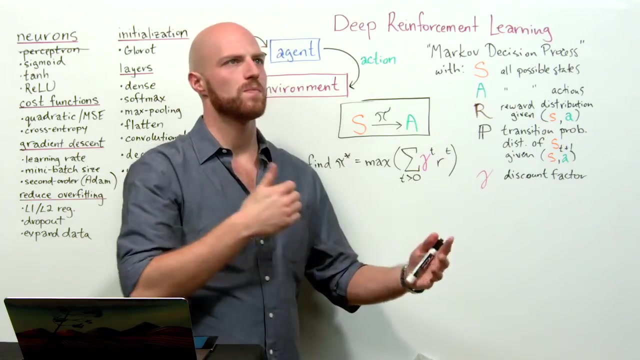 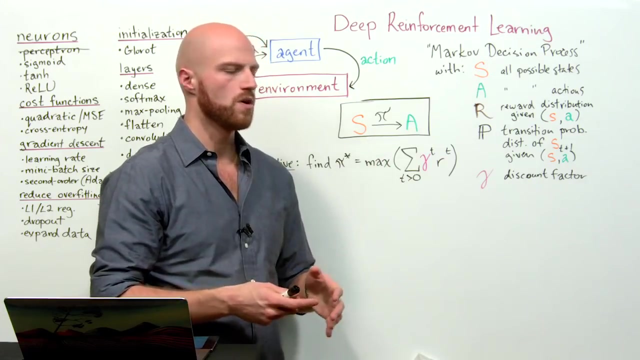 want the agent to discount future reward. So when our agent is considering any given action to take in the environment, it's going to try to take the action that maximizes its reward. The further that it tries to predict future reward, the less likely that reward is. So if you can imagine this kind of scenario where the algorithm 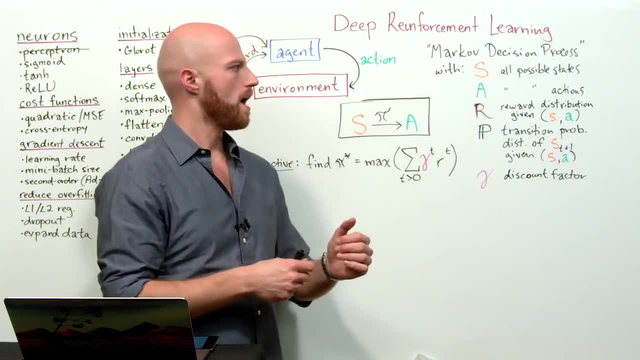 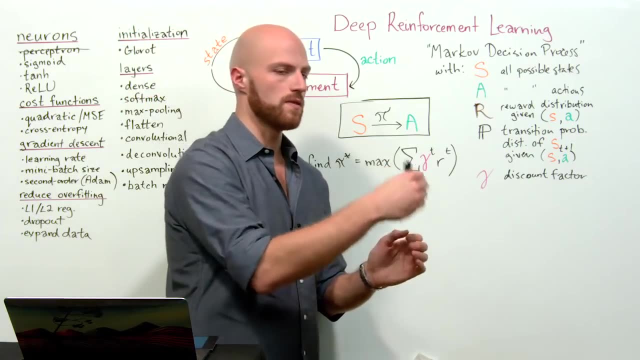 is thinking several steps ahead. and the very next step. it might have a pretty good sense of what kind of reward it's going to get, But then steps the further into the future those steps become, the more difficult it is to guess what the reward is going to be. So when our agent is considering any given action to take in the environment, it's going to try to predict future reward. So when our agent is considering any given action to take in the environment, it's going to try to guess what the reward will be. There's more. 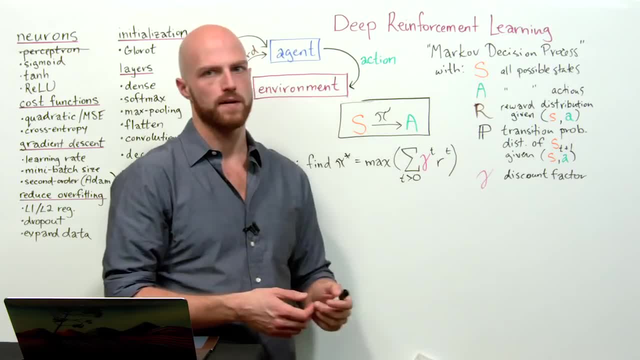 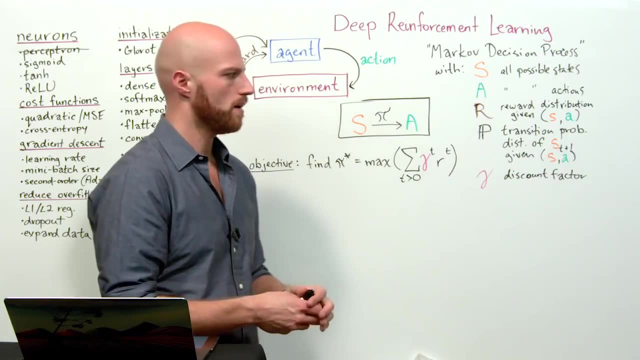 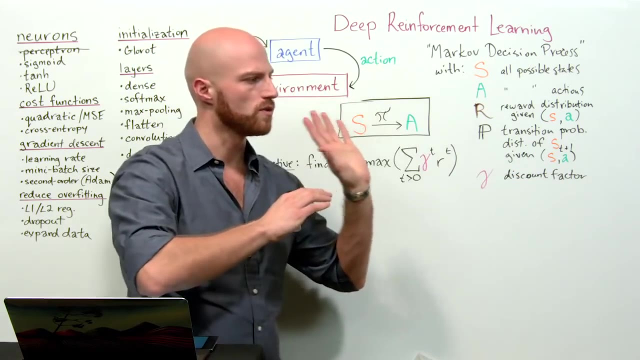 uncertainty. So this discount factor captures that, And so what this means is that the expected reward in the next time step is valued more highly than the expected reward in two time steps, three time steps, four time steps. So the further we try to predict into the future what our reward, 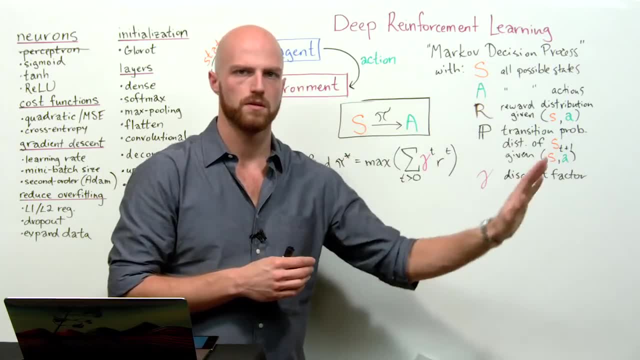 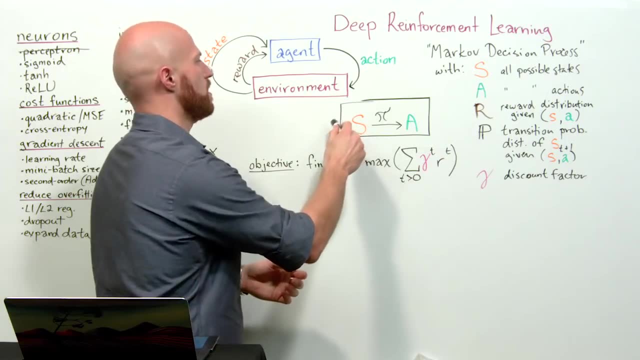 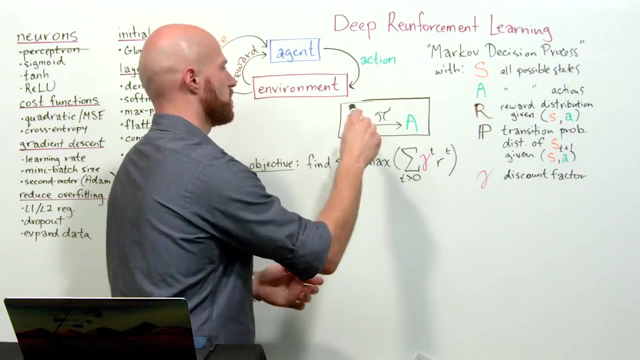 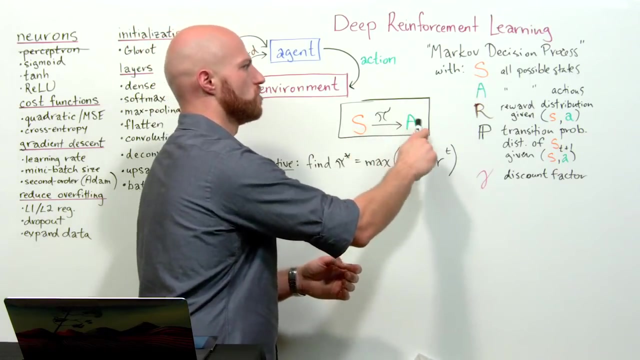 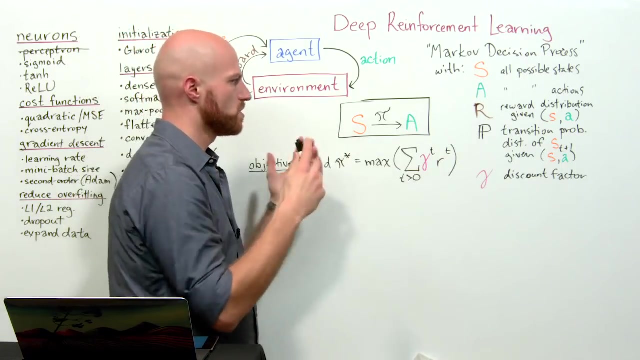 will be, the more discounted that reward is. So there's, given any set of states, our goal here is to create a, to identify a policy that maps our states to our actions. So, given some states, we want to have this overall policy of what we want to. 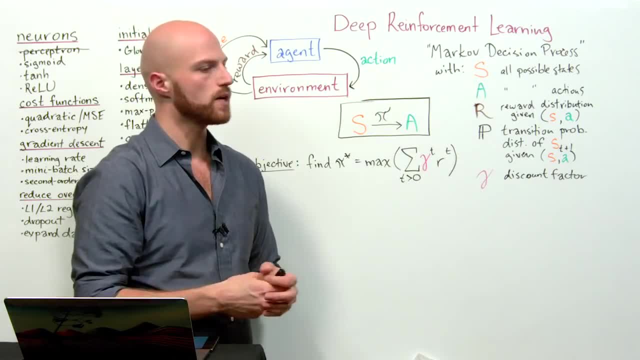 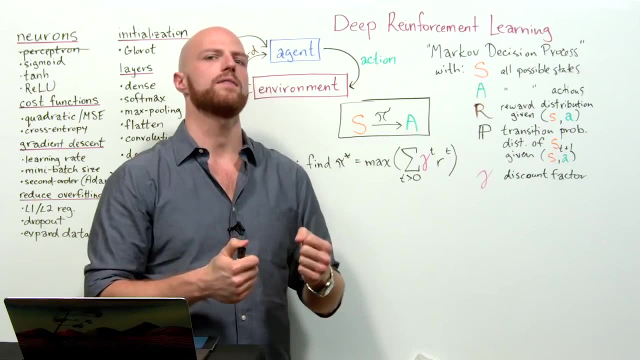 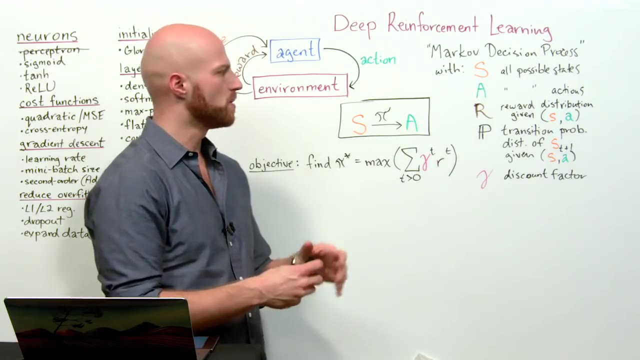 do, And then we want to know what kinds of actions we should be taking in those states. So it could be the case that in in some kind of states it's very clear exactly what kind of action we should take, And then in that case it's very it's relatively simple for the algorithm to identify a. 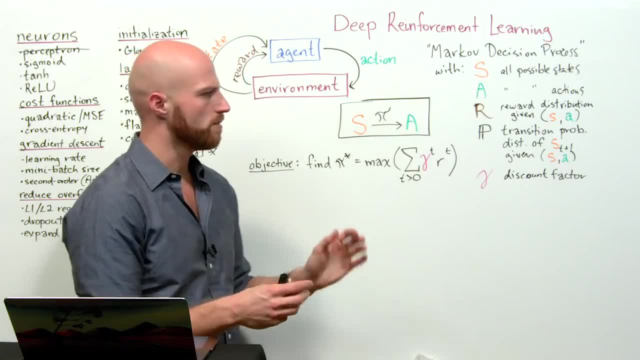 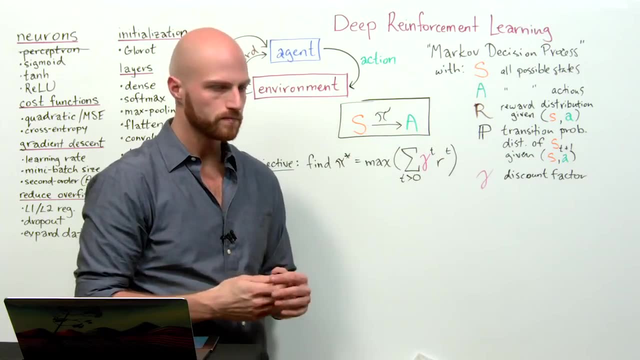 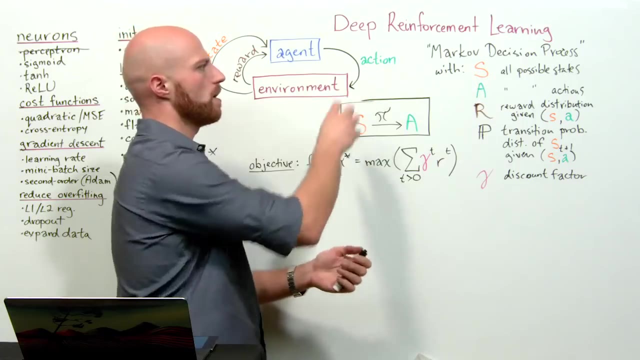 policy. But the more complex the game is, the more possible states that there are, the more uncertainty there is about what reward will be given in the future, the more complex this policy function is. So this policy function is the thing that we're trying to learn with our, with our deep reinforcement. 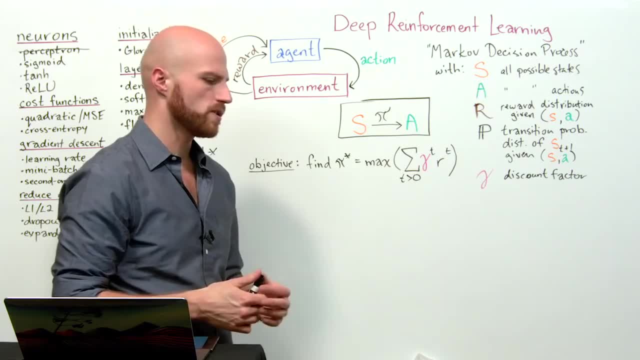 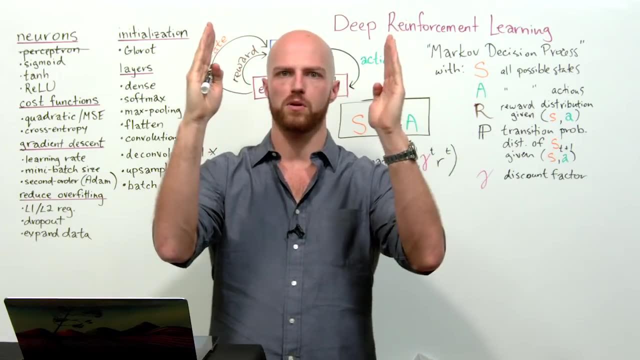 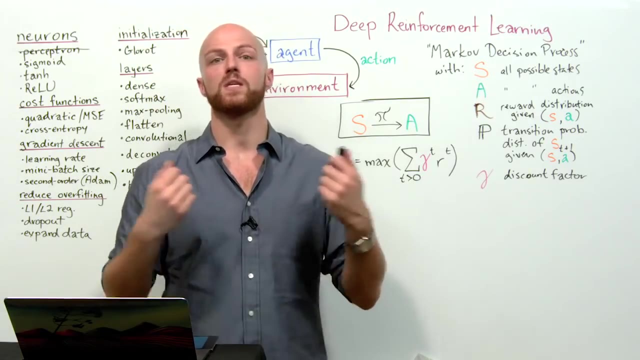 learning algorithm. You can imagine there's some kind of with this cart-pole game. if we're in a state where the pole is actually perfectly balanced on top of the cart, then the the policy in that particular situation is pretty easy to define the best policies to be used. 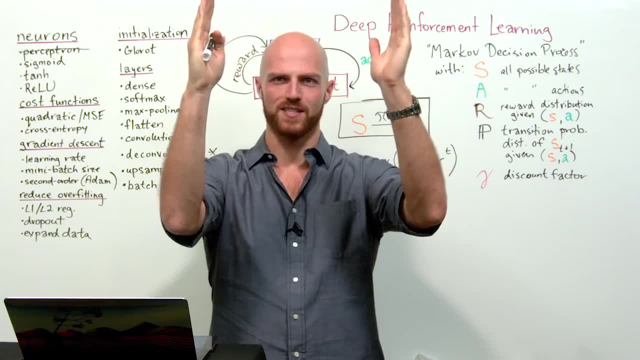 A to stand still. You know, the pole is balancing perfectly, so let's just stay in one place. We don't want to move to the right or to the left, But when the game starts, the pole is on some angle, and so 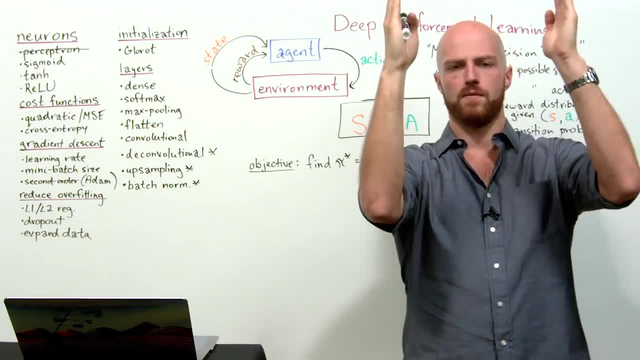 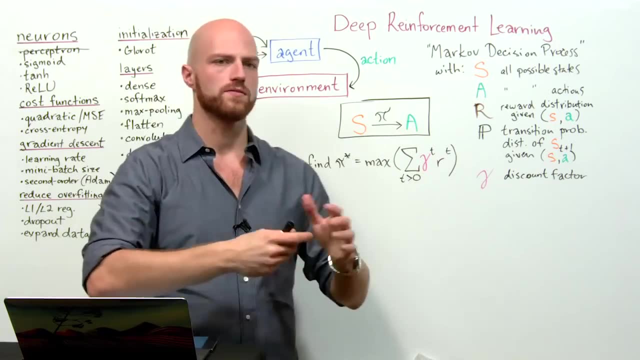 we need to figure out: okay, how many steps should I move to the left to get the pole to stay upright, to to keep us from dropping the pole? And so there's all these kinds of different kinds of states that we can have in the environment, all these different configurations of the cart with. 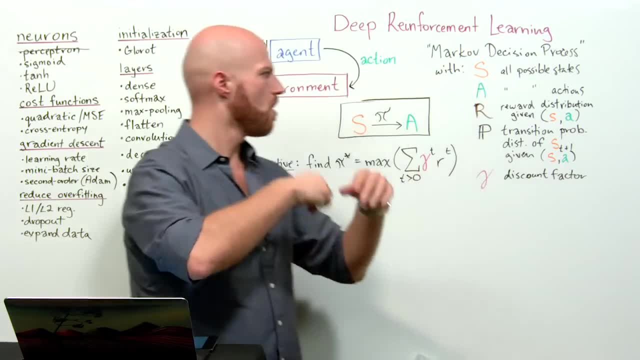 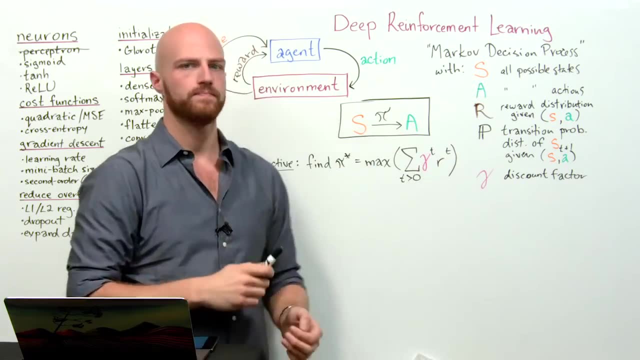 the pole on top of it and how quickly the cart's moving, how quickly the pole's moving, all of these, these various states. we need to come up with this overall, optimal policy of what action to take, And that's how we win the. 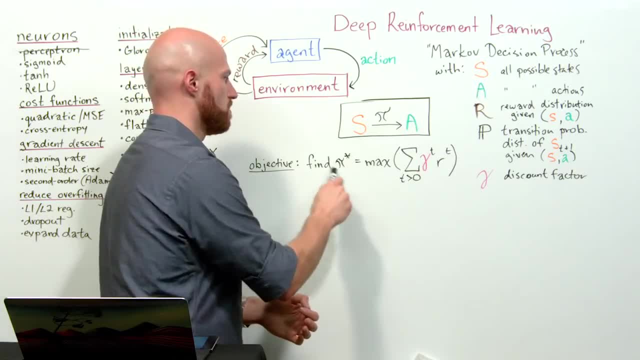 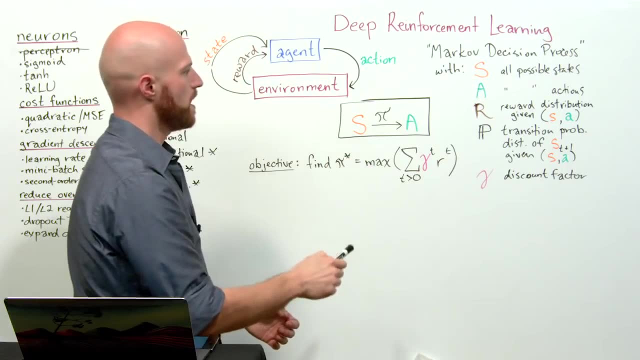 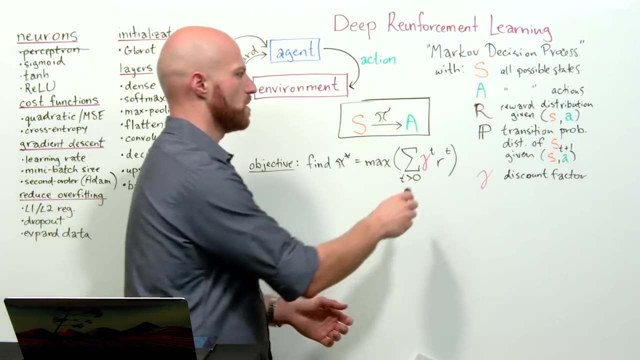 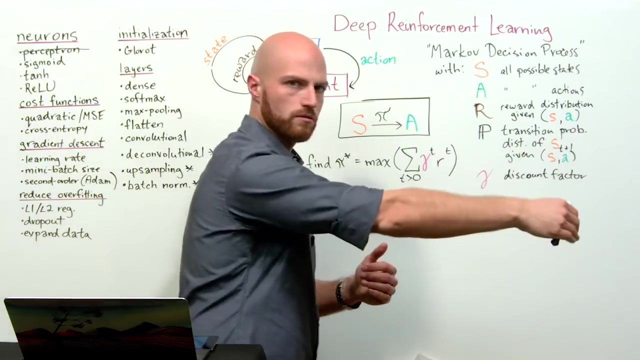 game. So our objective is to find the policy star, the optimal policy, And we can define this mathematically as the maximum expected cumulative reward. So you know, so we're trying to maximize our reward And we're discounting future rewards. So 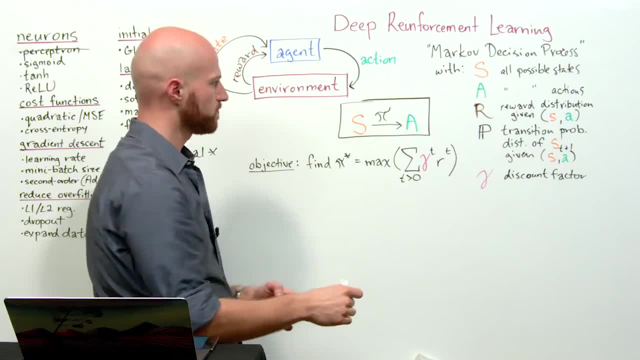 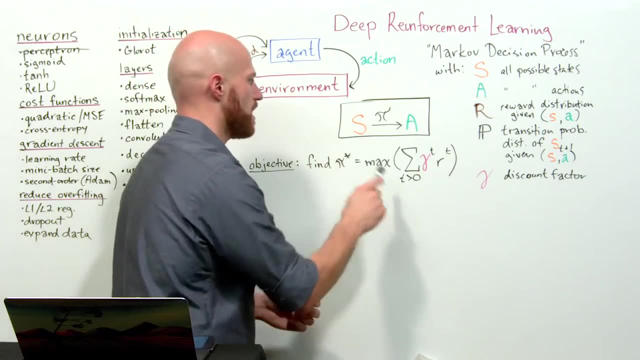 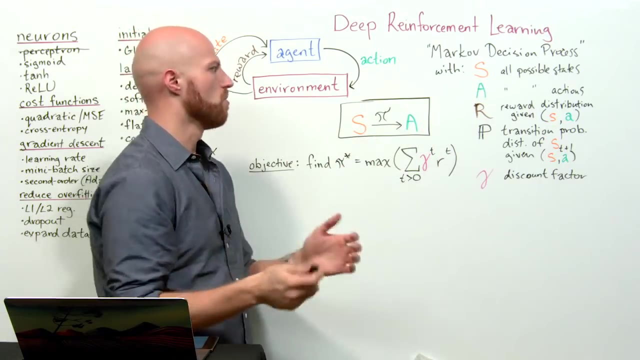 that's why we multiply our rewards by the discount factor And then we're just summing them together. So our policy, our optimal policy, here is to match, is to identify the, the perfect policy that guarantees that will maximize our reward given any particular state of the game. 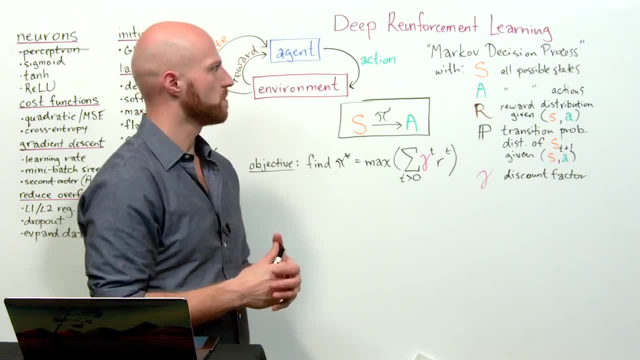 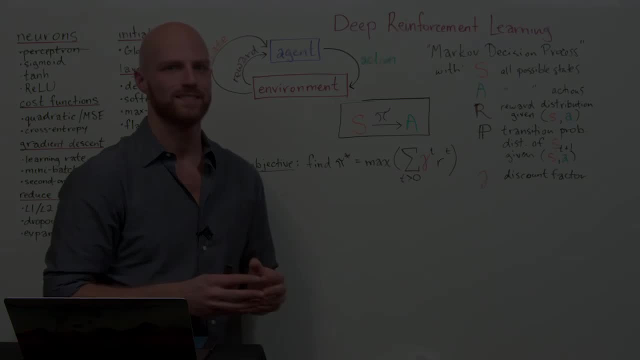 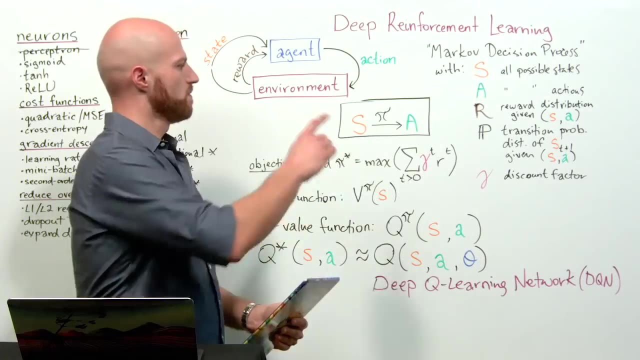 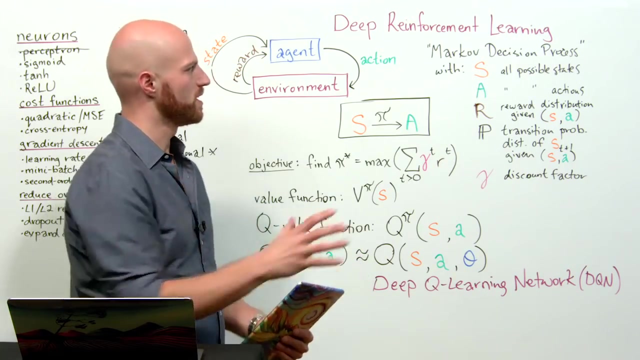 So that's overall what we're trying to do here. I'm going to throw a couple more equations at you next to define this a little bit further. So we defined up above here the general state of what's going on with reinforcement learning, the various terms that we need to be. 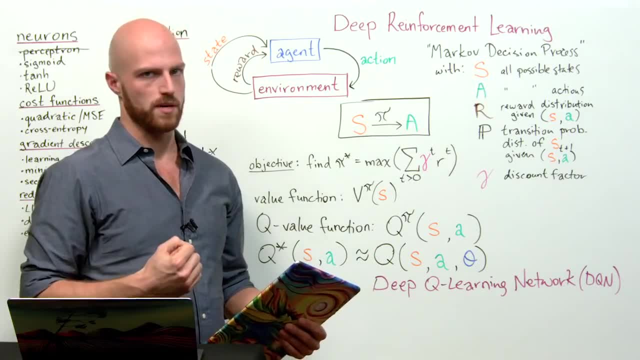 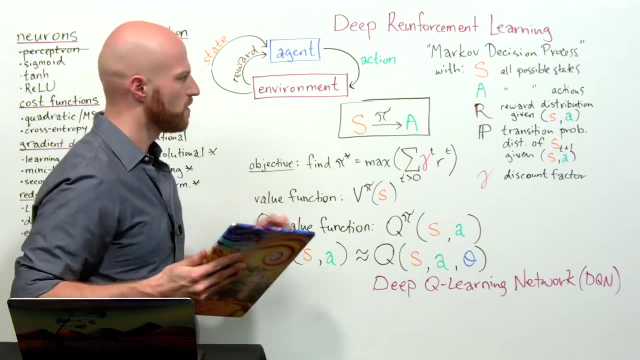 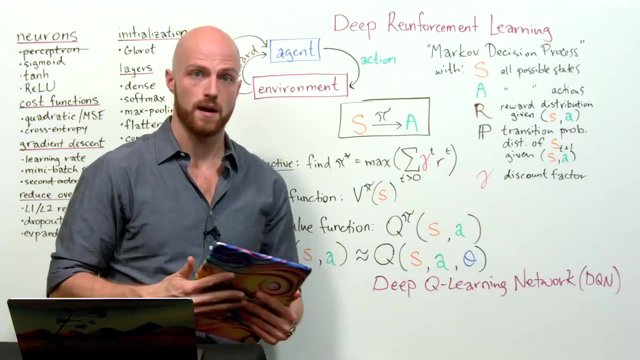 aware of as we start to build our deep reinforcement learning algorithm coming up next momentarily. just need to spend a few more moments here talking about a few terms related to the specific type of deep reinforcement learning algorithm that we're going to build in these live lessons. So let's talk about a few more. 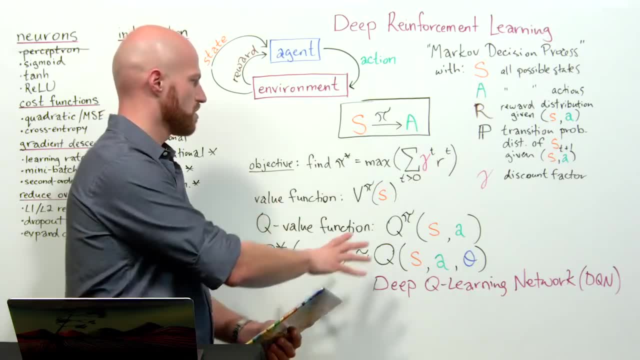 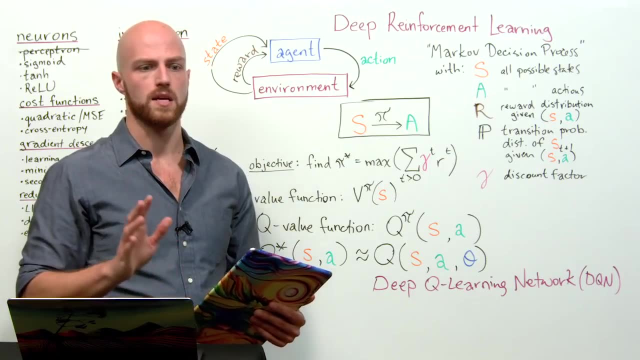 key terms at a high level. These are going to be these terms down here: the value function, Q value function, this kind of thing. We don't have time to go into the mathematics in incredible detail here. If you'd like to do that- and I encourage you to do it- I'd 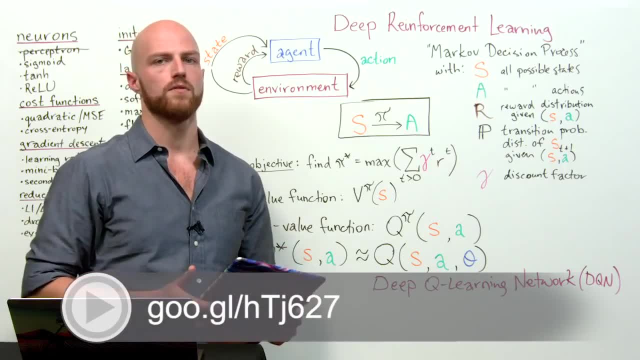 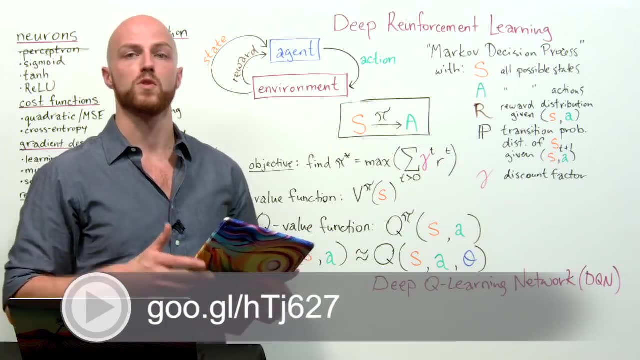 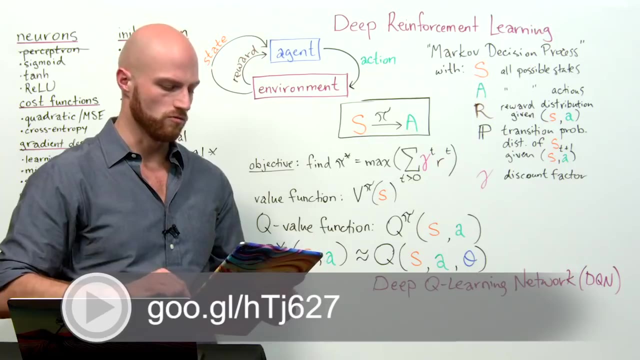 recommend you to check out lecture 14 from Stanford CS231N- their summer 2017 iteration of that. The class was given by Serena Young and she used the same kinds of terminologies I use here. So if you want to dive deep into the mathematics, that is a great way to do it. So we're 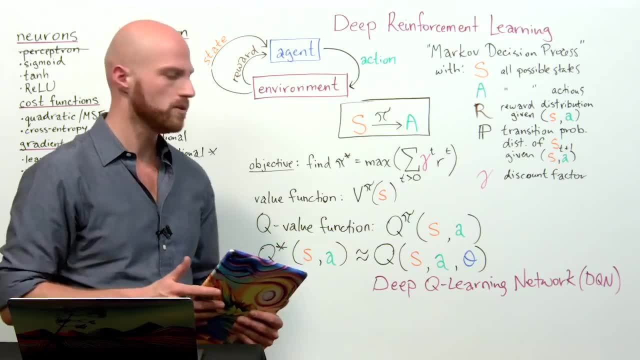 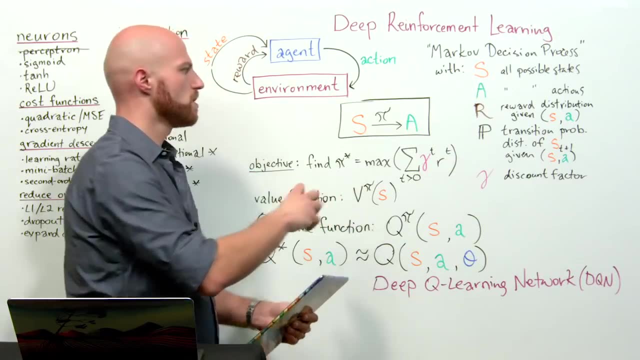 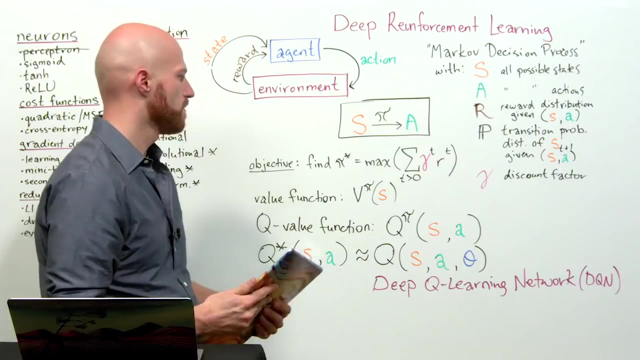 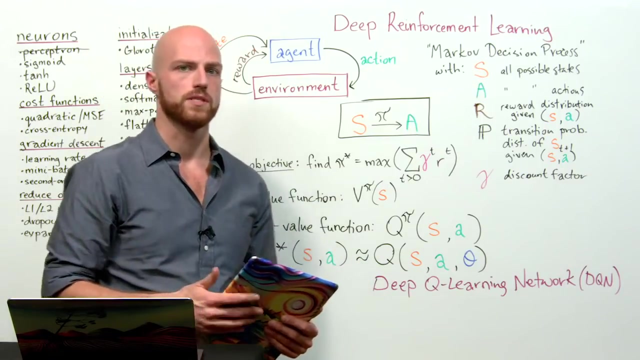 just going to talk about these concepts at a really high level. The value function is the expected cumulative reward. So what's the expected reward that you can get from being in a particular state of the environment? So in this carpool game, for example, if we are in a state where the 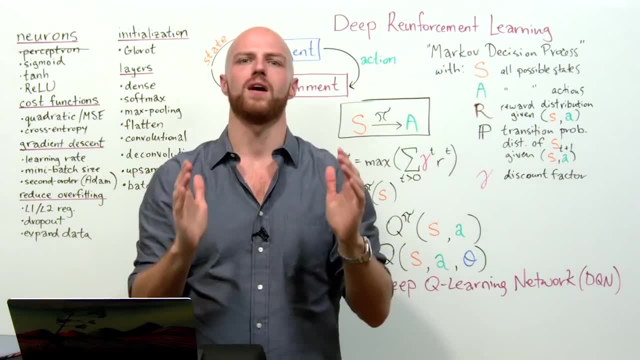 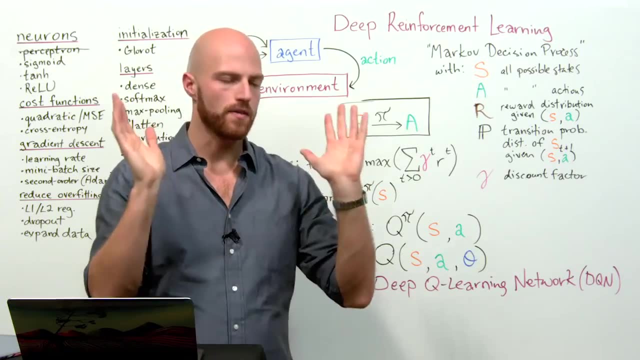 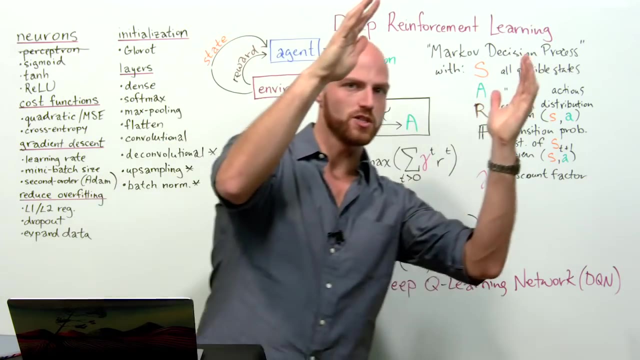 pole is nicely balanced on top of the middle of the cart, then our expected reward in that situation is pretty high. On the other hand, if we're in a situation where the pole is on a large angle and we're quickly chasing after it- that's the current state of the game. 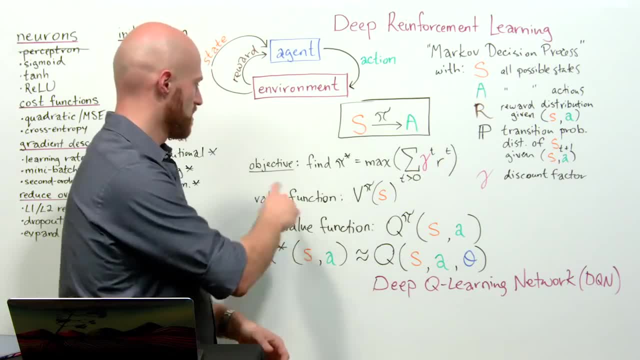 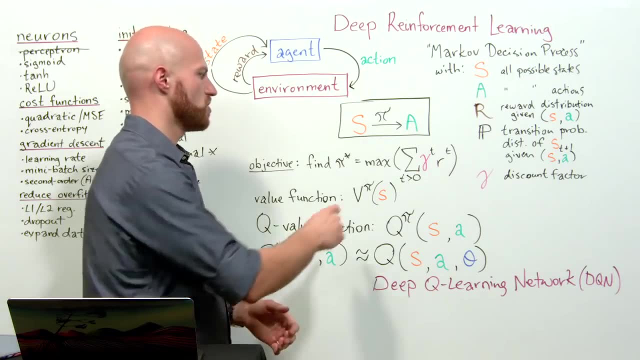 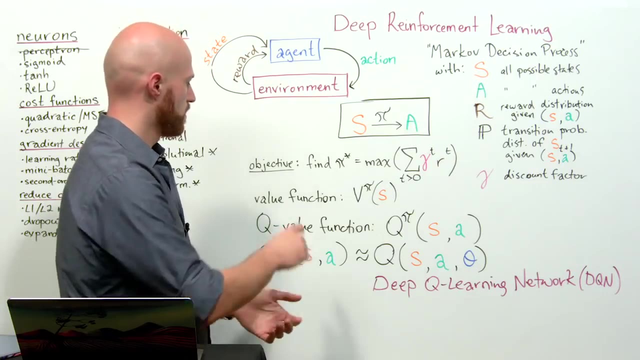 Well then, our expected reward in that situation is smaller. So that's where the value function comes in here. So with a value function, we're just taking into consideration our state and the pole of the seas, pi, that we take in that state. 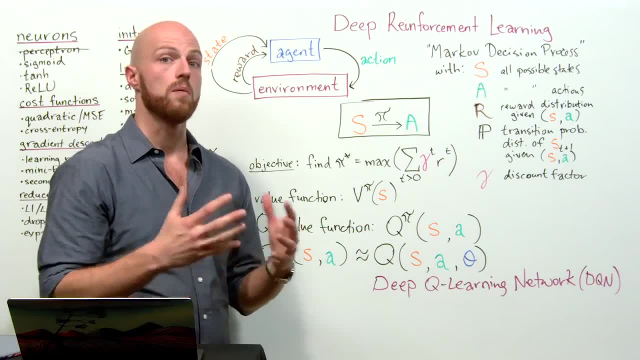 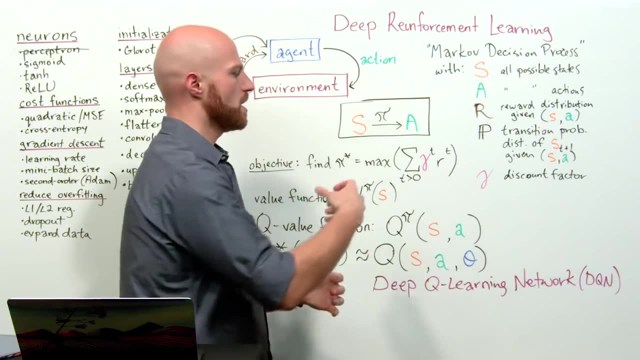 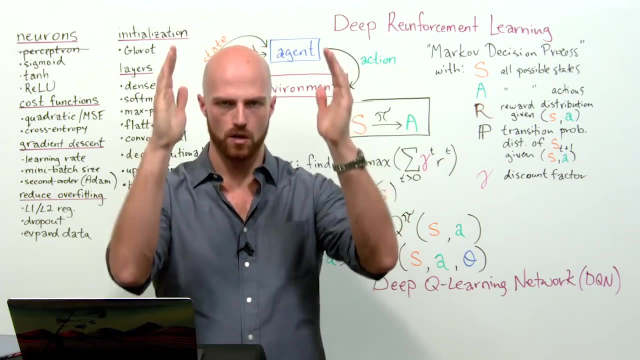 The Q value function is one step more complex because with the Q value function we consider both our state as well as a given action. So you know, same kind of thing in the carpool game. you know we have our state where we're centered there. 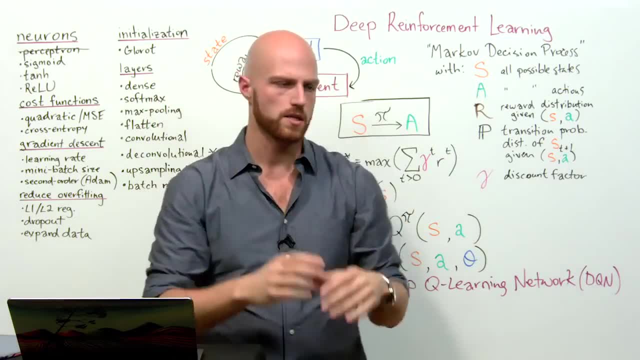 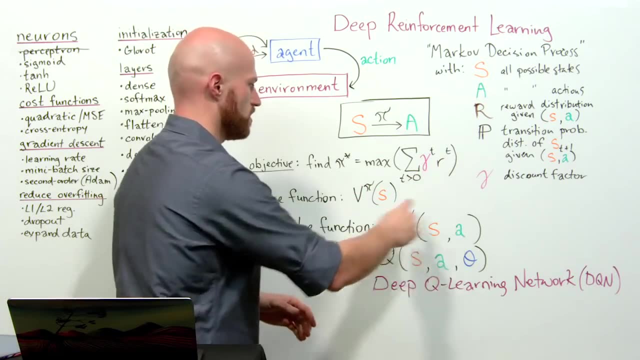 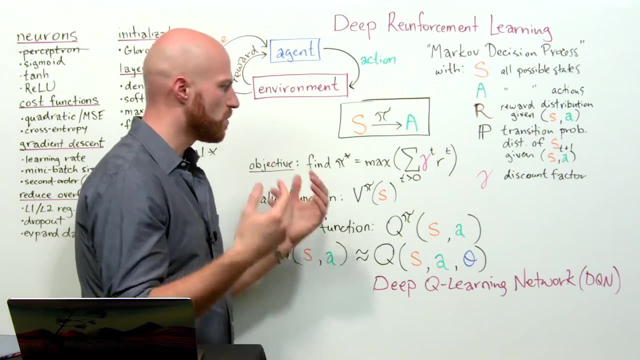 the cart is steady and the pole is well balanced. Well then, there's, you know, an action left or an action right that we can take, And the Q value function tells us what our maximum expected reward we can get from the situation of being in that particular state. 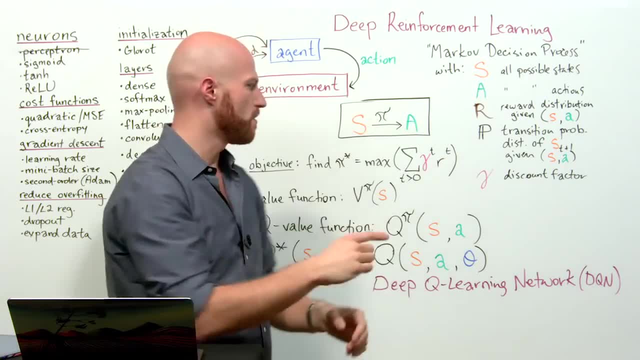 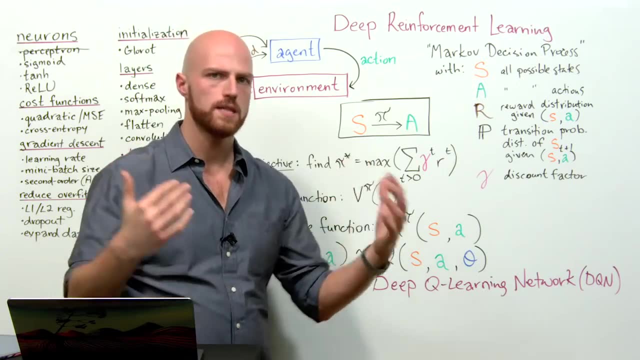 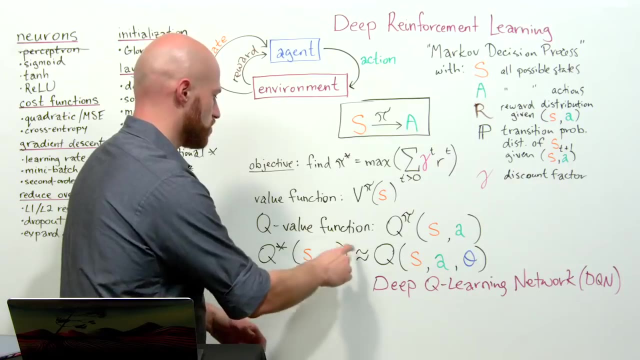 taking a particular action, so taking the left or taking the right, and then following our policy afterward. So the Q value function is the maximum reward in that particular state, given a particular action and then following our policy. The Q star, then, is the optimal policy. 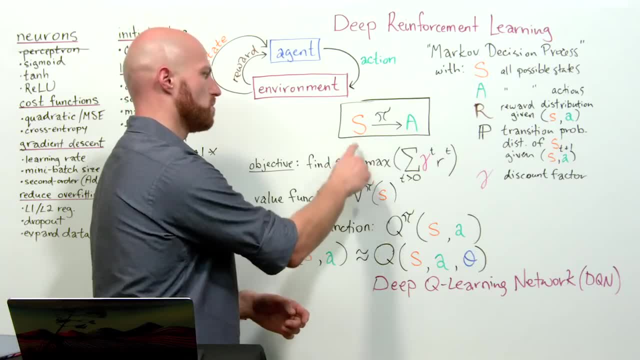 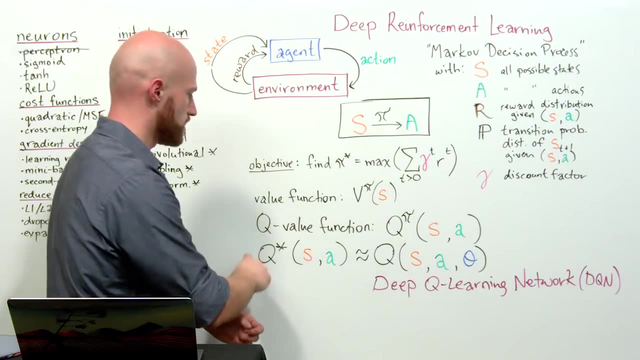 sorry, the optimal Q value function. So we have the optimal policy up here, recommended by denoted by the star, the asterisk, And so it's the same kind of idea. here We use the asterisk to denote the optimal Q value policy. 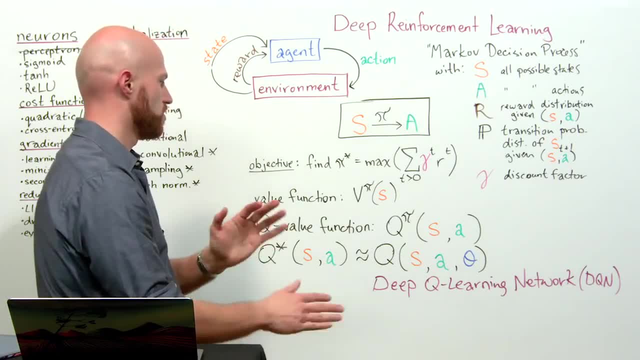 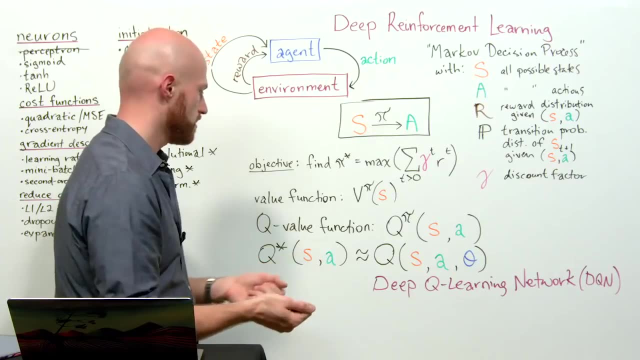 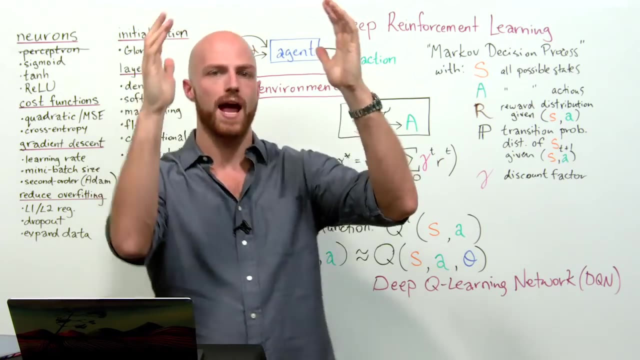 given a particular state and a particular action. So this is the optimal, the most optimal, the most optimal, the most expected reward that we could get, given the particular state that we're in. so the particular cart and pole configuration and the particular action. 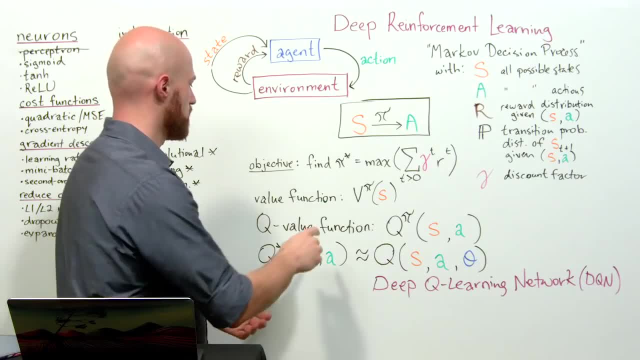 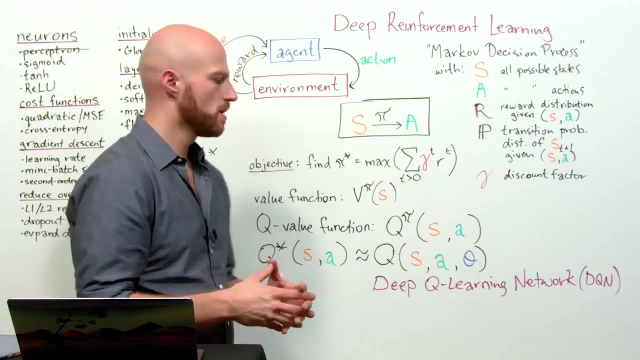 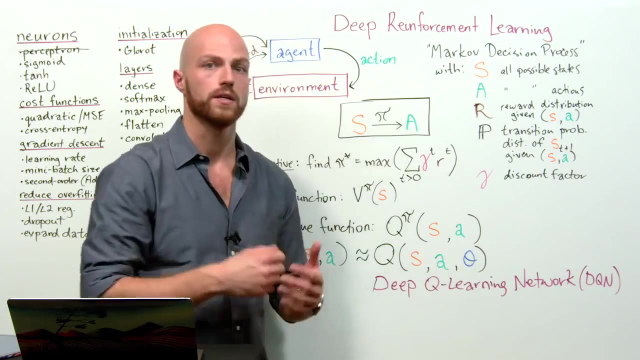 And then following the policy from that point onward, this is the optimal. this is the Q star. Well, what we're going to do to approximate Q star is to use something called a deep Q learning network, DQN. So that's the particular type. 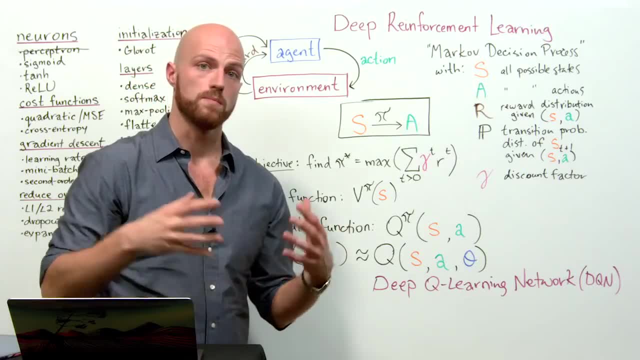 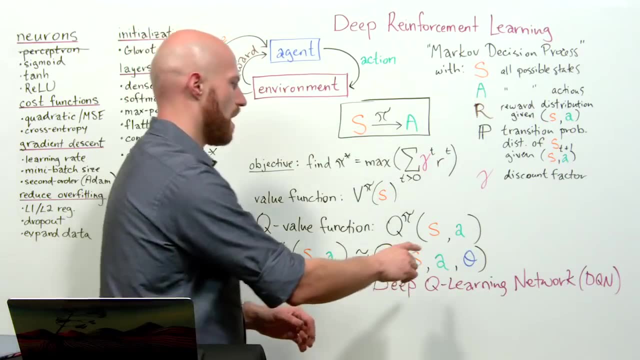 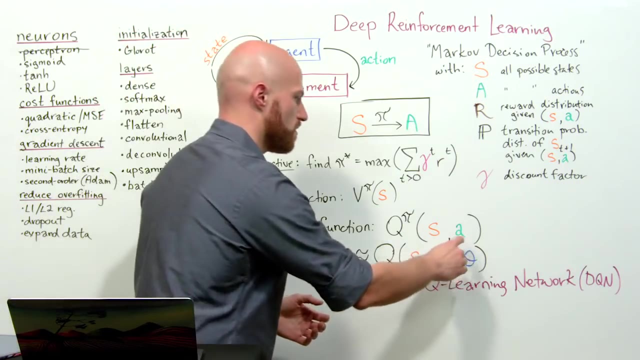 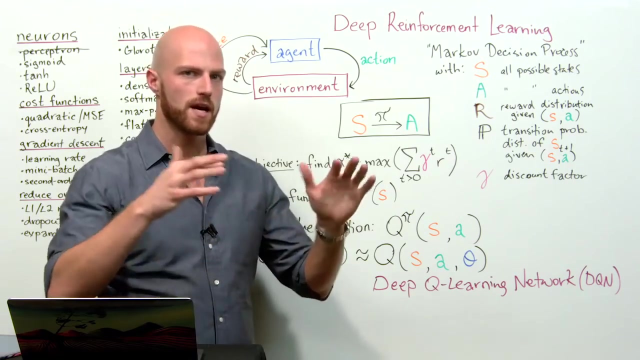 of deep reinforcement learning agent that we're going to build in these live lessons, And so to define that, we can simply add one more term to our Q function here, And so this is theta, and theta represents all of the weights in this kind of function that we're using to approximate. 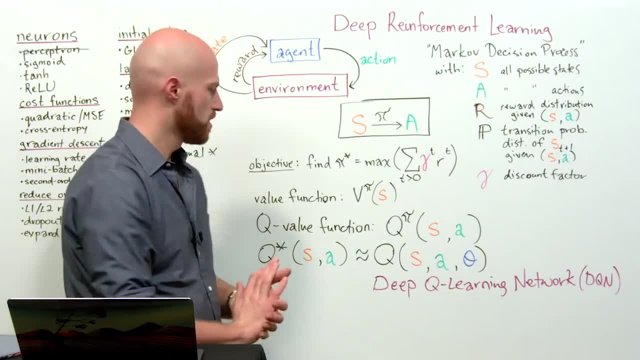 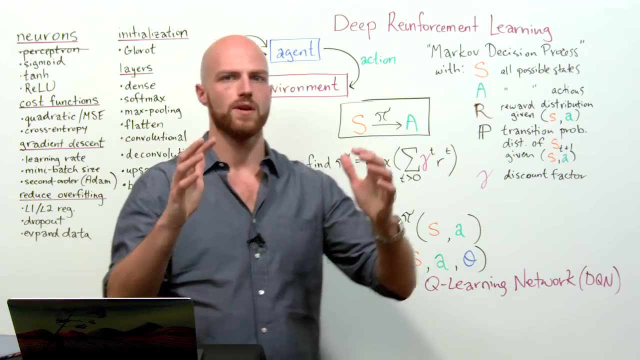 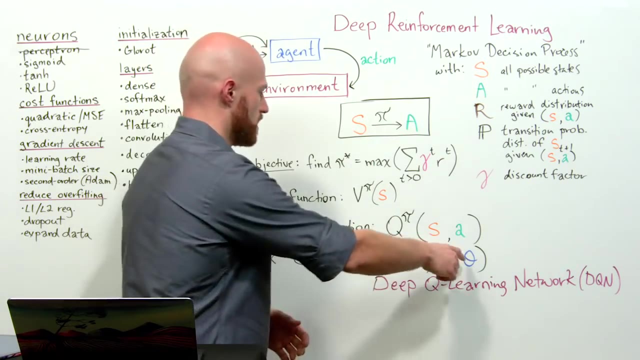 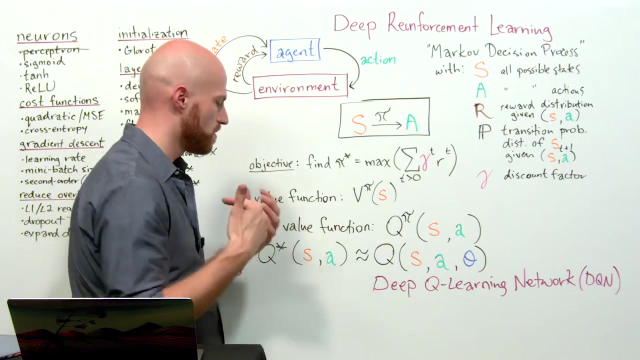 approximate the optimal Q. So we have a given Q. so with a particular state and a particular action, and then this particular set of weights, we can estimate what the maximum expected reward could be, what the you know the best that we can do. 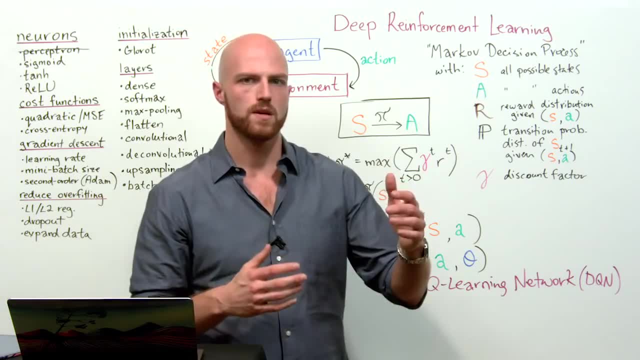 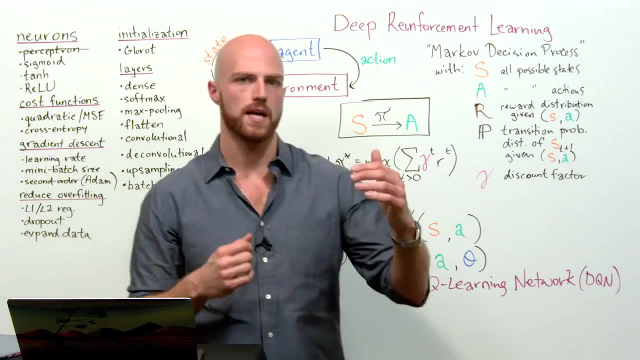 And so that enables us to figure out: okay, well, if there's these we can, we can test the various possible situations. So we can say: okay, so I'm in this state If I take this action left or I take this action right. 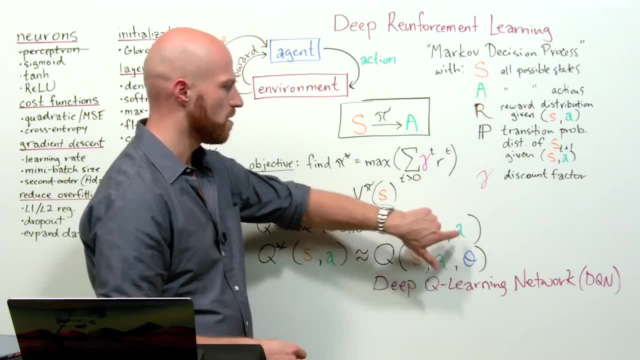 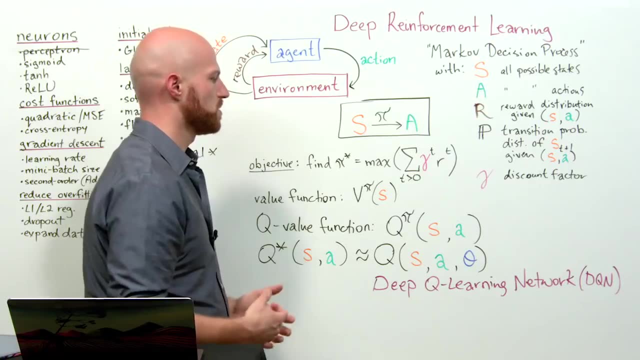 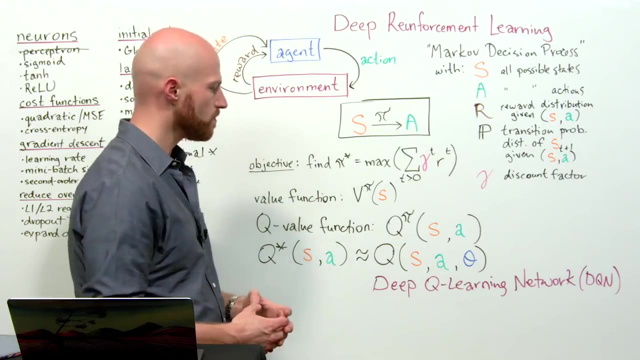 and then I have this way of approximating with all, with all of my weights, the maximum expected reward that I could get. this enables us to take the action that will give us the maximum expected reward, So this theta could actually be any kind of function. 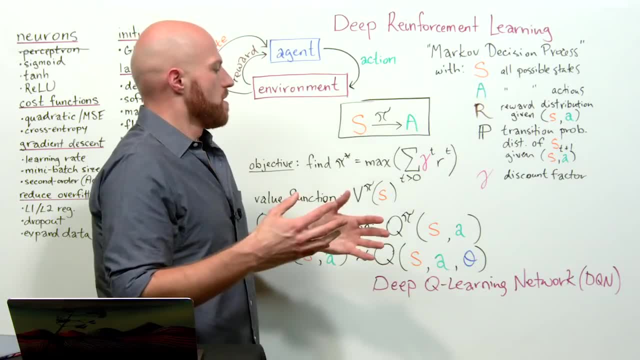 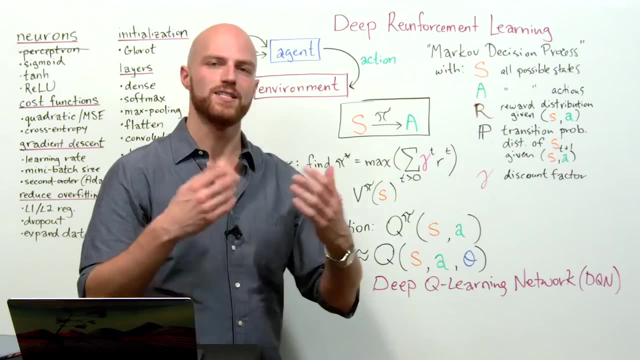 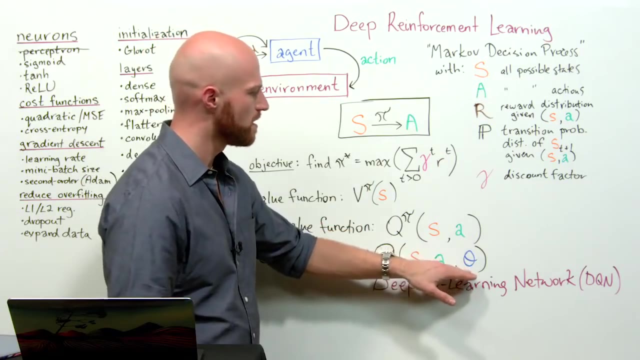 It could be a linear regression model or something. The thing that makes this a deep Q learning network is that this theta is a deep neural network. So you build some kind of architecture with TensorFlow or Keras to have a set of weights and biases. 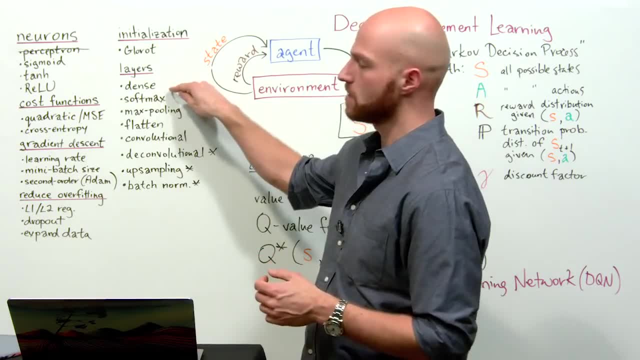 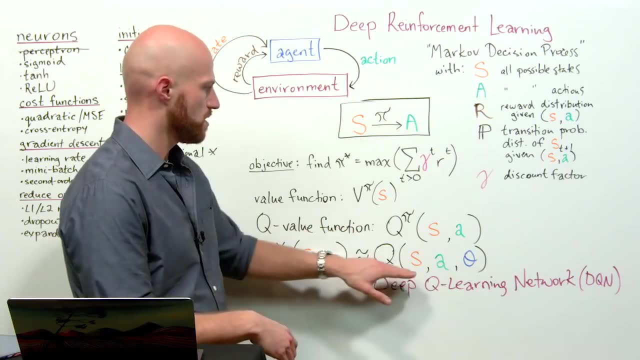 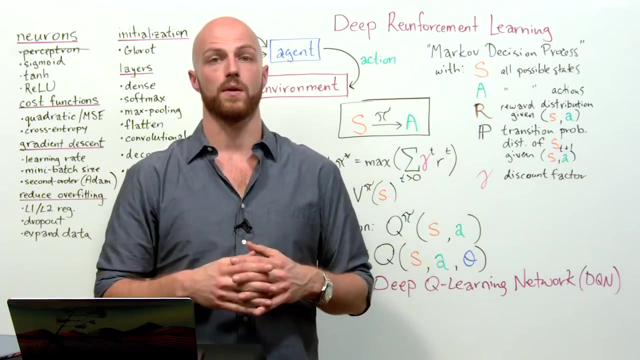 In our case, in the deep Q learning network that we're going to build, we're going to use simple dense layers to approximate this equation here. So our theta is going to consist of the weights and biases in our dense layers of this neural network. 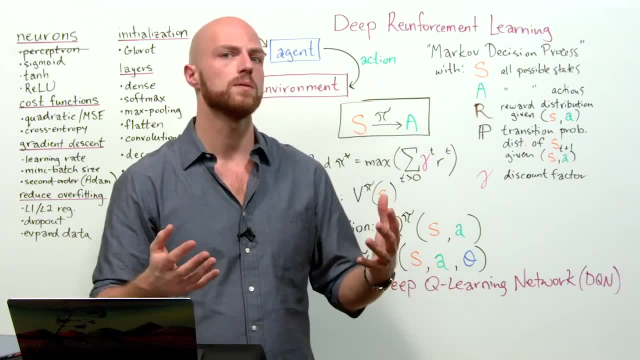 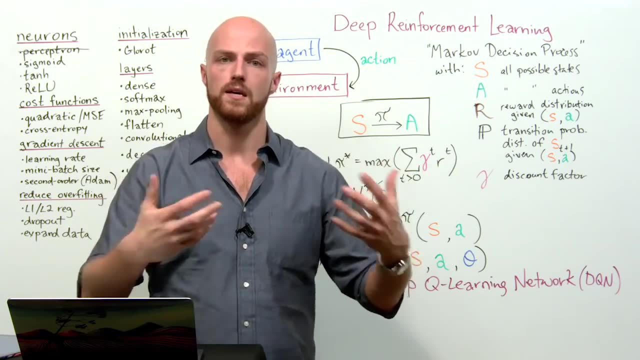 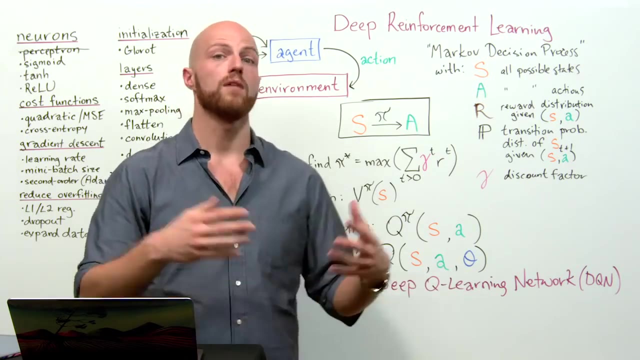 that we're going to build. If the situation was some kind of other problem- so let's say that we were using the whole screen of an Atari video game as the state- then we would have some more kind of complex deep neural network like a convolutional neural network. 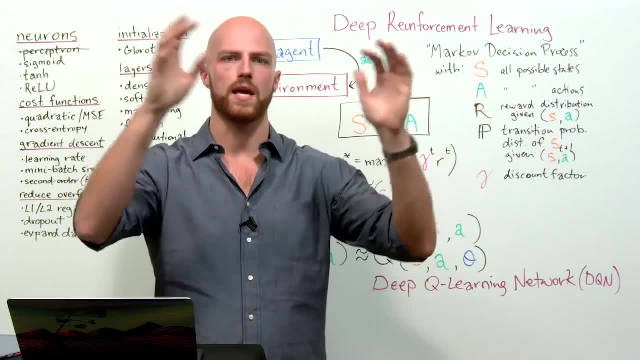 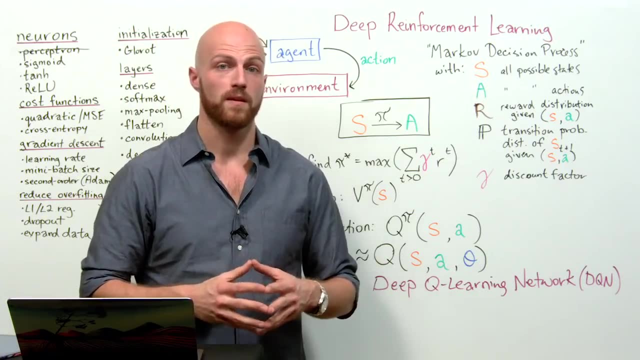 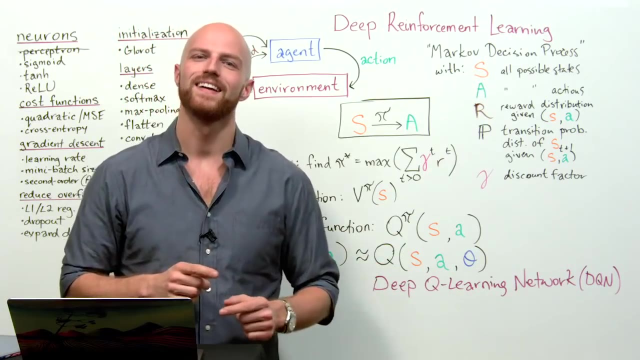 for identifying features in that whole game screen that enable us to take the best course of action. So that's the idea here. This is a high level overview of all the theory. We're going to reinforce these terms as we start building our code. 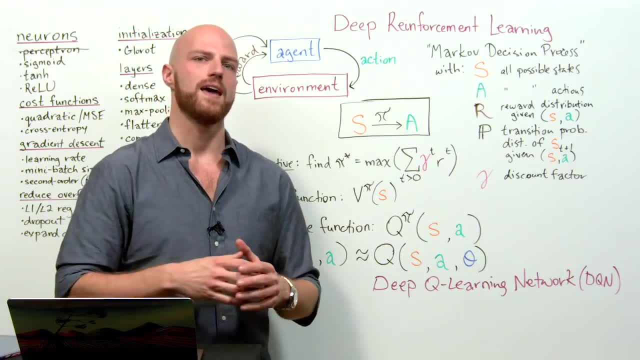 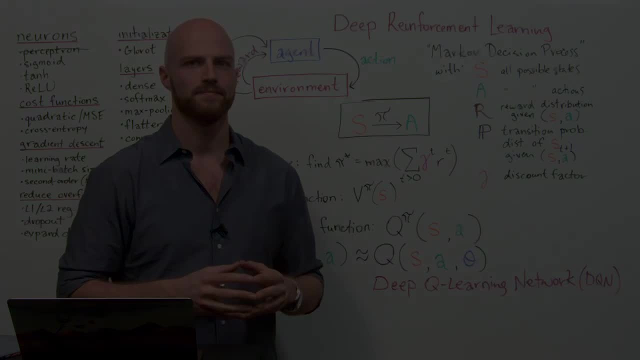 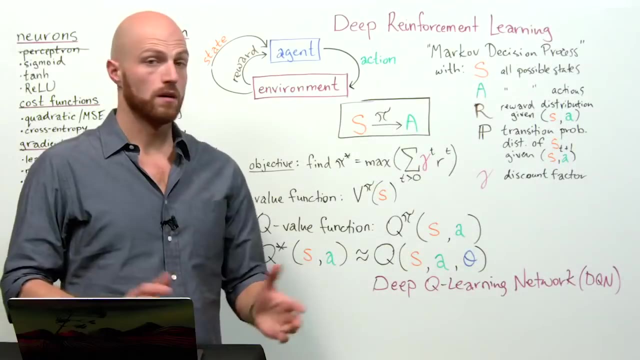 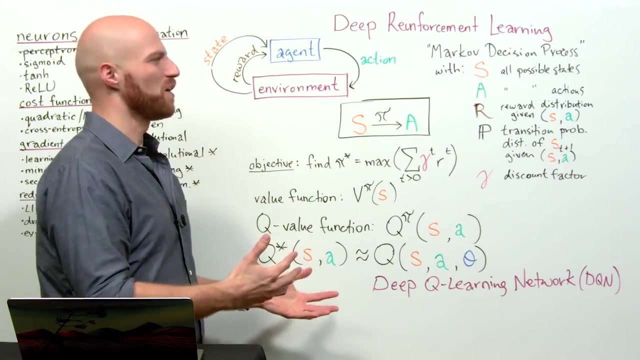 We're going to talk about many of these terms again, And so bear with me. Everything will start to fall into place as we go. What an exciting time in these live lessons We've gotten through the drudgery of all of our deep reinforcement learning theory. 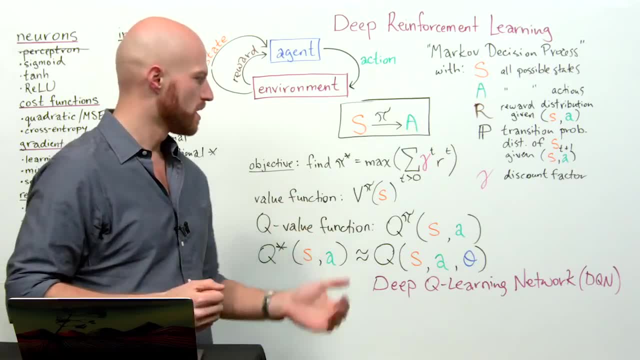 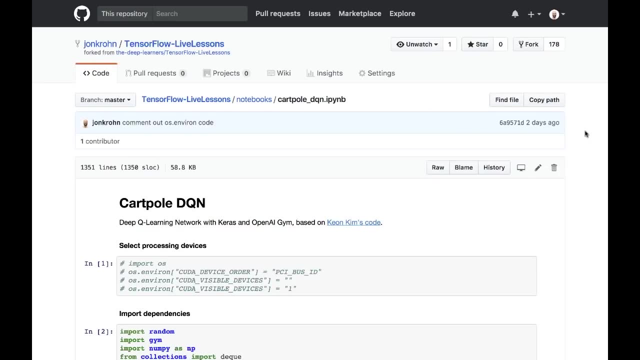 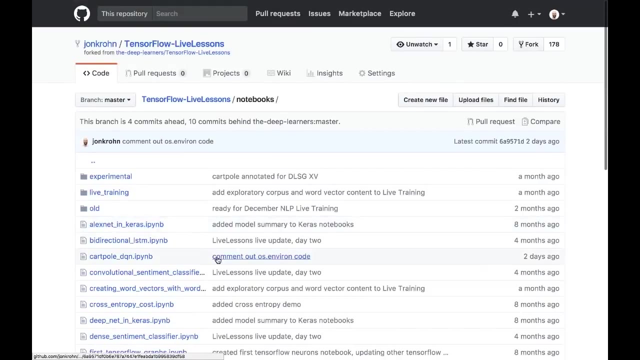 and now we actually get to put it to use in code and build our own deep Q learning network for winning the carpal game. So the completed notebook is available for you, of course, in the notebooks directory. for you to follow along, It's the carpal DQN network. 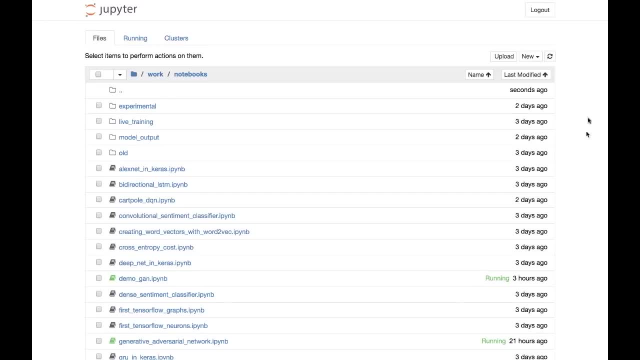 I am going to be rebuilding that for you guys here so that we can talk about it line by line. make sure I don't go too fast over anything And I encourage you to follow and do the same thing. It'll help reinforce what we're doing here. 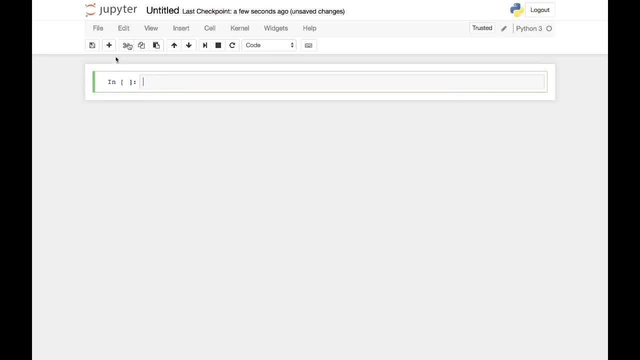 So I've got a new Jupyter notebook open. I'm going to give it some kind of name like demo DQN. I'm going to add a title. It's going to be a carpal DQN. So the code in this notebook for this deep Q learner. 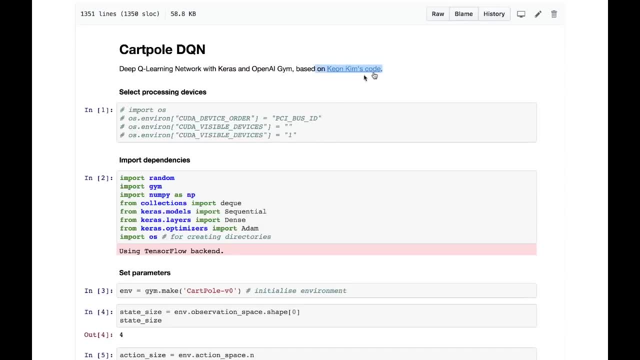 is based on code by Keon Kim, who is a student at NYU. You can check out his implementation by clicking through that link. There is a first step that I've put again at the top of the notebook here, just like for our generative, adversarial network. 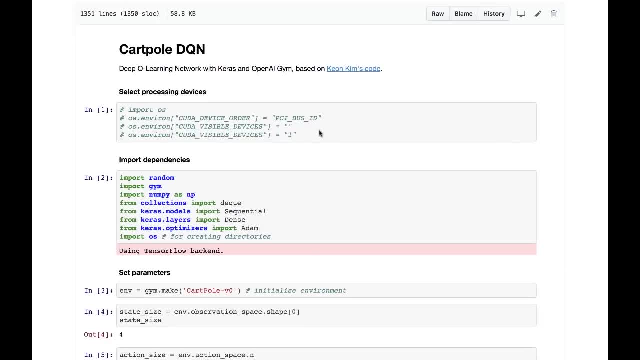 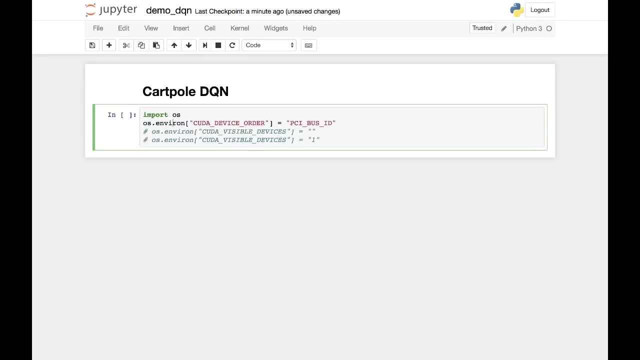 If you're using a machine with multiple GPUs, then you can use this code in the same way that we used it in our generative adversarial network to decide on which devices you want to be running this on. So in our case here, I actually just want to run it on my CPUs. 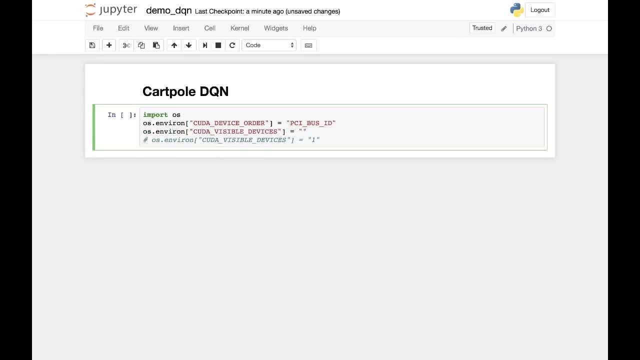 So I'm going to leave this blank here, And this means I won't use any CUDA devices, which means I won't use any GPUs. I want to take a moment to reiterate that this cell here is only useful if you have NVIDIA GPUs on the machine. 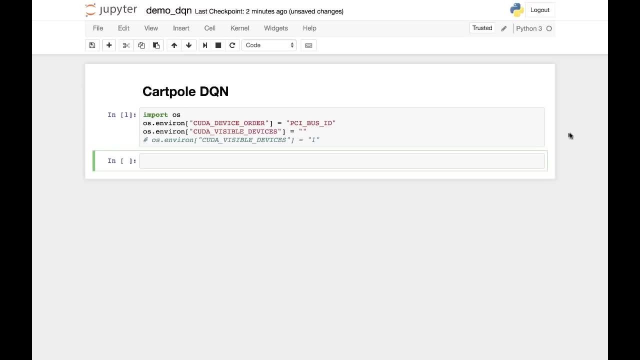 that you're doing this work on. Otherwise, you can ignore the cell completely. All right, the first step for everyone is to import dependencies. So we're going to need something called a random. We're going to use the OpenAI GIM. 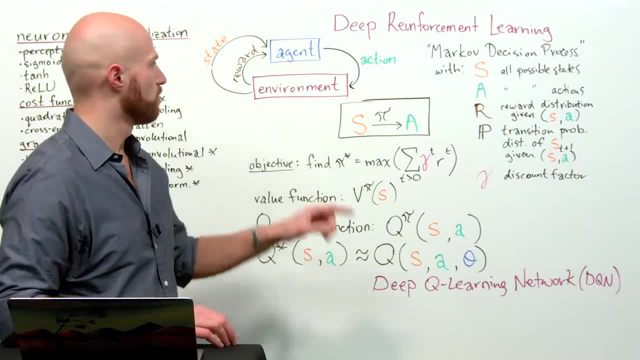 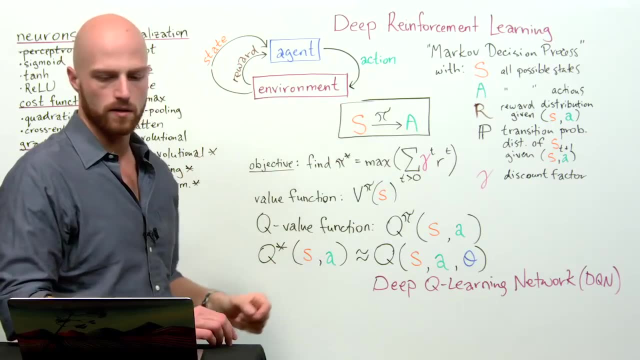 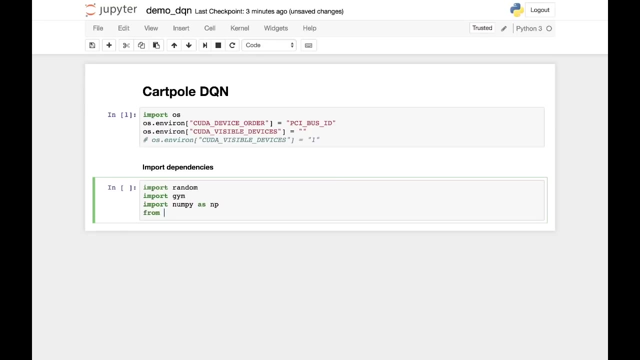 which I showed you guys earlier in these live lessons, to render our environment for the agent to take actions in and receive feedback from. We're going to use NumPy, We're going to use a special kind of list at one point for the memory of our agent. 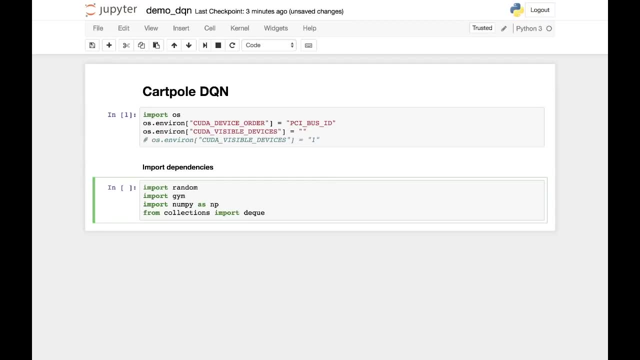 We'll talk about memory more later on. We're going to use something called a DEC, which is just like a list, except you can add things to the front or the end of the list, And then we get into our Keras stuff. 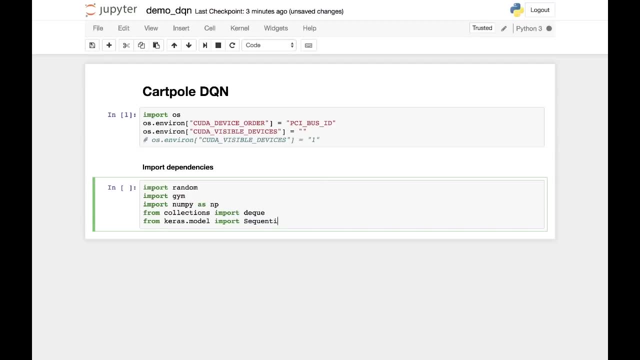 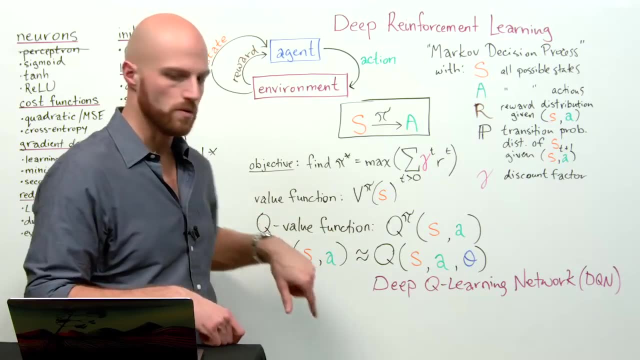 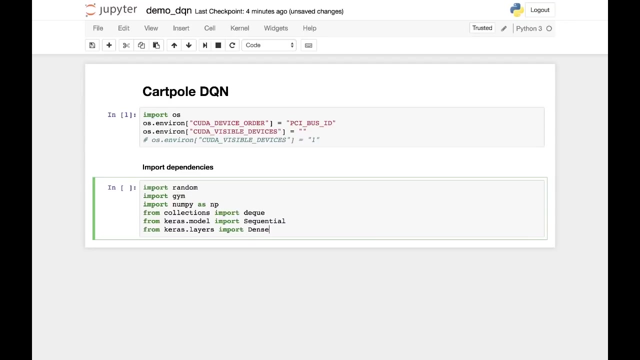 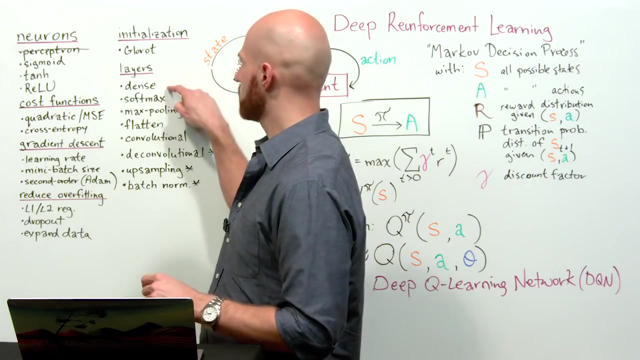 So we're going to use a sequential model to build our neural network for approximating the optimal behavior of our agent, And then we're going to use a Q. here We are only going to use dense layers in our network, So the theta weights. 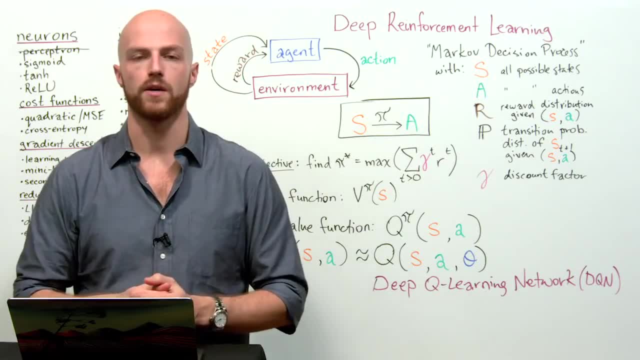 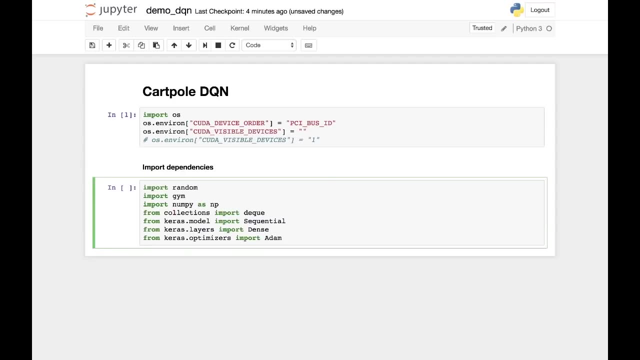 will simply be the weights and biases of neurons in between layers of a dense network. We are going to use our trusty old model. We're also going to import OS for creating directories later on, if you didn't happen to do that already in the cell up here. 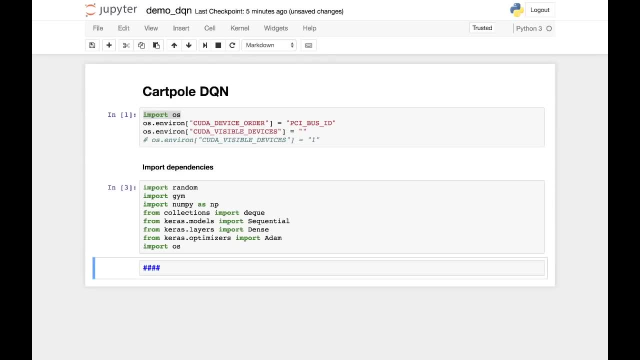 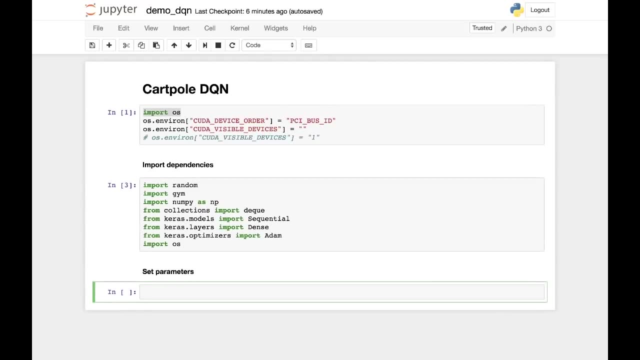 Keras models, not model. Let's set some parameters at the top of this file, So it's ideal to have as many hyperparameters as we can at the top of the file. I'm not going to be super religious about that rule this time around. 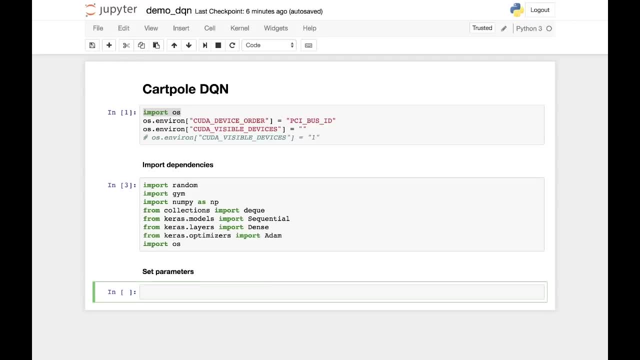 but we are going to define some of our key parameters at the top here. So one of the first things is to define exactly what environment our deep reinforcement learning agent is going to be in And, as we've discussed, this is going to be the Card Bowl game. 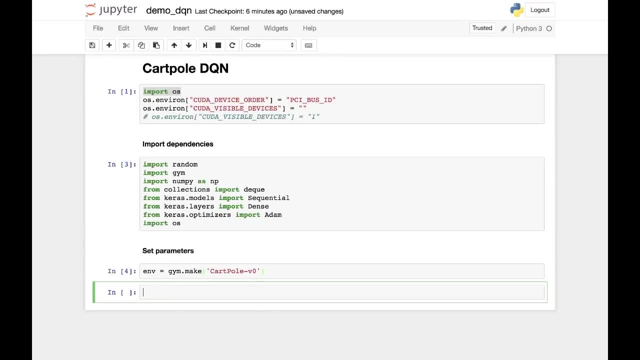 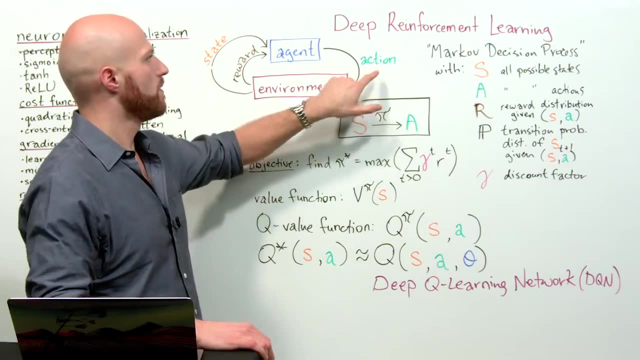 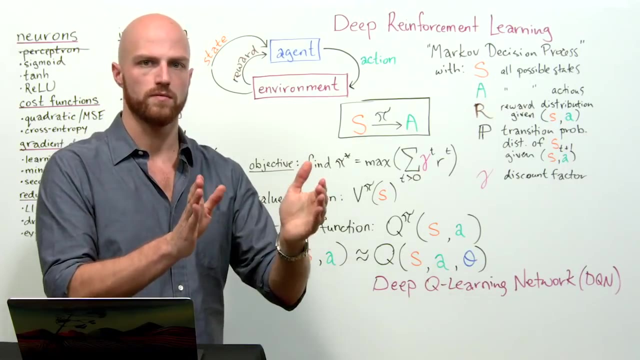 Version 0.. So that initializes our environment. There are some hyperparameters related to the size of our state and the size of our actions. So we have four possible states in the Card Bowl game: The location of the cart, the velocity of the cart. 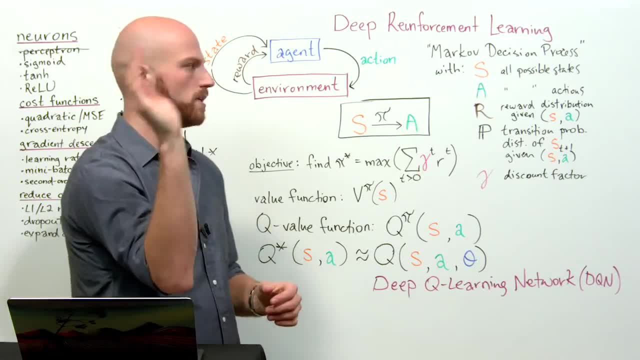 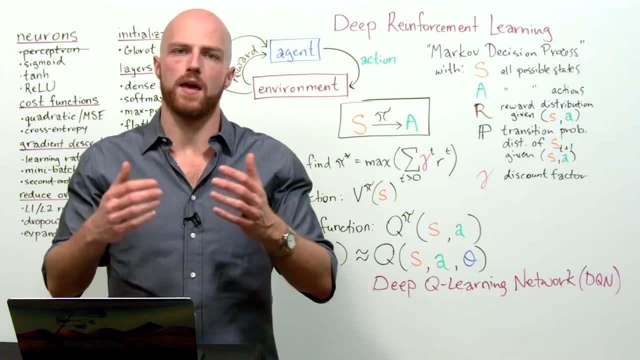 the angle of the pole and the angular velocity of the pole on top of the cart. And then we have two actions. So we're just going to create a couple variables here, because we're going to use those numbers a lot, And by doing it this way, 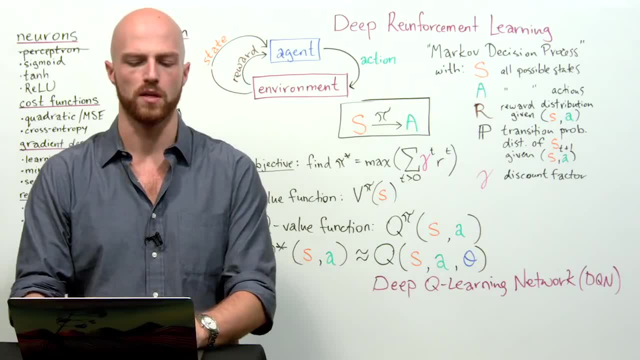 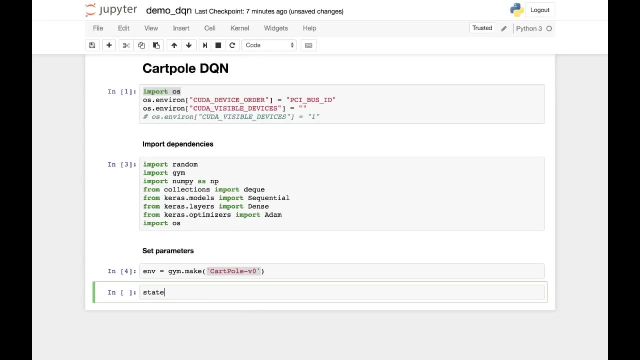 instead of hard coding in 4 and 2, it makes this code a bit more flexible If you want to switch to a different kind of environment in your own time. So let's define the state size variable. So it's simply here we go. you can see four. 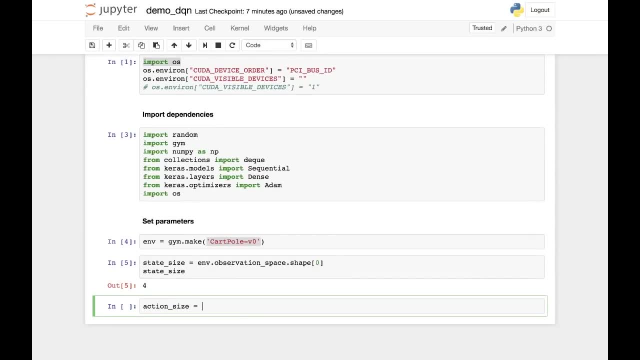 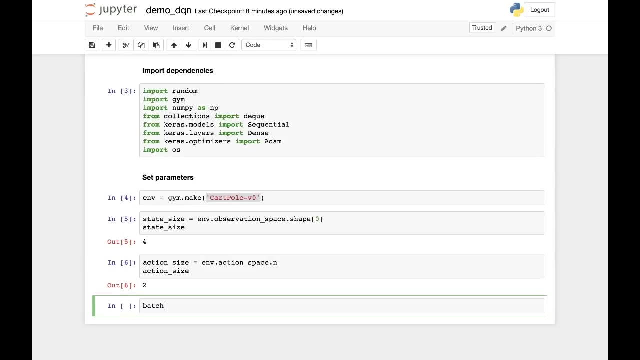 four possible states, like I just said, And action size is going to end up being 2, as I will show. So we are going to define a batch size for our gradient descent. We're going to set that to 32.. It's a hyperparameter that you can vary by powers of 2. 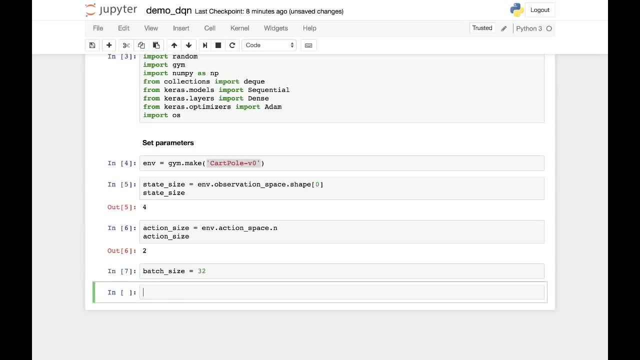 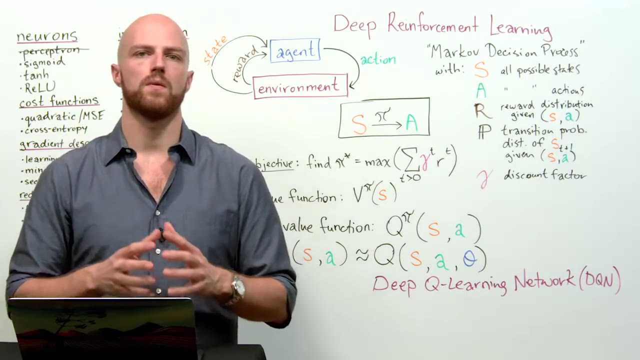 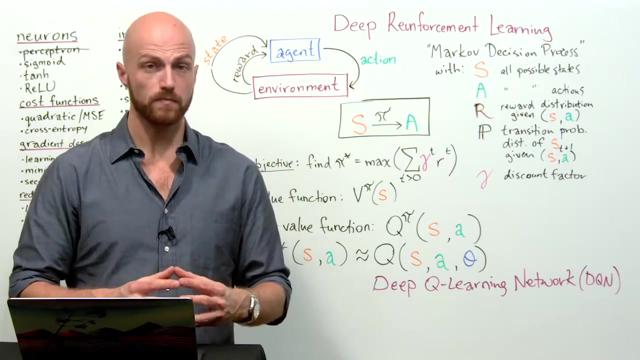 if you want to, It shouldn't make too much of a difference on the outcomes. And then the number of episodes is the number of games that we want our agent to play. So you'll see, as we get into the code form, the number of games that we play. 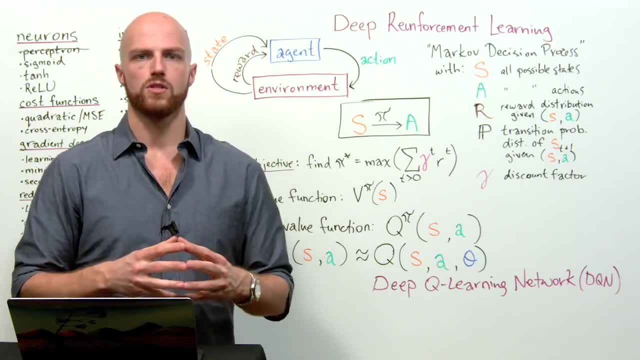 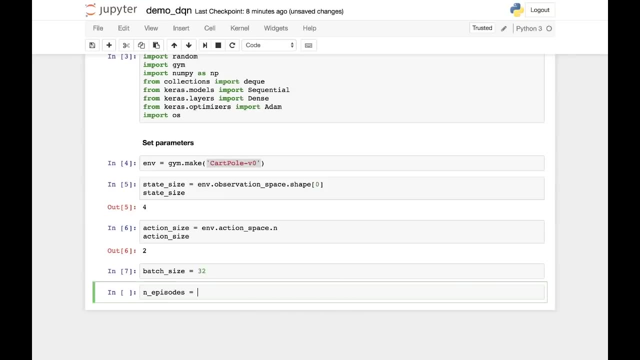 provides us with more data for training. So what we're going to do is we're going to play a number of episodes. Let's say we're going to play a thousand and one episodes. Let's say we're going to play a thousand and one episodes here. 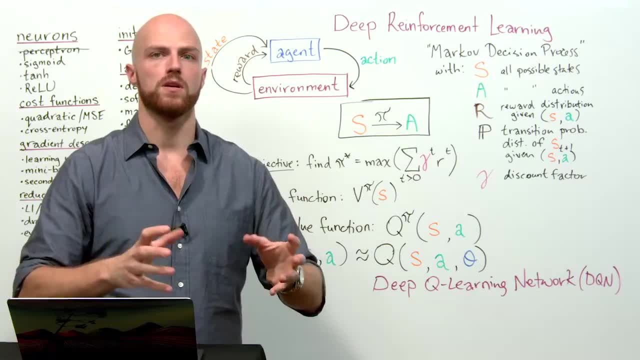 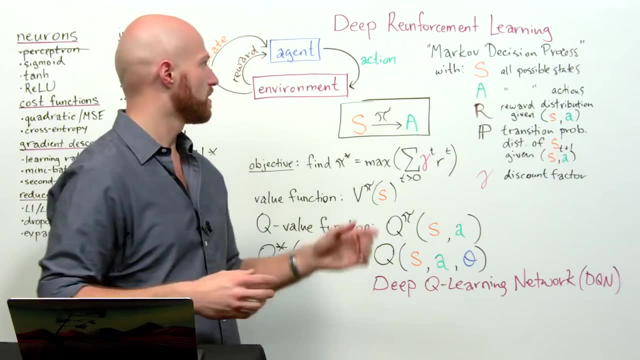 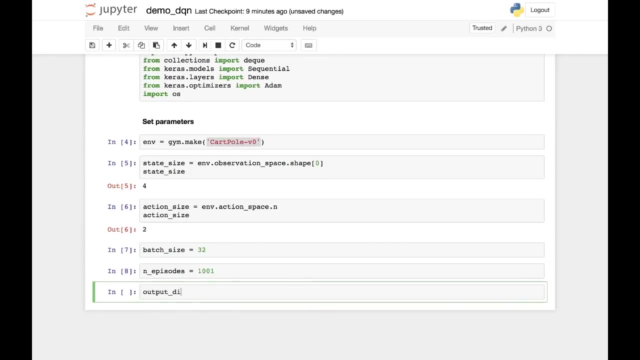 In each of those episodes we are going to randomly remember some of the things that happened in that episode And we're going to use that memory to actually train our deep reinforcement learning agent. So we'll see those step by step as we go through. 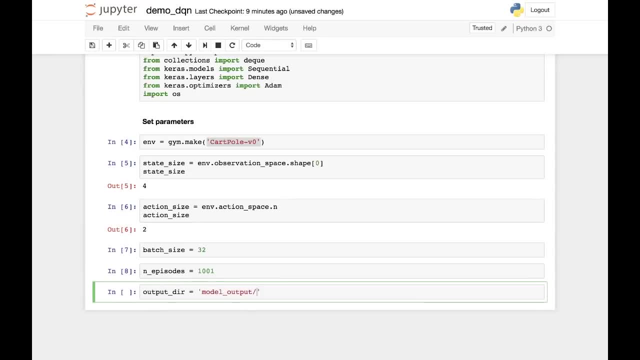 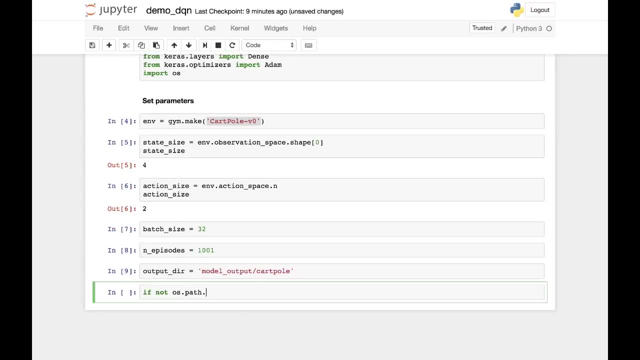 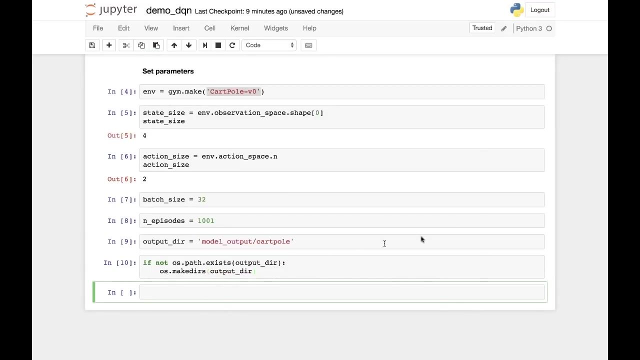 We're going to define an output directory to store our model output, And I've got this line of code here to enable us to create that output directory if it doesn't already exist. Alright, that's the preamble. Now we can actually get into defining our agent formally. 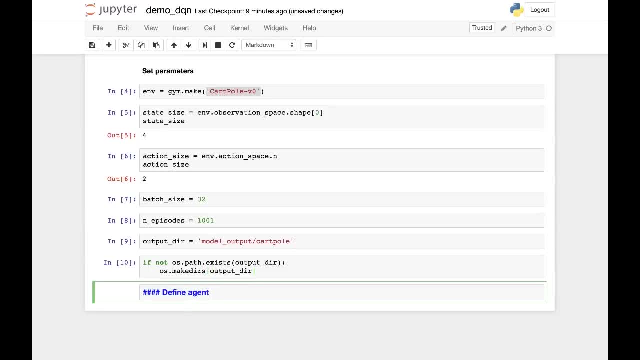 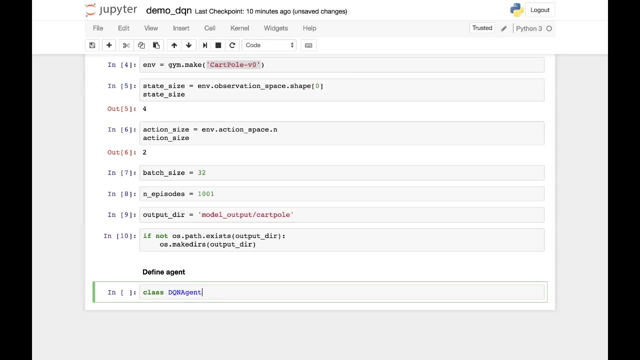 So we're going to define our agent. We're going to create a Python class to do this, So it's going to be Python class dqn-agent. It's going to have some of its own parameters, So we'll use init to define those. 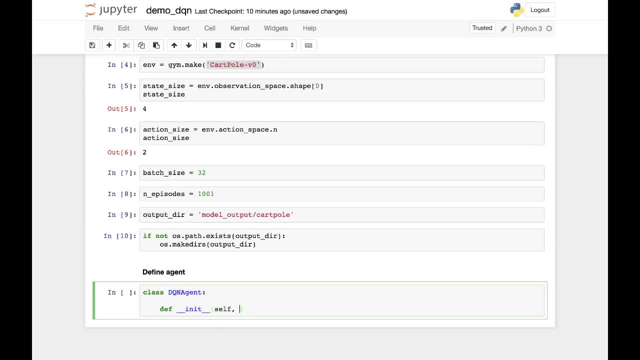 The only parameters that we need to input are going to be state size and the action size, which we defined above as four and two. So we'll just set those here so that internally they are the same as the parameters that we input And we're going to define our memory. 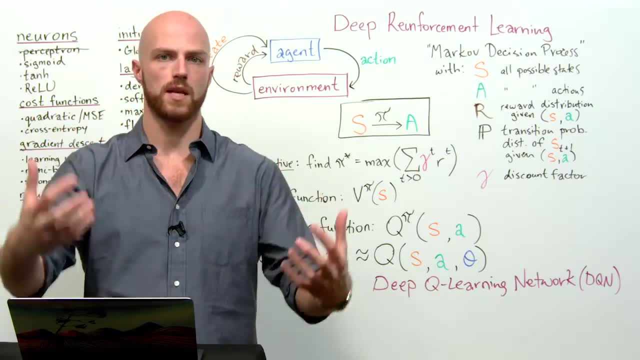 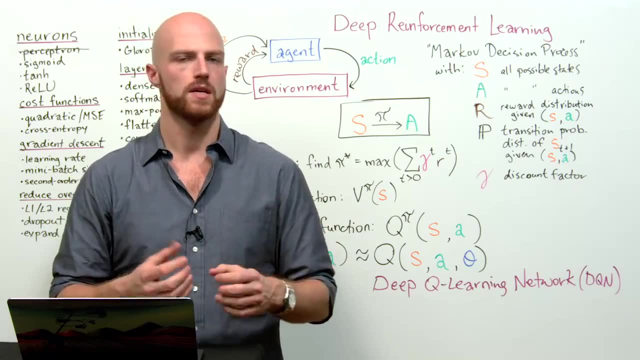 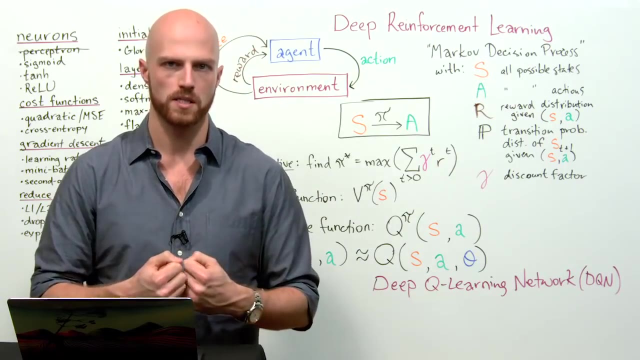 So remember that I just said. we're going to play a thousand episodes of the game And on each episode we're going to randomly remember some of the events that happened, some of the state and action pairs and rewards, And we're going to use those memories. 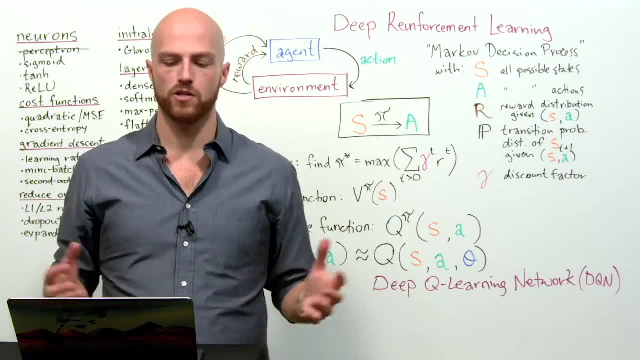 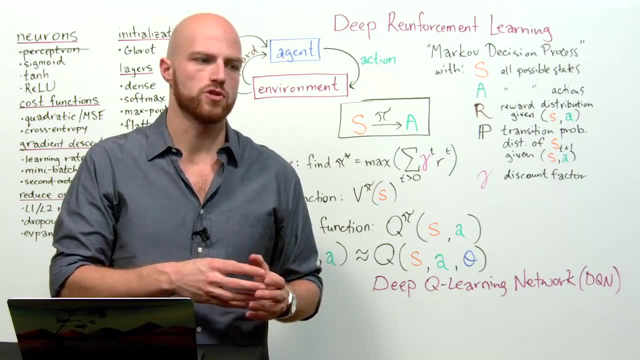 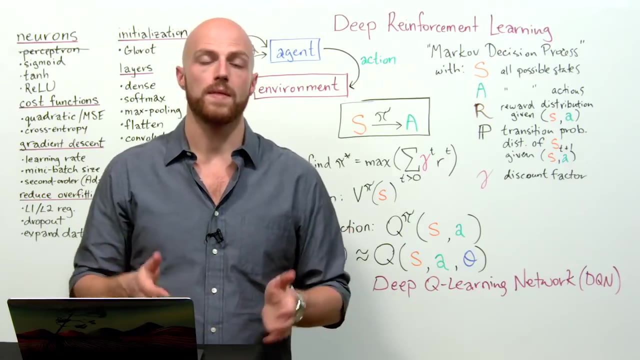 and replay them to actually train our model. The advantage of doing things this way is that it prevents us from trying to go over all of the episode and use every single event that happened. That's inefficient, first of all, because events that are closer to each other in time 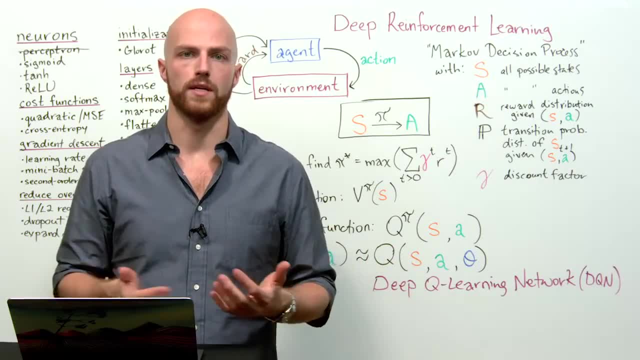 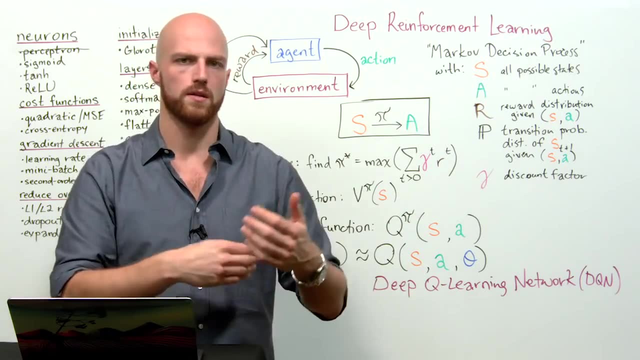 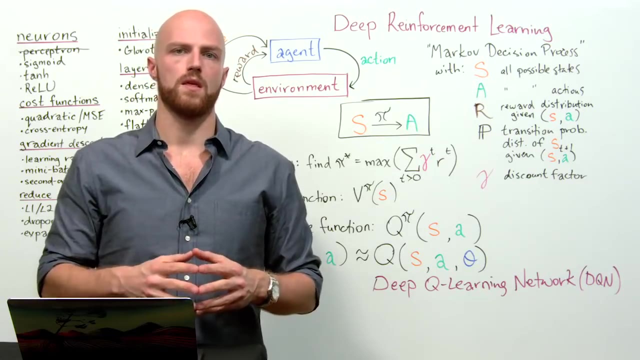 are very similar. They're highly correlated, So they don't provide very much extra information. It's worth it to sample from random spots all over the game as opposed to a bunch of continuous points in the game, So it's more efficient. The other thing: that's great. 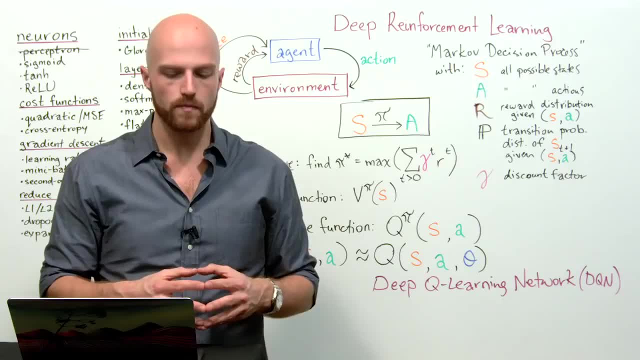 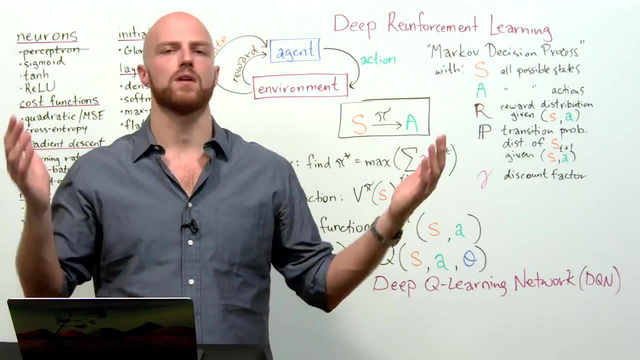 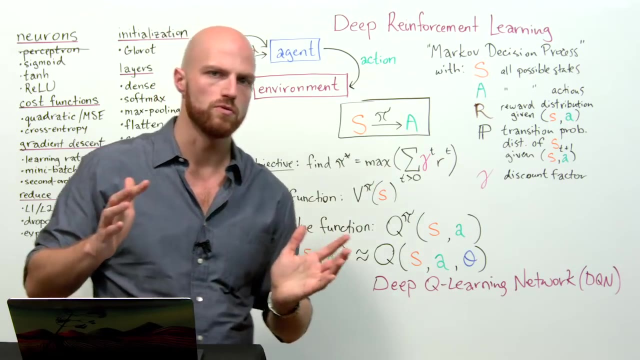 about using memory replay to train a model is that it prevents us from say we were playing some kind of video game, say even the carpool game, where if the way that our agent started to learn to play it always moved left first. 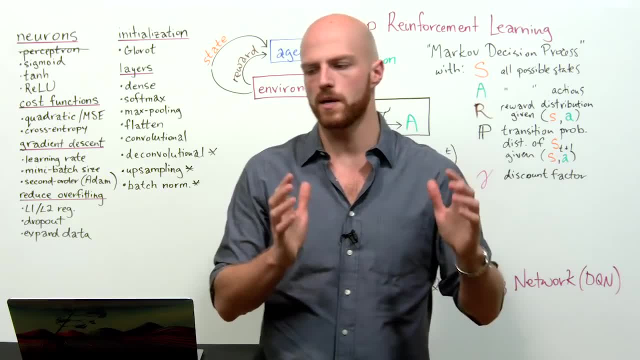 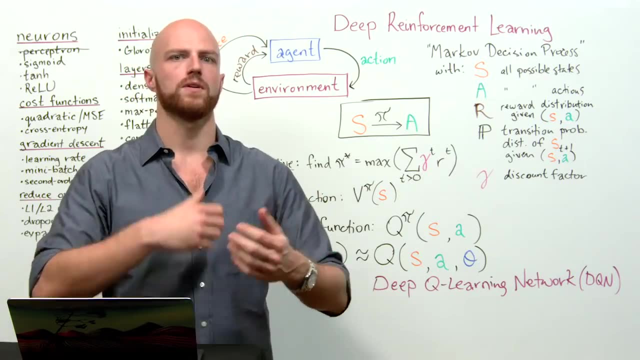 then we might start sampling only what actions are like on the left And we might not learn very much about what it's like to go right. So by sampling from all the kinds of episodes that have happened, we get a greater diversity of training data. 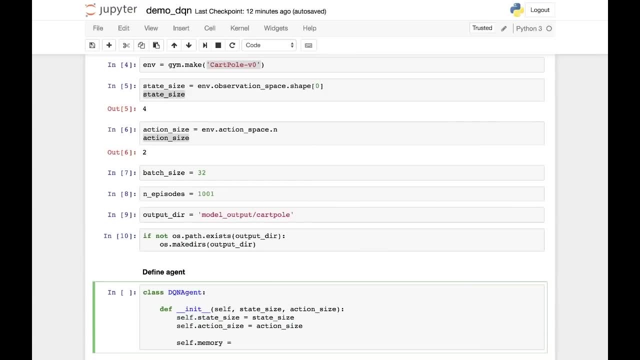 as well as being more efficient with our use of the training data. So our memory is going to be a deck with a maximum length of 2,000.. So remember that a deck is just a list, but we can add or remove elements from either end. 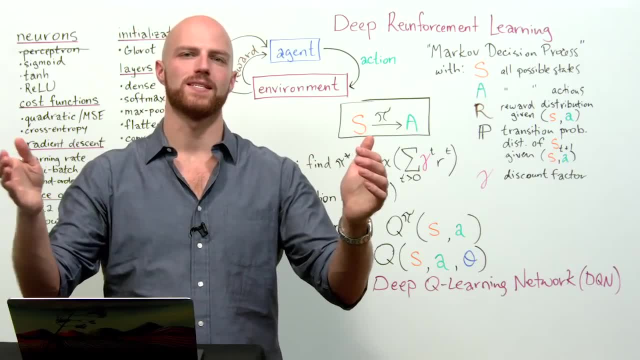 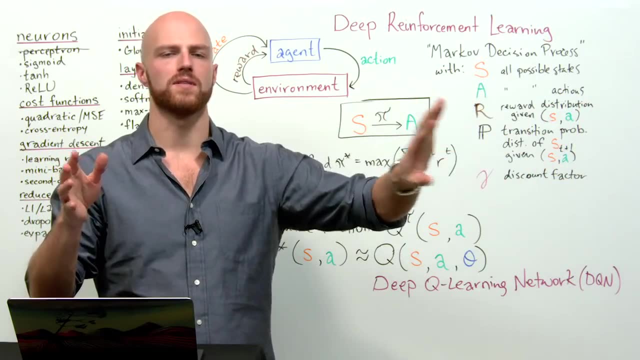 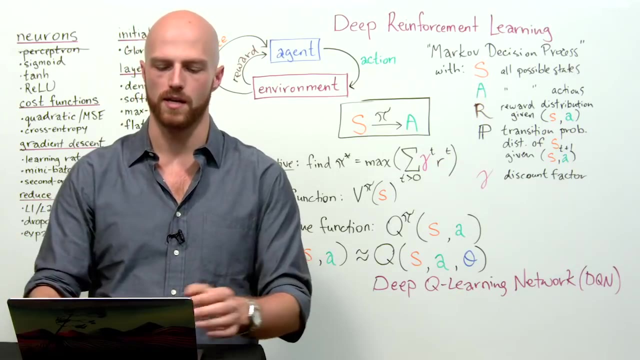 So this enables us to keep adding pieces onto our list, But as soon as we get to 2,000, the oldest elements of the deck will start to be removed. So this is more efficient than just building an infinitely sized list, If we're only interested in the last 2,000 memories anyway. 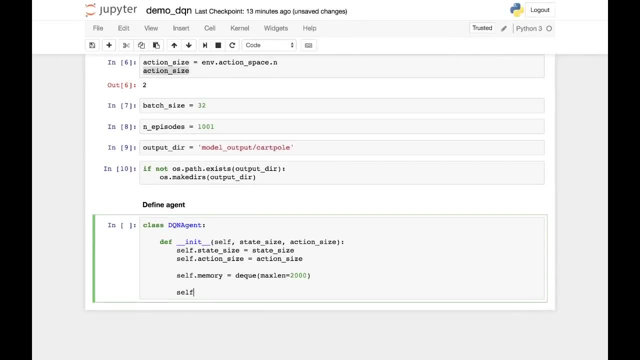 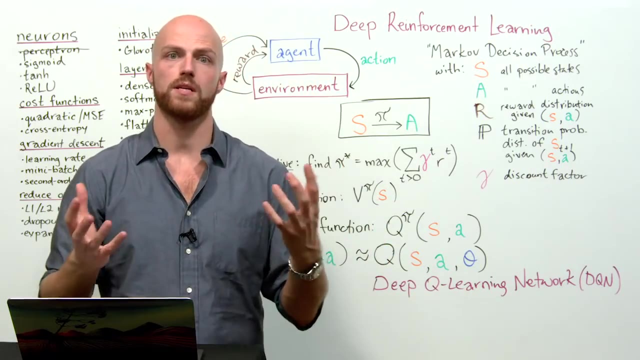 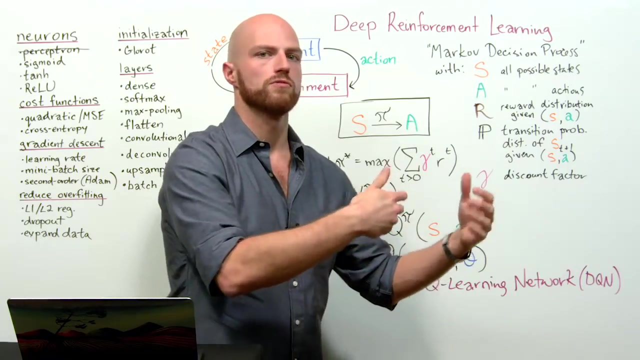 Now we have to define some hyperparameters. So gamma is the first one. So gamma is this discount factor. So this is how much to discount the future reward. So, as I mentioned earlier when we were discussing theory, specifically the next, when we're trying to estimate future reward. 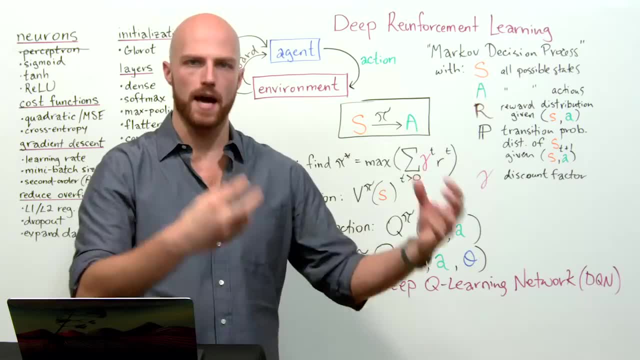 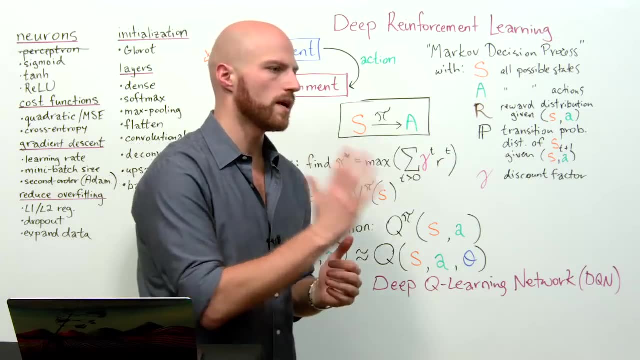 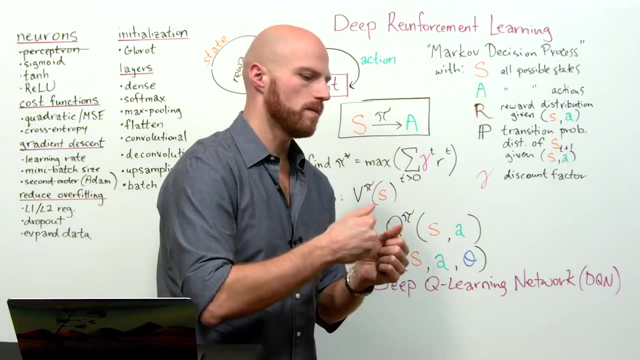 the next time step is easier to guess. we're more likely to guess correctly than five or ten time steps from now. So when we look ahead to estimate how much reward we're going to accumulate based on the actions we take, we want to weight the upcoming actions. 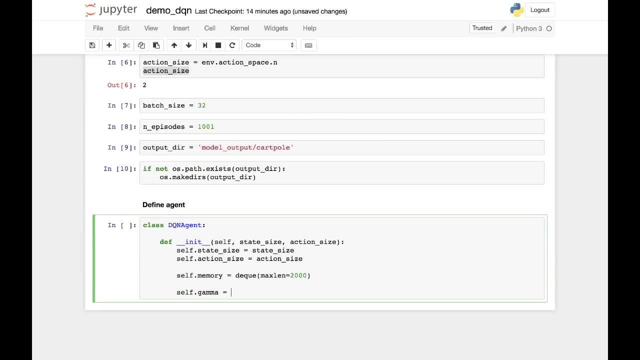 more heavily than the ones that are in the distant future. So we use this gamma parameter to discount future reward. Another hyperparameter for our model is epsilon. We haven't talked about this yet, but epsilon is really important. So epsilon is the exploration rate for your agent. 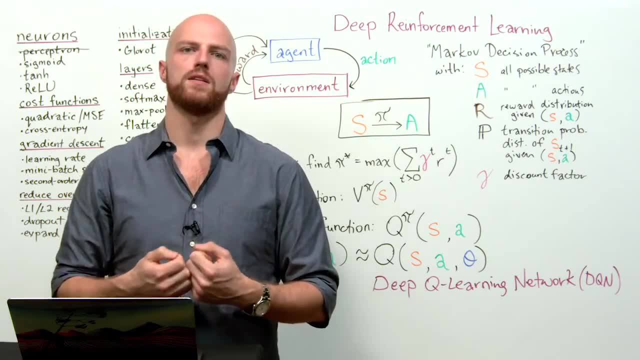 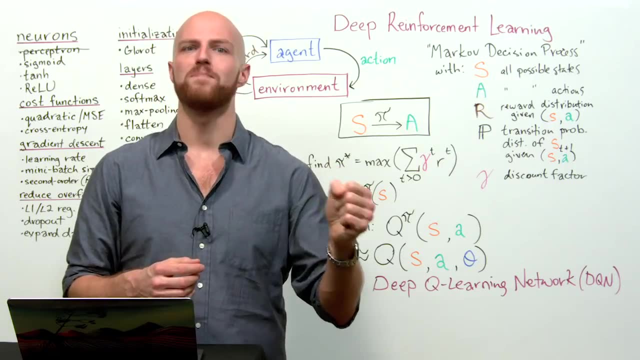 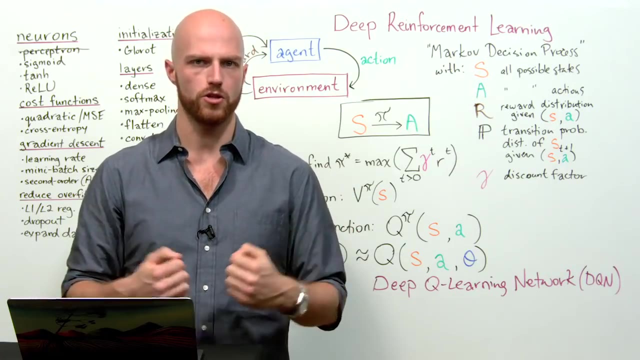 So there are two kind of modes that your agent can take action with. The agent can either try to take the best possible action based on what it's learned, So this is what we call exploitation of existing knowledge. The alternative to exploitation is exploration. 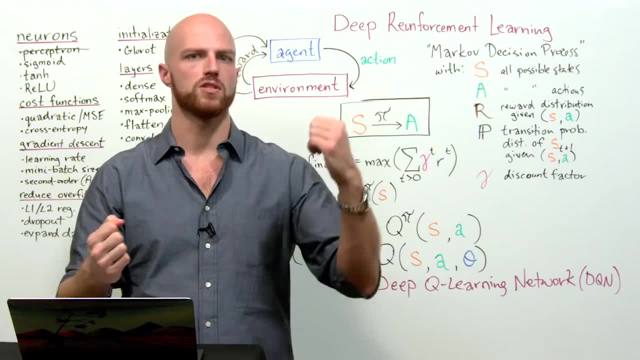 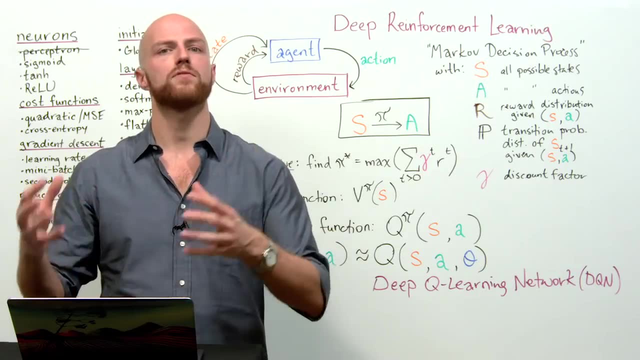 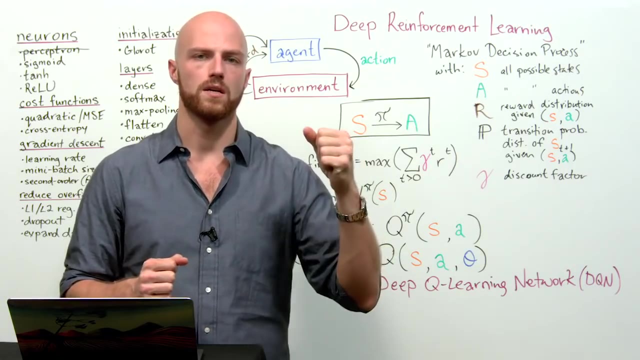 And the reason why we might want to explore instead of just exploit is because the kinds of environments that deep reinforcement learning agents have to explore are often very complex, And if we only stuck with exploiting our existing best practices then we might not uncover something new that's helpful. 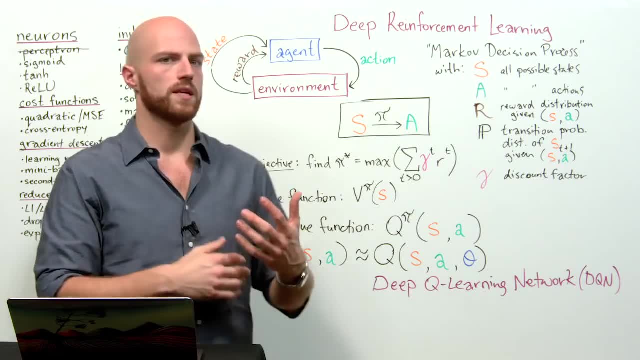 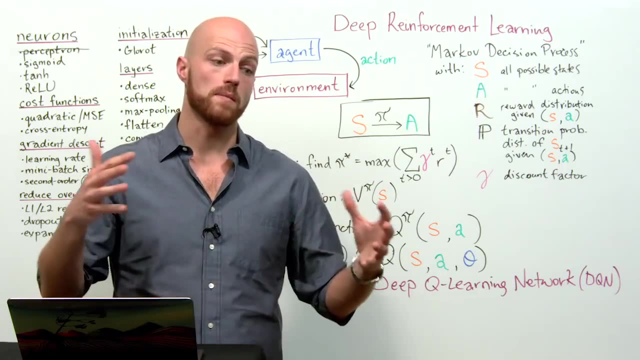 This is particularly important because the deep reinforcement learning environments can evolve over time. So in the carpool game that doesn't really happen, But in some other kinds of games or if you imagine a self-driving car, you can get into new kinds of situations. 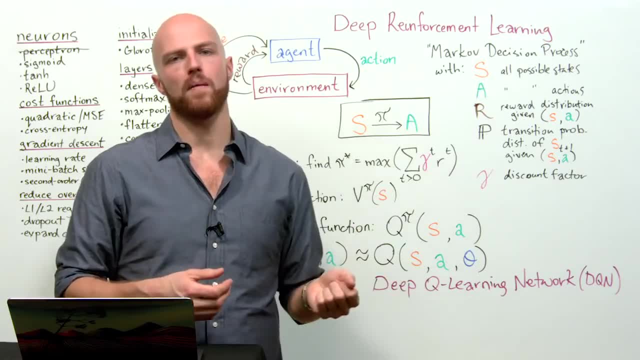 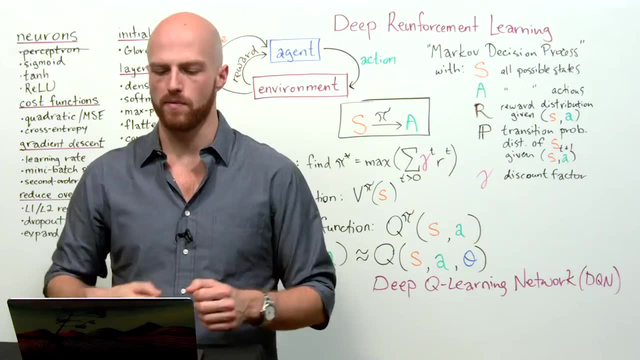 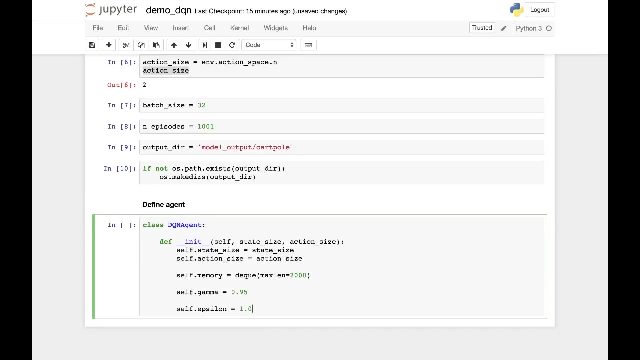 where maybe just exploiting isn't the optimal course of action, where it's worth spending some of your time randomly exploring a new type of action. So the epsilon, the initial epsilon. so what we're saying here by setting it to one is that our initial exploration. 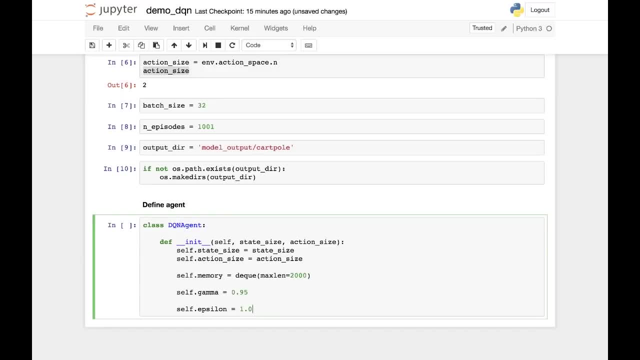 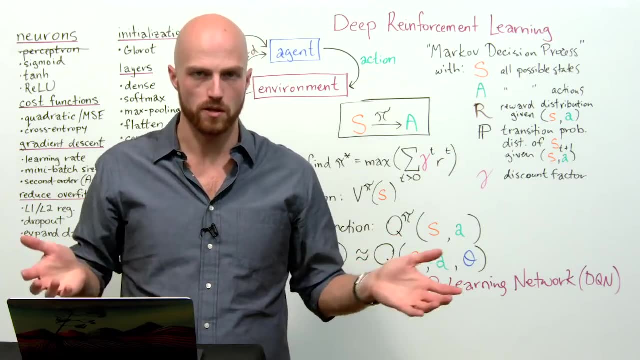 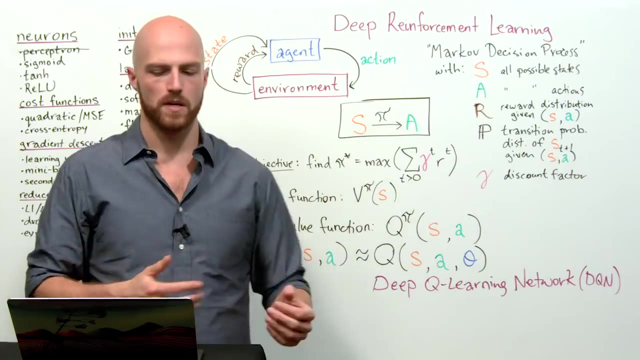 versus exploitation rate is going to be skewed 100% towards exploration. So at the very beginning of training our agent, we assume- and I think this is the correct assumption- that the agent doesn't know how best to exploit the information about the environment. 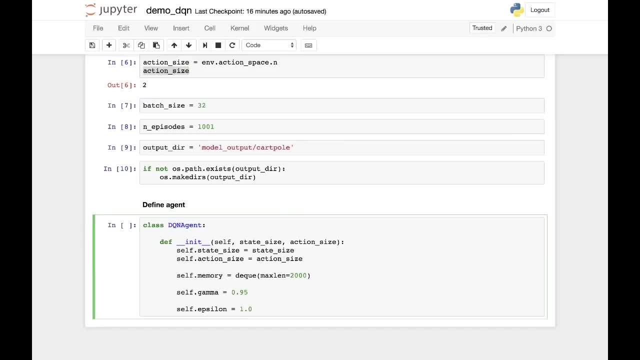 And so we're just going to explore at the start. However, we're going to decay that epsilon over time, So this parameter allows us to. with ongoing training, we decay our epsilon so that we slowly shift our agent from exploring at random to exploiting the knowledge that it has learned. 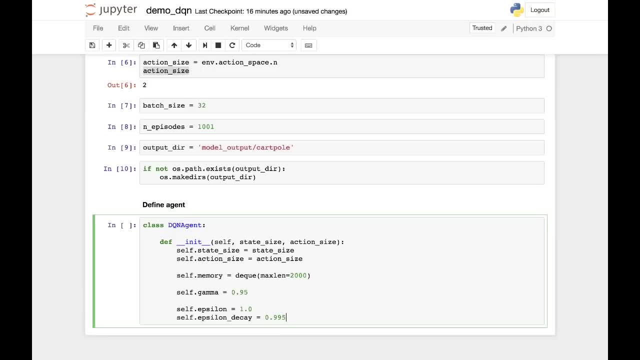 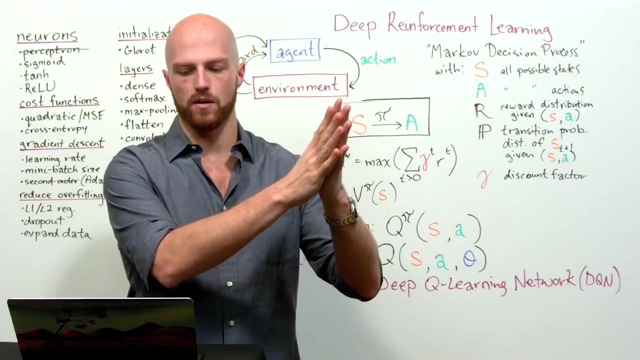 And over time this exploitation starts to dominate and we do very little exploring. But we can set a floor on how low the epsilon can go, So we'll set that here The minimum. so this means that at the very least, even after we've decayed our epsilon- 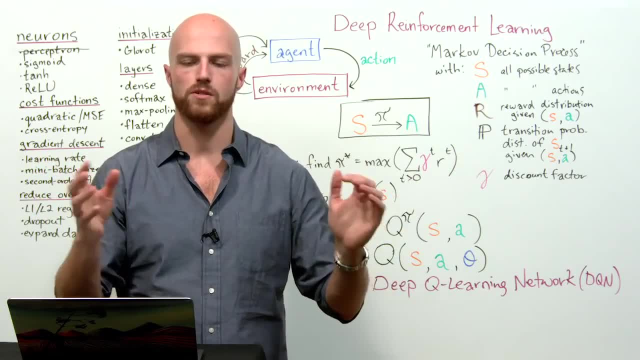 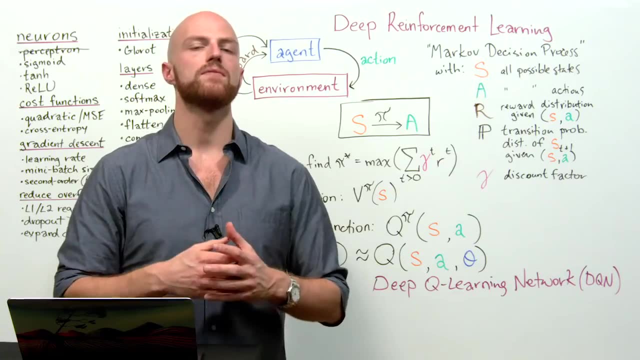 all of the way towards zero. the lowest that we'll let it go is to 0.01, which means that 1% of the time the agent will explore even you know that's the very minimum. So we start exploring 100%. 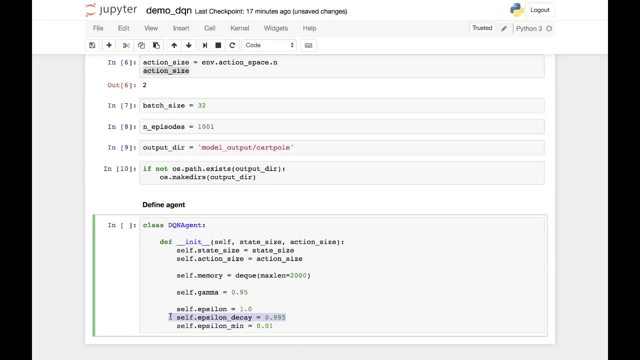 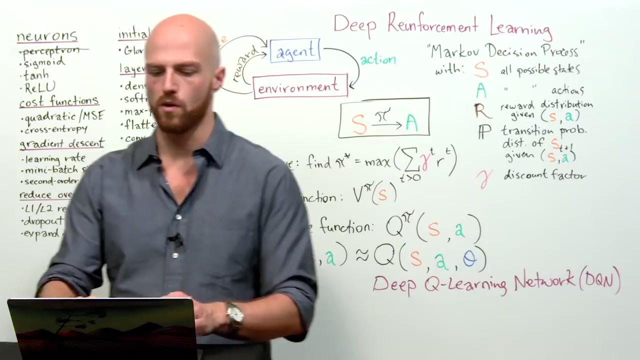 We use the decay to shift that exploration towards exploitation over time until eventually we reach this minimum amount of exploration which we've set to 1%. Our agent also has a learning rate. This is the stochastic gradient descent learning rate. This is the step size. 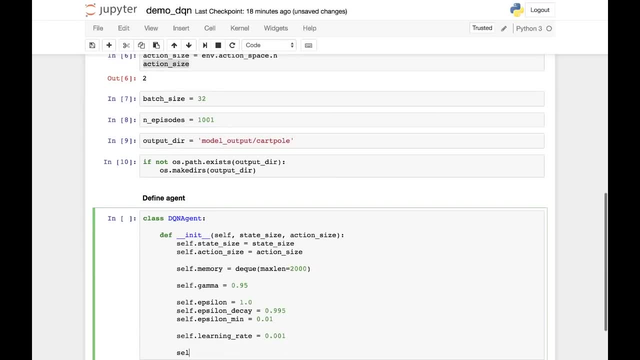 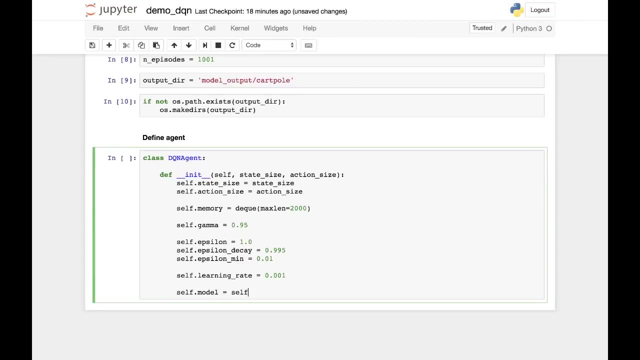 for our stochastic gradient descent optimizer. And the final parameter to set here within the agent is this build model, which is just. it's just a private method that we're setting up here. This means that the method can be used only by this particular instance of the class. 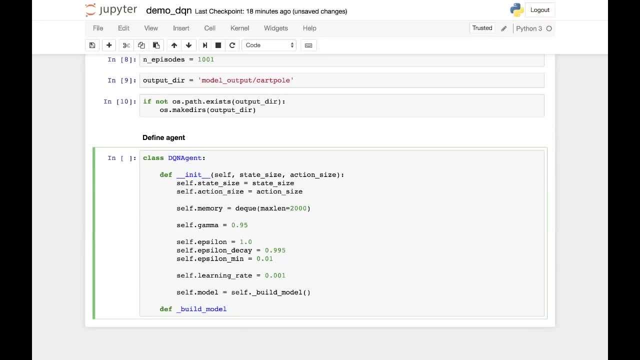 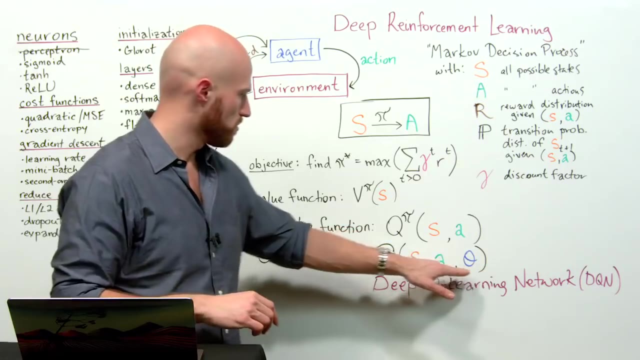 Let's define that build model method. So it's in this build model private method that we're going to define our dense neural network for approximating Q star. So this is going to be the usual way that we set up a Keras model. 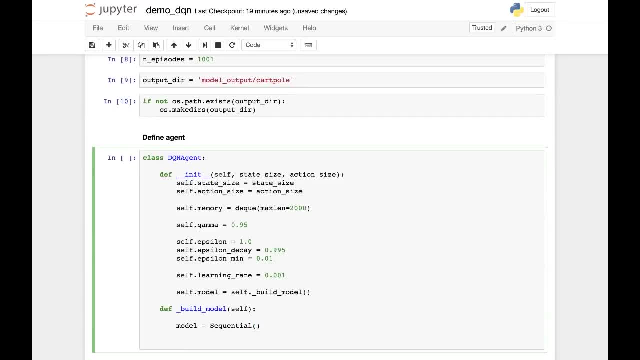 So we're going to use sequential And the first layer is going to be dense. All of the layers are going to be dense. The first layer- we found that 24 neurons works well. The input dimensions is equal to the state size. 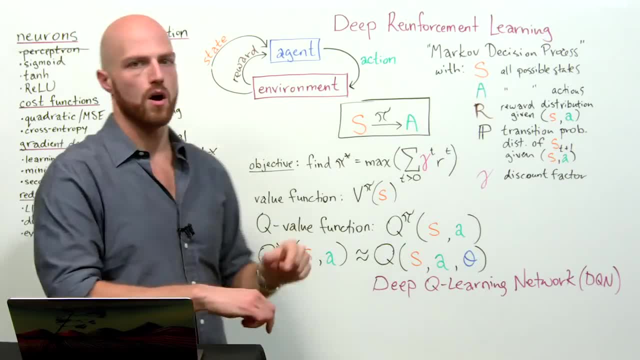 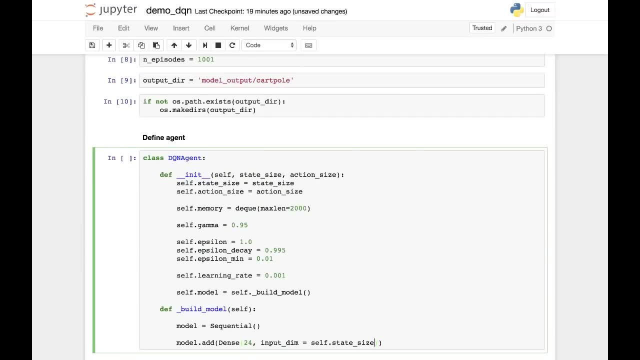 So the four states of the environment are the inputs into our model And we are going to set activation to our good old friend rectified linear unit. Notice a problem? Surprise is there. ReLU is our favorite. In the next layer we are likewise. 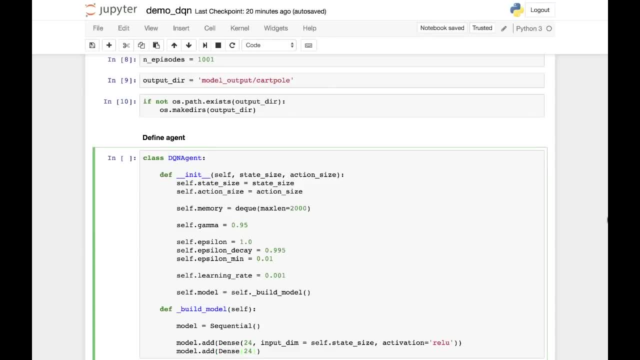 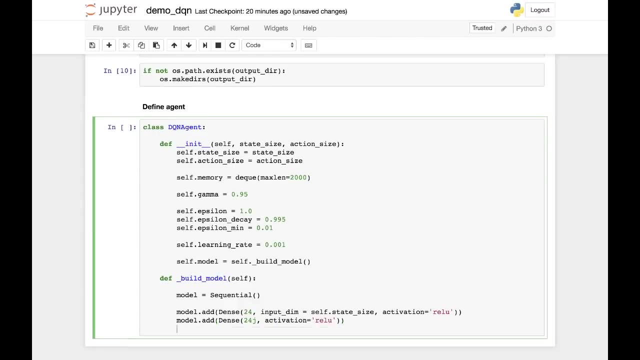 of course going to have a dense layer And it's going to have 24 neurons And again, activation is going to be rectified linear unit. That's actually it for our hidden layers. It's a relatively shallow neural network actually. 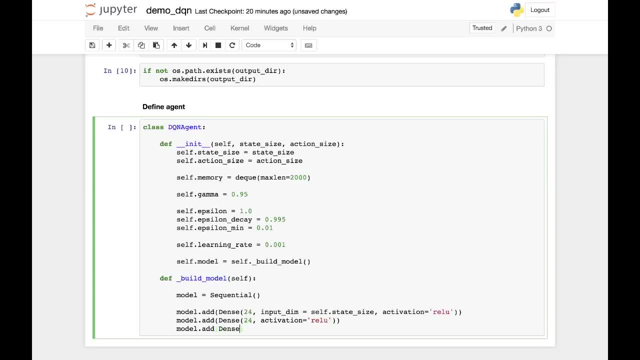 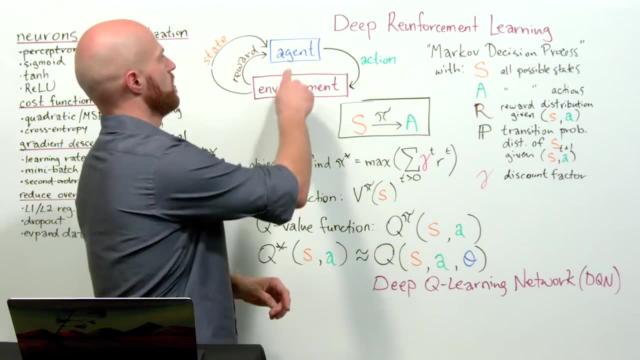 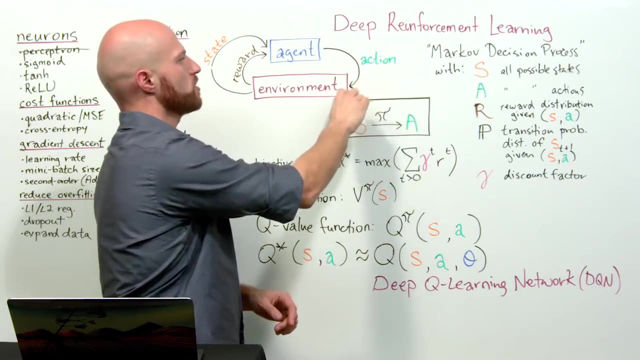 Because now we're going to define our output layer, which has as many neurons as we have possible actions. So this model is sitting here in the middle between taking states as inputs and actions as outputs. So the action size, the two possible actions. 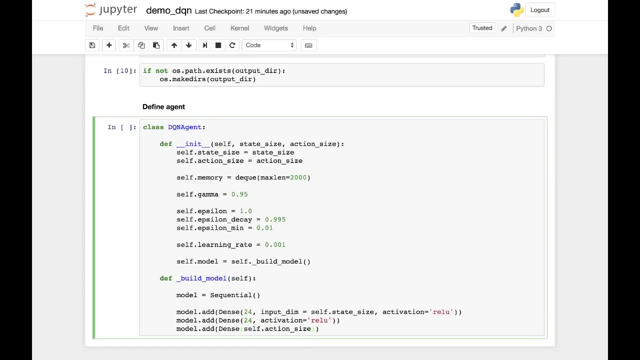 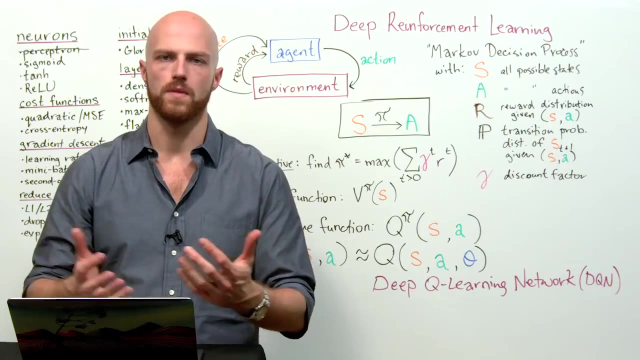 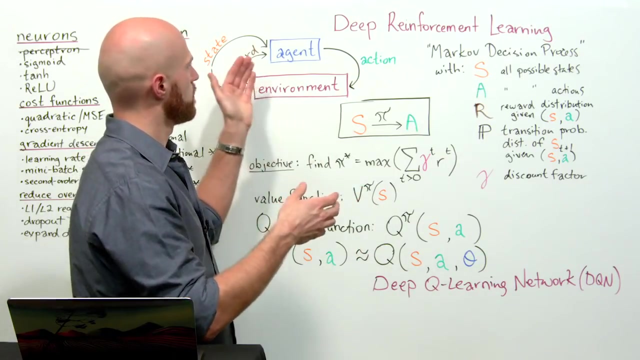 right or left are the output neurons, And these are going to have a linear activation. The reason why we have a linear activation is that we are directly modeling these actions. We don't want some abstract probability. We want the action estimates to be direct. 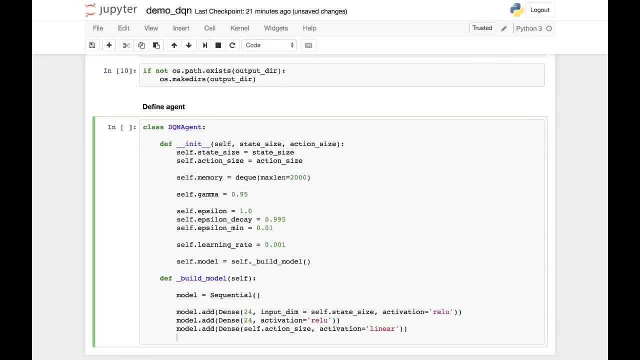 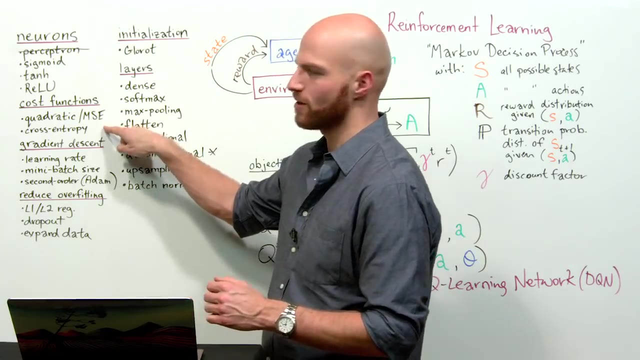 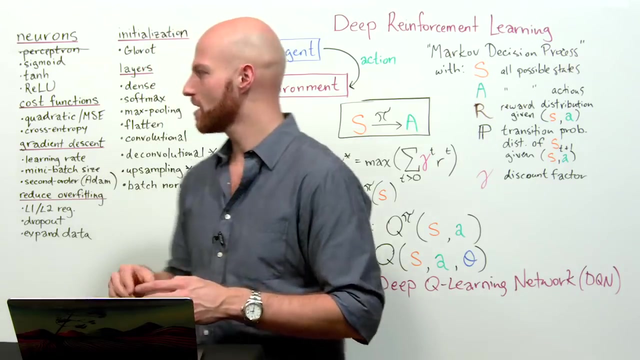 out of this neural network. Now we are going to compile the model. We have almost always used cross entropy as our cost function. It turns out that for this particular configuration of our agent, mean squared error unusually ends up being a good choice. You're welcome to play around. 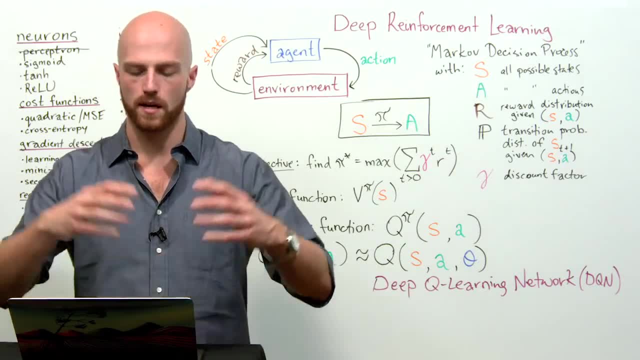 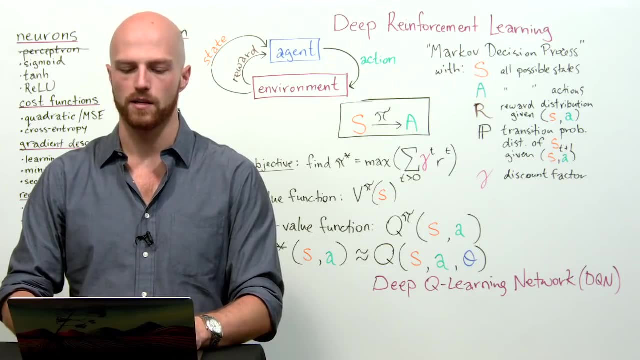 with your hyperparameters and try using cross entropy as well, But it ends up being that, given the particular parameters of this specific problem that we're solving, that the mean squared error loss is unexpectedly the better choice of loss And we need to pick our optimizer. 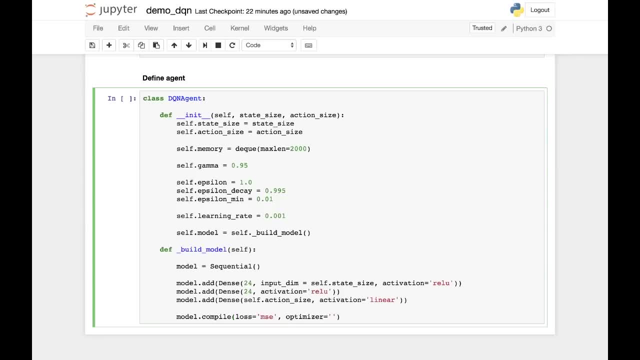 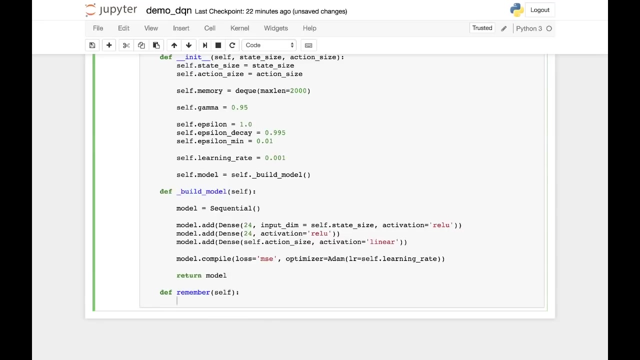 which is going to be atom, And atom is going to have the learning rate that we specified up above. Okay, so this method is going to return the model. The next method to define is the remember method. The remember method has a bunch of parameters. 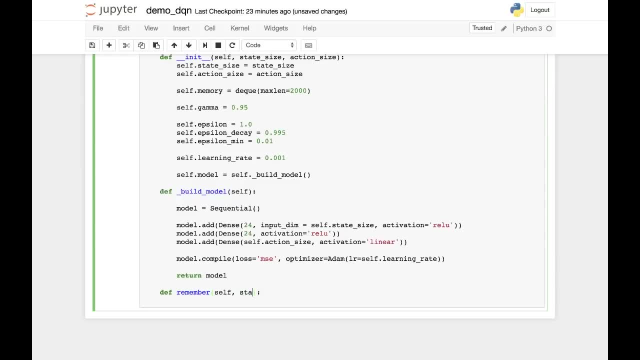 So the remember method takes on state action reward next to state and done as parameters. So this remember method is really important. It's one of the most important bits of how this DeepQ network works well, Alongside the memory replay. 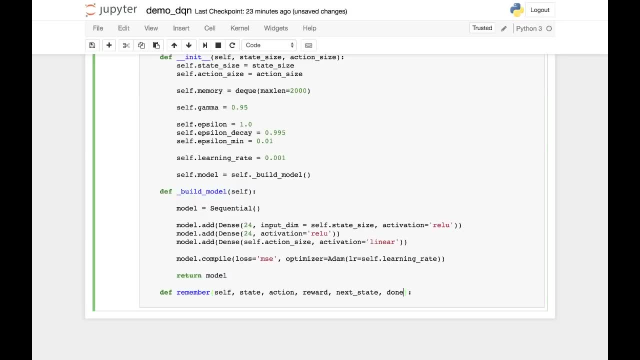 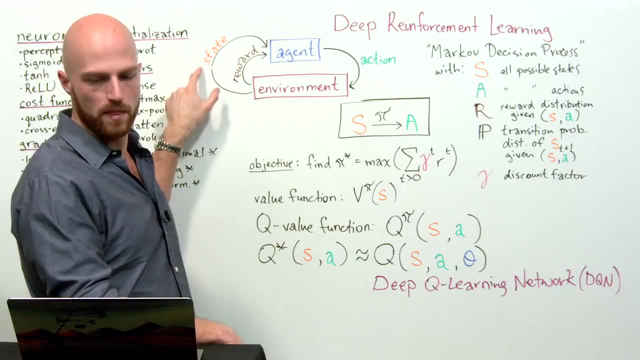 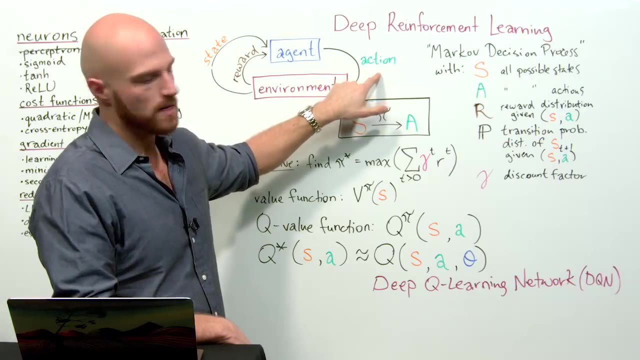 that we're going to go into after we define this remember function, And so this remember function takes in state at the current time step, It takes in the action at the current time step, It takes in reward at the current time step And it takes in the next state. 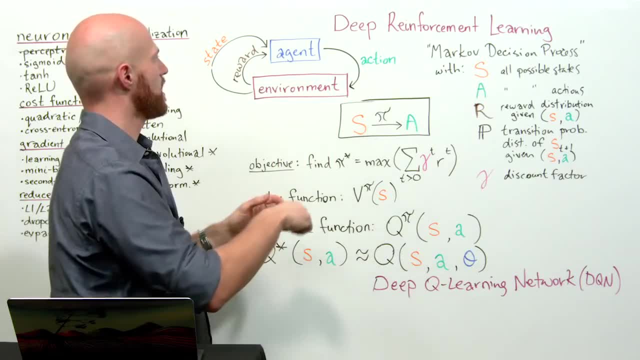 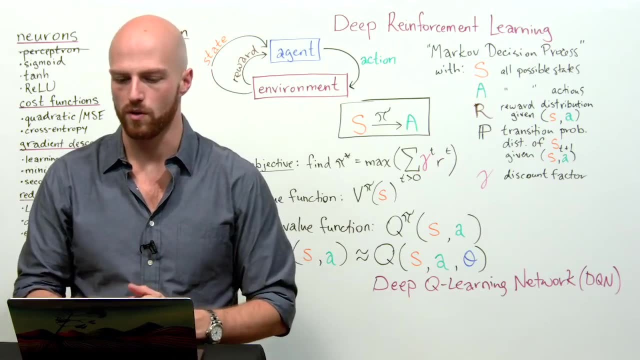 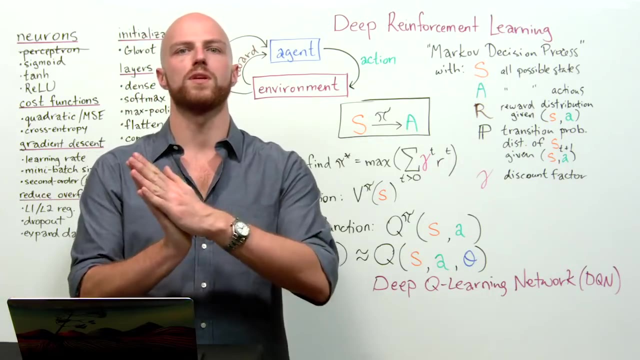 So it enables us, given a particular state-action pair, to model what's going to happen in the next state and what kind of reward we can expect to receive. Done is simply a parameter that lets us know whether the episode has ended or not. 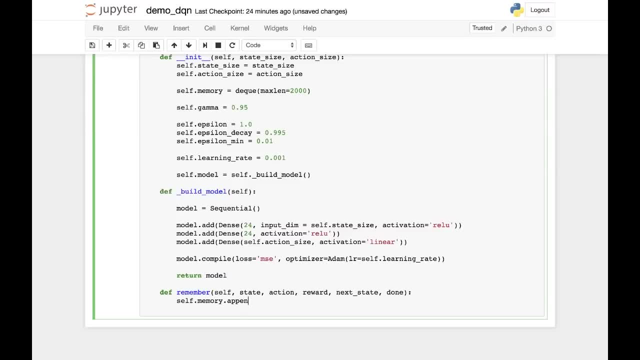 The only thing that this remember method is going to do is to append this information into our memory deck. So it's simply going to append the state, the action, the reward, the next state and, done So, you can just copy and paste those in. 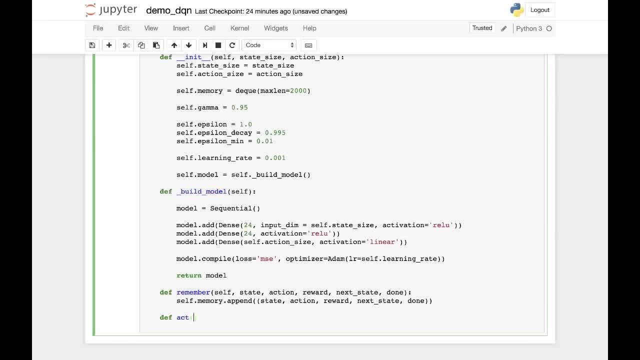 The next method is the act method. We only really have one more method after this act, which is the replay one, where we do all. the training Act takes in only the state. So in this method we are figuring out what action to take. 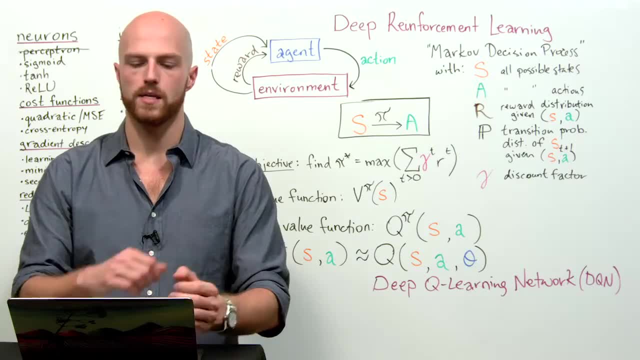 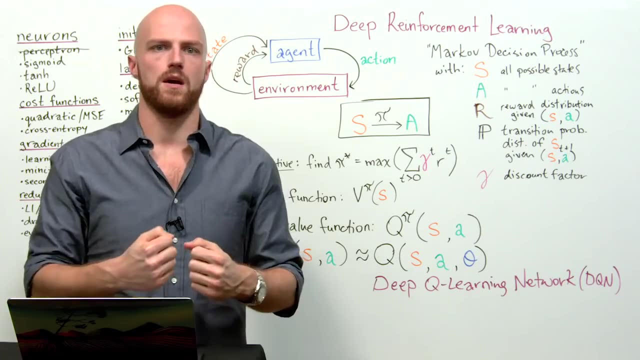 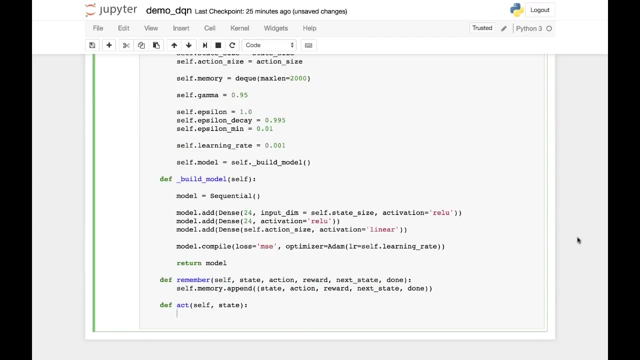 given a state. So, as I mentioned earlier, based on the epsilon, we're going to either explore randomly or we're going to exploit the existing information that we have accrued within our theta weights of our dense network. So we're going to use the random. 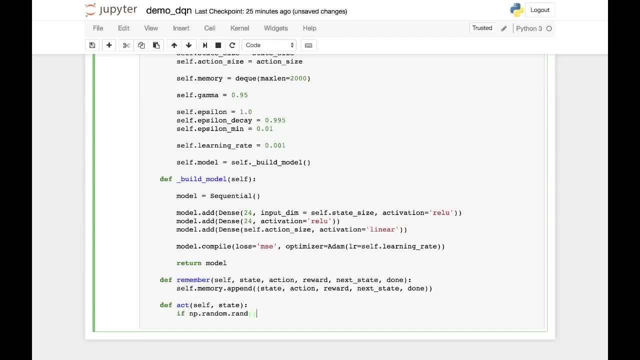 we're going to sample a random value between 0 and 1.. And if that value is less than or equal to our epsilon, then we are going to just act randomly. So this means that we will simply pick a random action, which in our case means: 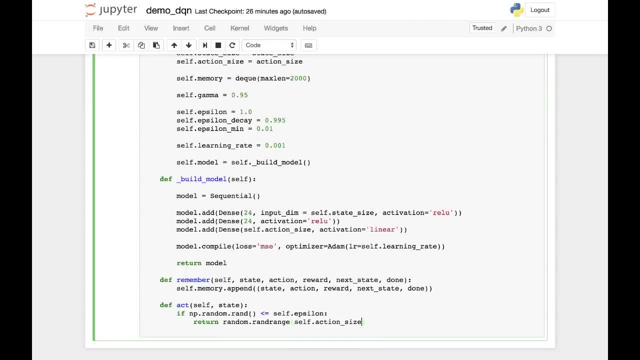 we'll just go right or left at random. So this is the exploration mode. So if we randomly select a value that is less than 1 on the range 0 to 1, then we will take an exploratory action, a random right or left. 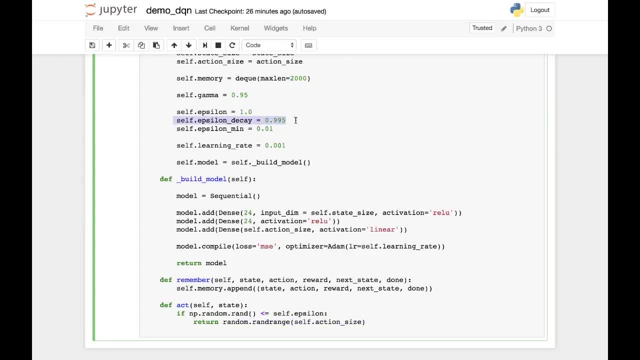 And then, over time, as our model trains, the epsilon will decay, And so we will tend towards exploitation instead of exploration. So how do we exploit? In order to exploit our existing knowledge, we use the theta weights and the predict method on our model. 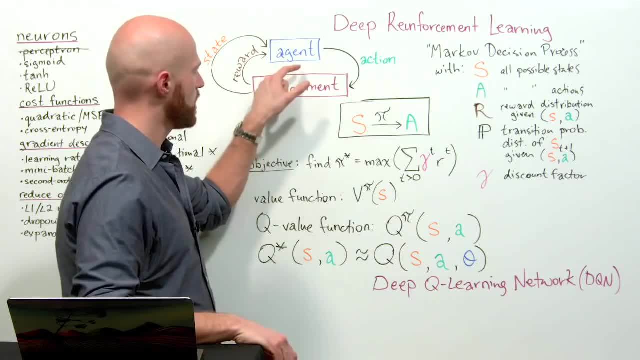 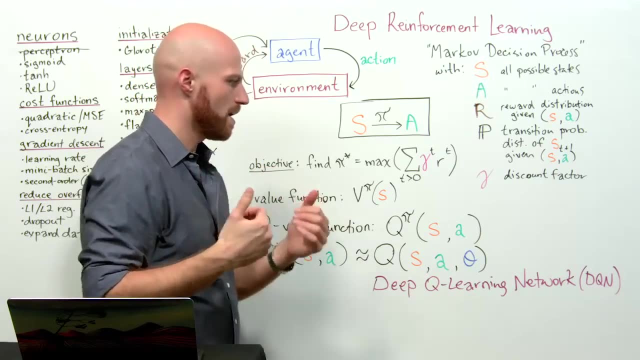 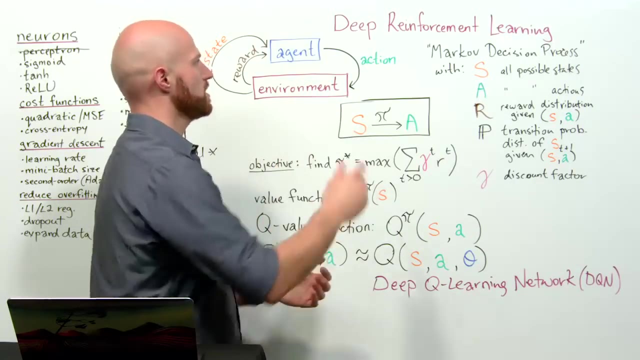 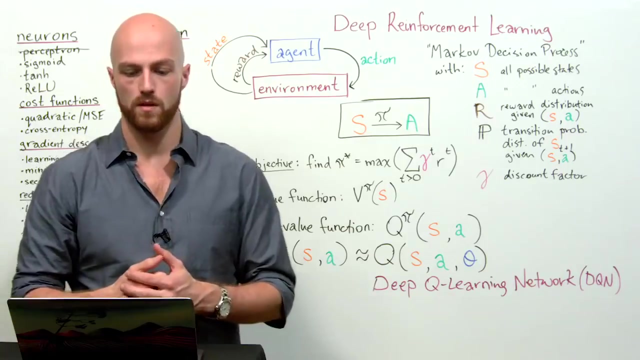 So we pass into our agent when we want to exploit, We pass in state information and we use the predict method on our deep learning model inside the agent to have a guess at what the best possible course of action is to maximize our future reward, And then we simply return. 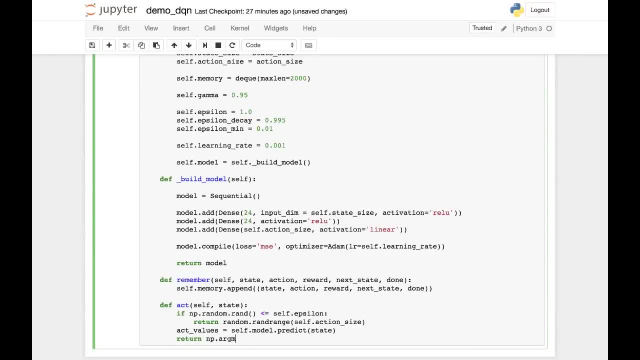 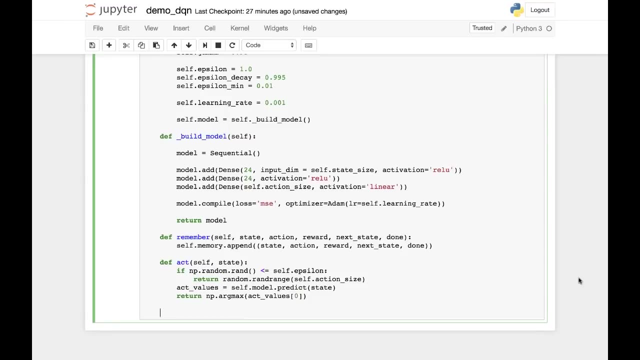 from this method, the action that is determined to be the best choice. So that's it. Finally, this is the. There's two other tiny little methods after this about loading and saving data, But this one here, this replay method, this is the bulk of all we have to define. 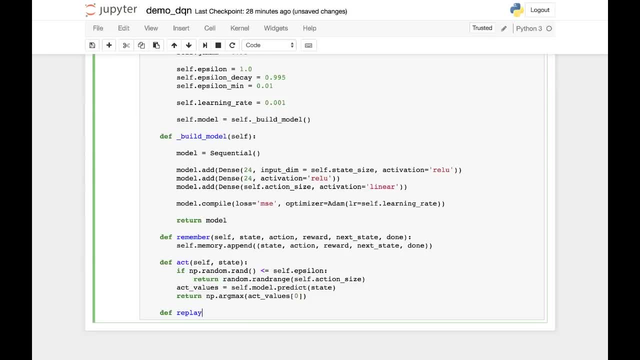 still within our agent. So the replay method. this takes in as its only parameter batch size. This is really where the action happens, Really cool stuff. So the first thing that we want to do is we want to create a mini batch that is a random sample. 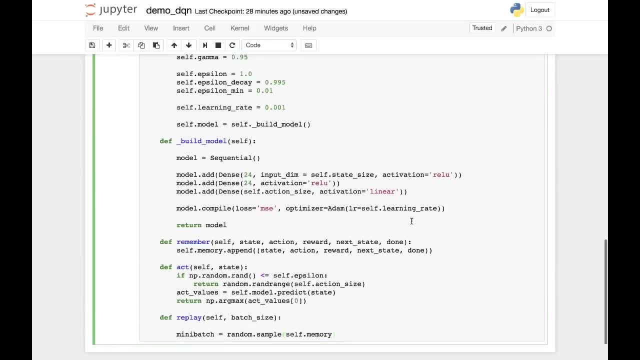 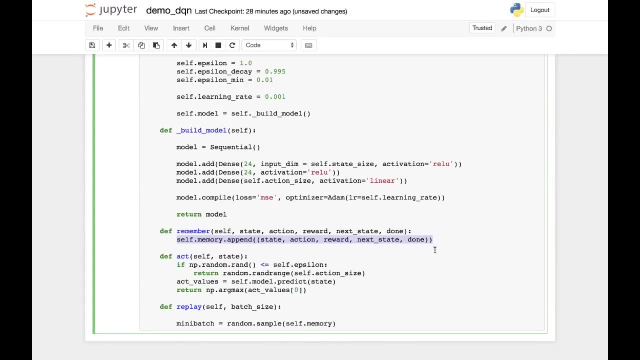 from our memory. So remember, we've been building up this deck of memories with the remember method- See how that happens later- And we're now going to, with our memory replay, randomly sample some of those memories And the number of memories that we're going to sample. 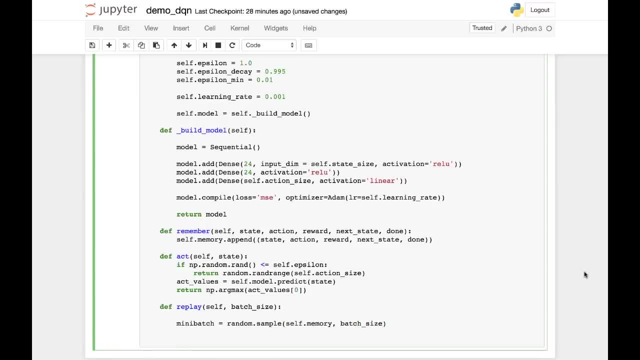 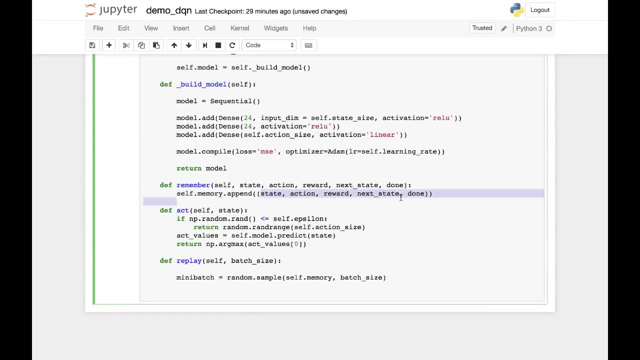 is our batch size, And so every one of our memories has a state, an action, a reward, the next state, and whether the episode is done or not. So, before each of those values- state, action, reward, next state done- 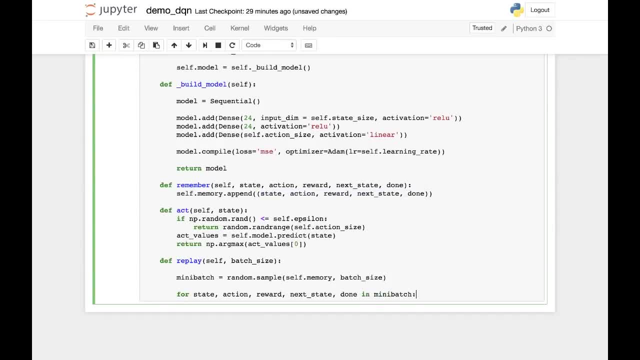 in our mini batch if the episode is ended, so if we've either reached the maximum number of time steps that are allowed, which, with the card poll game version zero, is 200 steps, or if we've ended the game by dying, by either the poll getting too large of an A 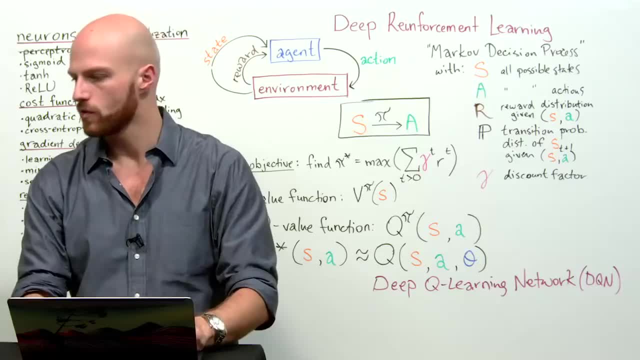 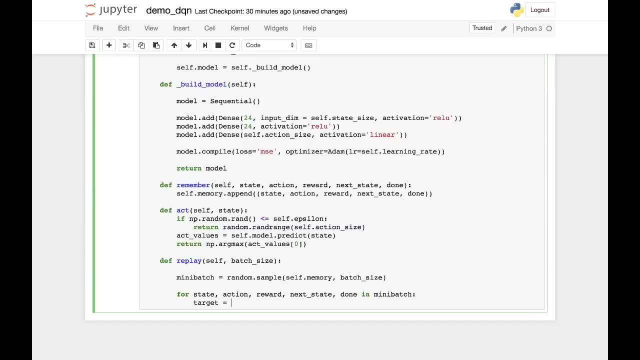 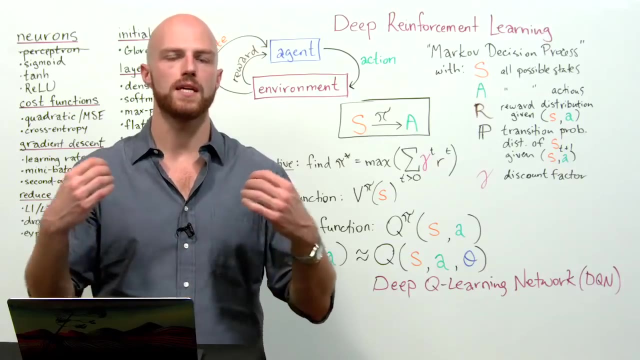 or by moving the cart off of the screen. if that happens, then we're done, So done equals, true, And in that case there's no mystery about what our target is. Our target is simply equal to the reward. We know how the game ends. 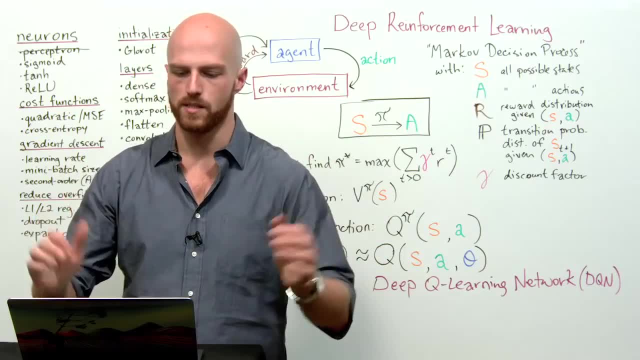 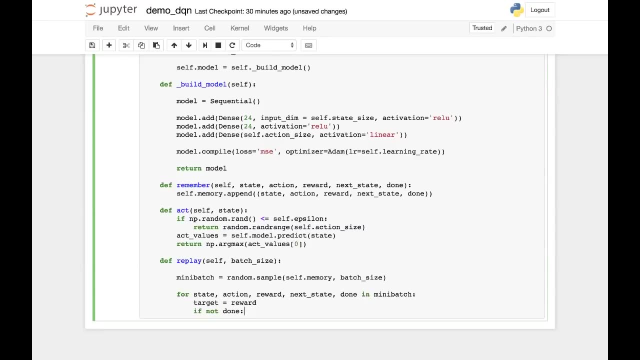 We don't need to make predictions about future reward. This target is equal to reward. If we're not done, however, then we have to make some estimates about what our future reward would be, our discounted future reward. So in that case, 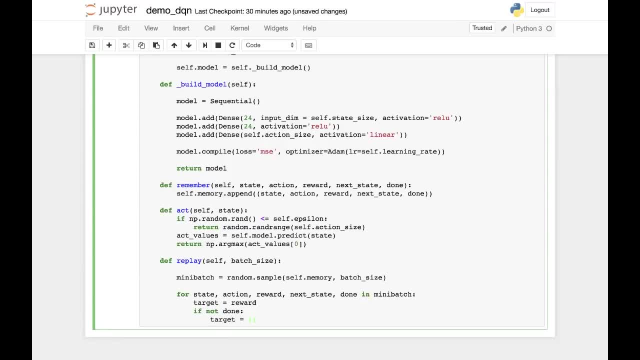 our target is equal to our reward that we know we get at the current time step, plus our discounted. so we use gamma to discount future reward times, our estimates of future reward. And the way that we estimate our future reward is by using our neural network. 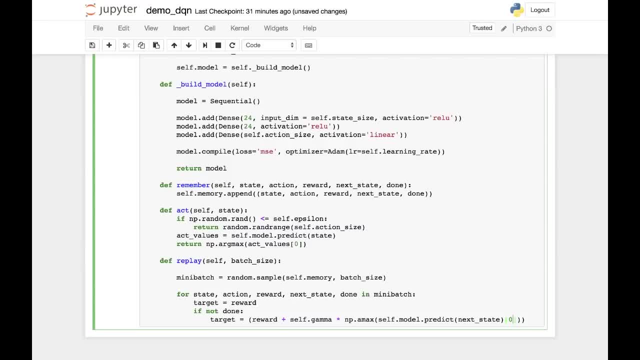 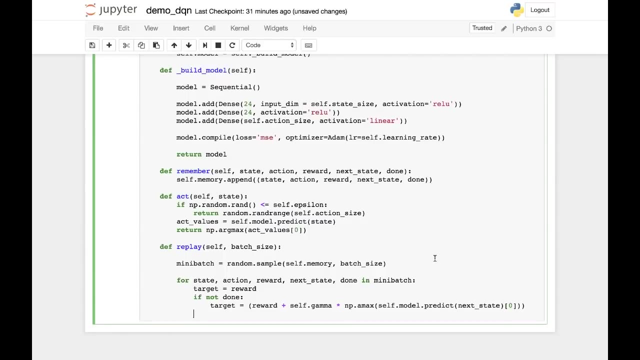 So here our neural network, based on information about the next state being passed into it, can predict what the future reward should be. The next step for us here is to map that maximized future reward to the current reward, and we're going to do that. 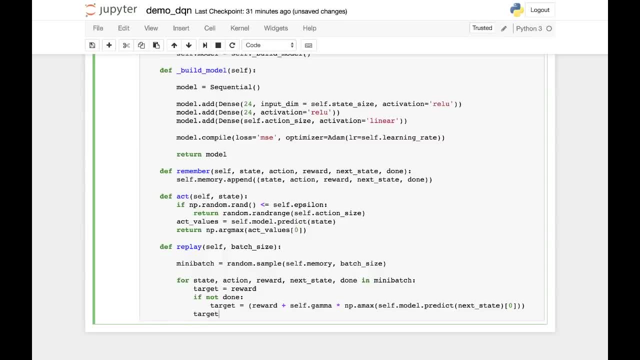 with the theta as well. So here we define our estimated, we use our neural network, again here, to estimate our target given the current state, and then we map that target from the current state to the future state with this line, And then, finally, 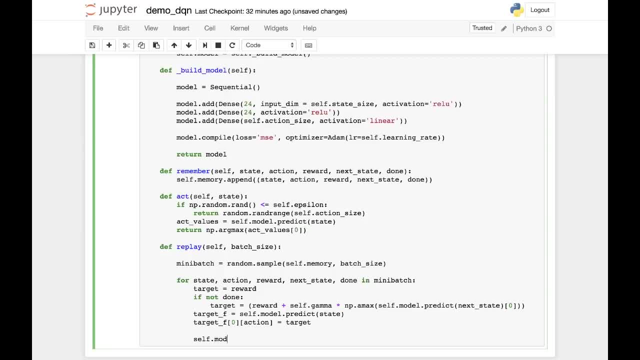 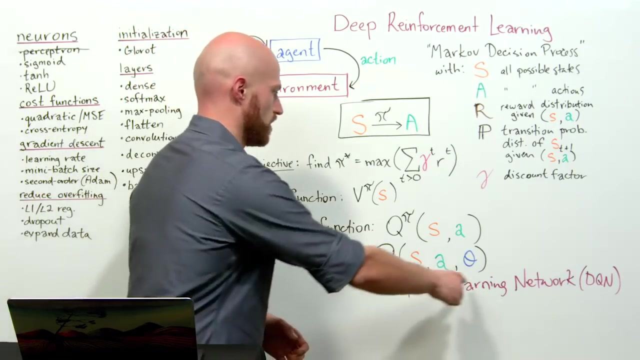 with all of that information all together we can fit a model to train. So our x's into the model, our inputs into the model, are the current state, Our y in the model is the predicted future reward. And so here we're, modeling this relationship. 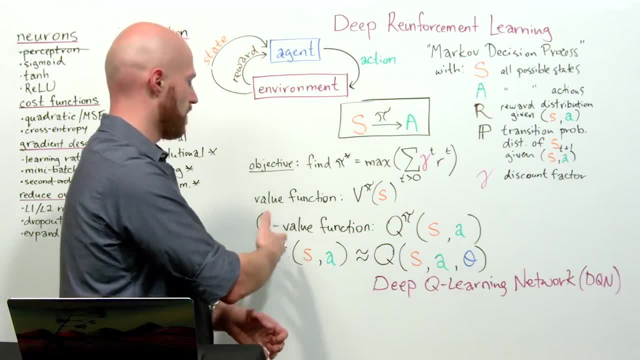 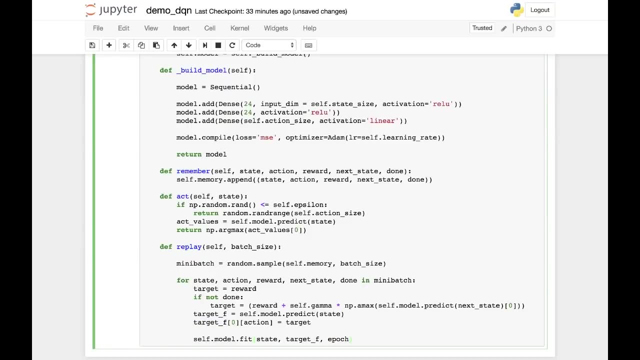 We're using deep Q learning to model the optimal Q star, And we only do that for a single epoch, because we only really have one moment of information, one single memory to replay here And we don't want any verbosity because we would just be getting. 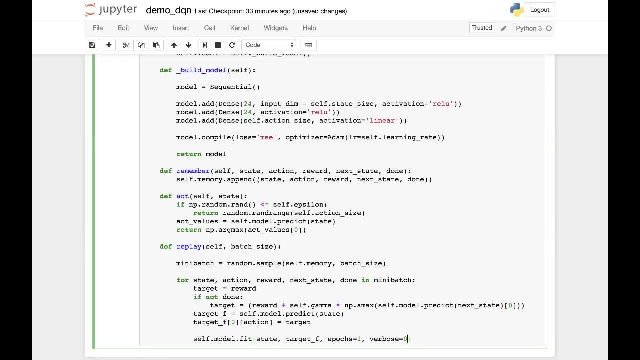 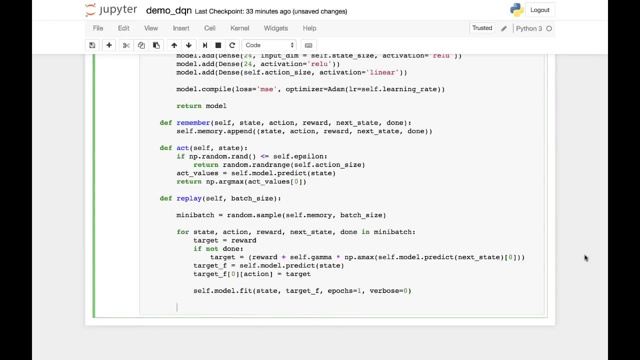 a lot of verbosity output. we're going to decide exactly what we want to output to the screen later on. The final thing to do inside of our replay method is to decrease our epsilon. So with each time step we want to be decreasing our epsilon. 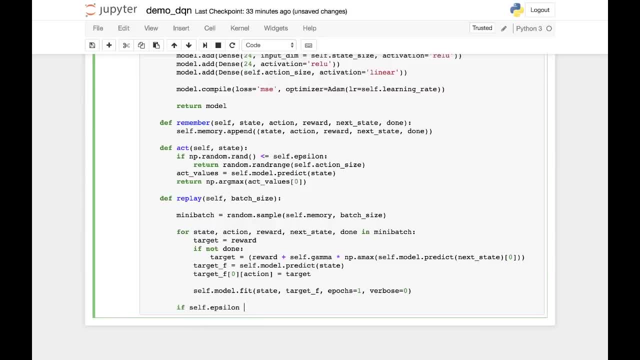 So if epsilon is greater than our epsilon minimum, then set our epsilon for the next replay to be a little bit smaller, decaying it a little bit by multiplying it by our epsilon decay. Okay, that's the end of the bulkiest method. 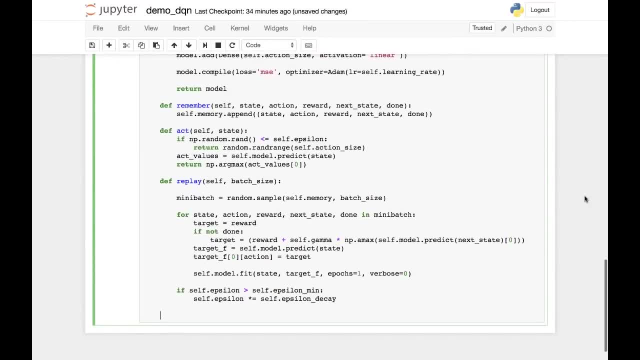 We just have two tiny little methods for saving and loading data so that you can save information and reload it later, Save your model weights. So you just simply have this load method for loading weights and we define a save method to save those weights for loading later. 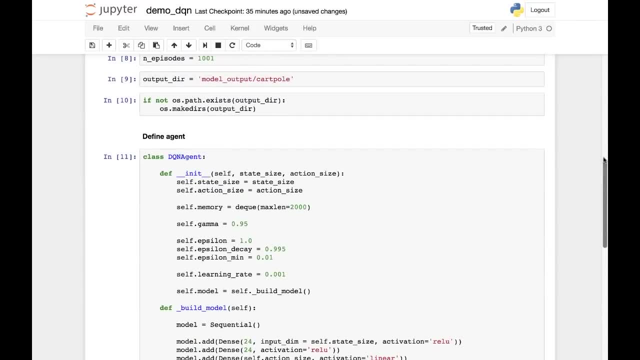 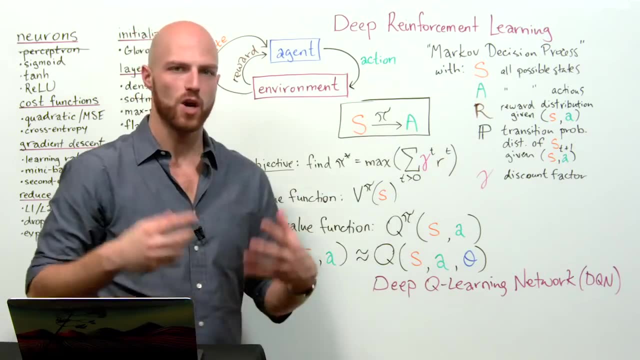 So there you have it. We have defined our DQNAgent. We're now ready to rock, to get our agent inside of the OpenAI Gym cart-pole environment and train it to perform well at the task to win the cart-pole game. 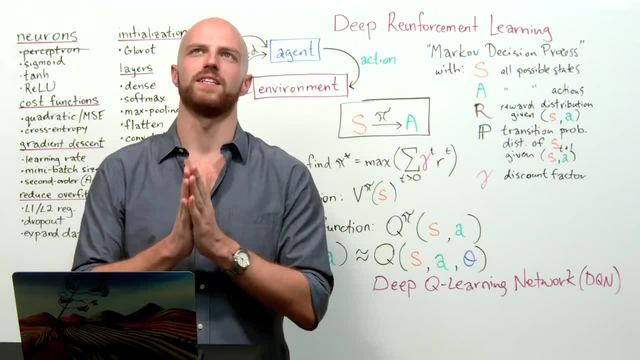 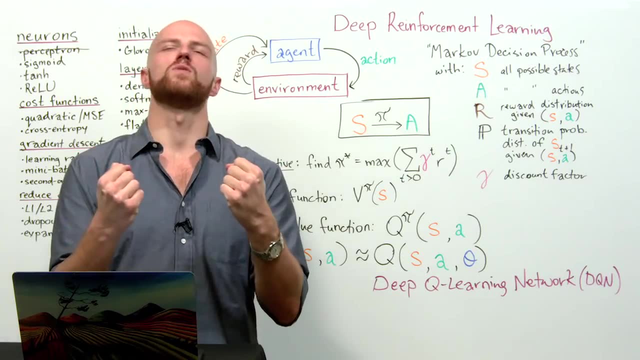 Yes, yes, yes, We are in the home stretch. We can finally do it. We have all of our theory in our pocket. We have our agent defined. This DQ learning agent is excited to play the cart-pole game. How can we do it? 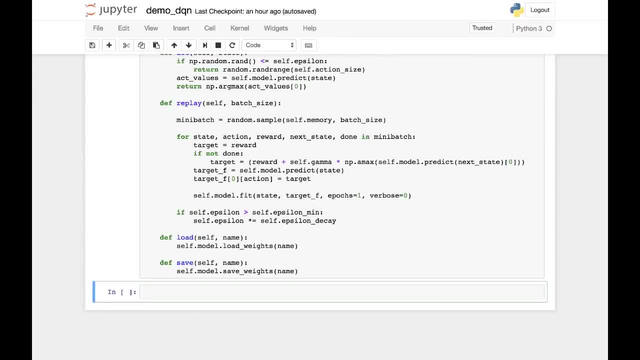 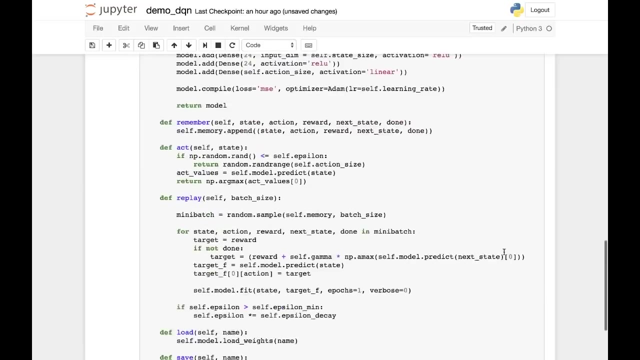 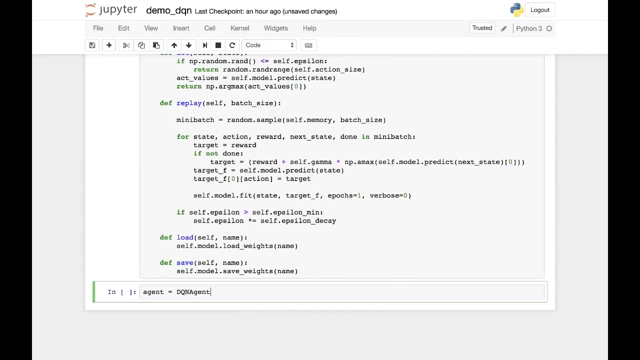 Well, here we go. So we're now going to interact with our environment. Let's define a particular instance of our agent. So we've got our agent class ready to go here And we pass into it only two parameters, which is the action size. 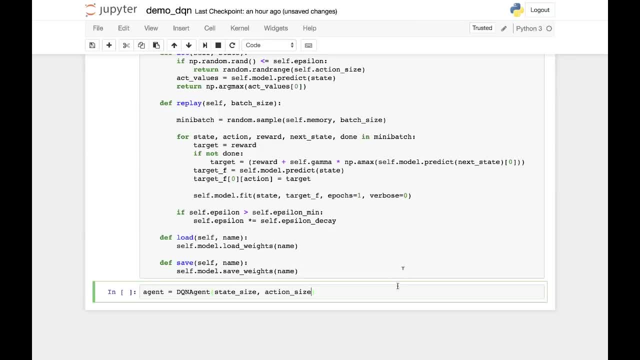 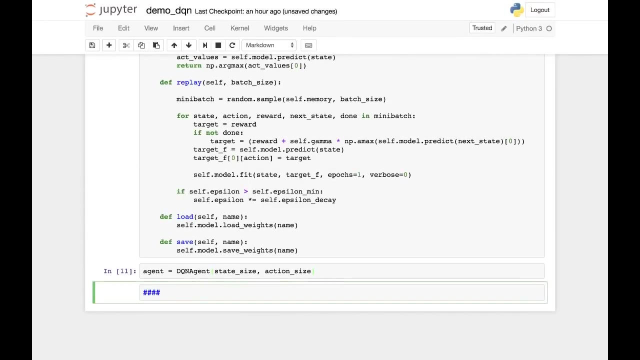 and the state size as we defined when we set up our class. So these are the four possible states of the game and the two possible actions, left or right, that we can take. Agent initialized And now we can interact with the environment. Nice little comment there. 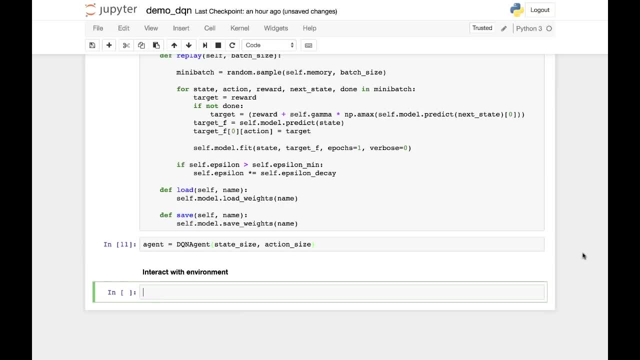 So we're going to start each episode- and our algorithm running in general- by saying that done is equal to false. So the default state is that the game episode has not ended, And then for each episode, in the range of the number of episodes that we selected. 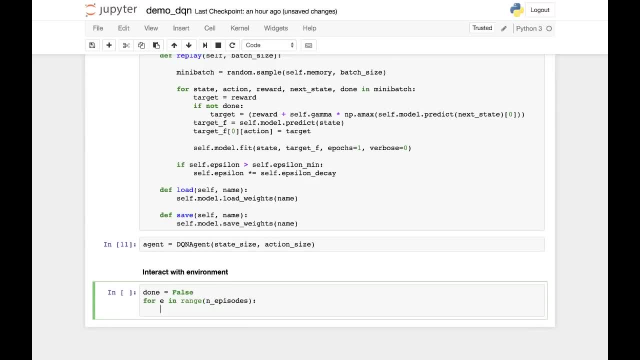 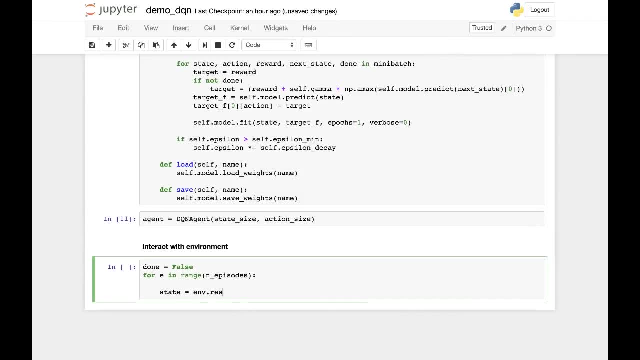 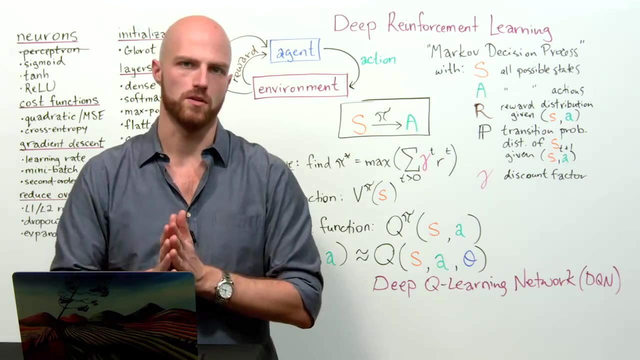 which was 1,001,. we're going to take the following actions. So, first things first. we're going to start with a reset state, So we're going to start each episode at the beginning of the episode, So in the card poll game. 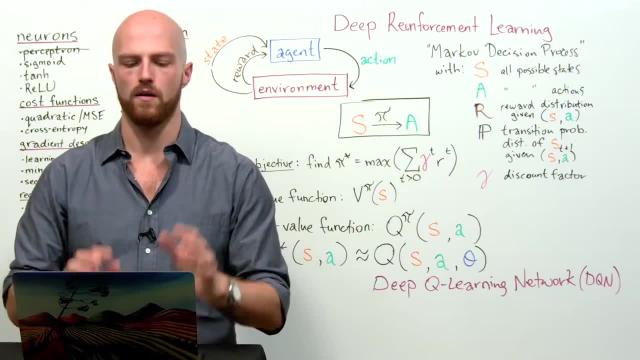 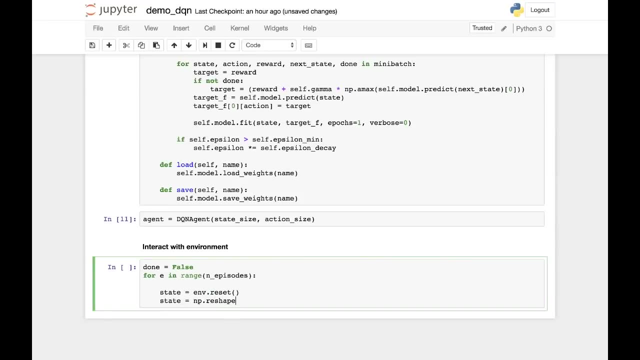 that's just a random starting position of the four possible states. Then we just reshape those states, We just flip them, transpose them so that they can fit nicely aligned with the deep learning network that we've defined in our agent. So we're not doing. 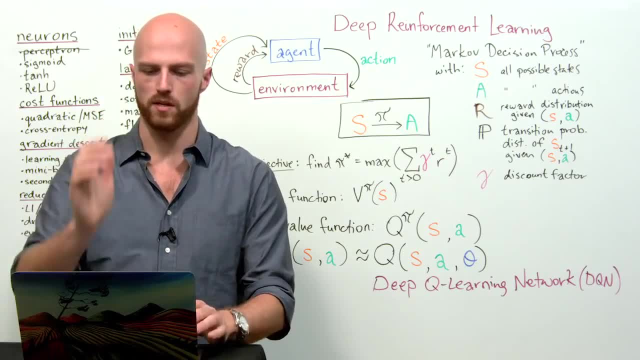 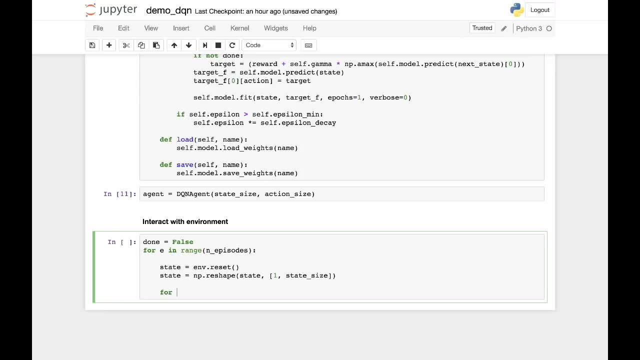 really any computation there, We're just flipping, transposing from Rotocom. Then we are going to iterate over time steps of the game So we can set a maximum number of time steps that our episode can run for. So I'm going to set that time. 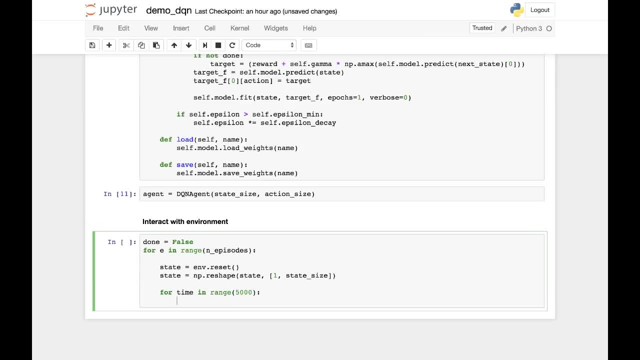 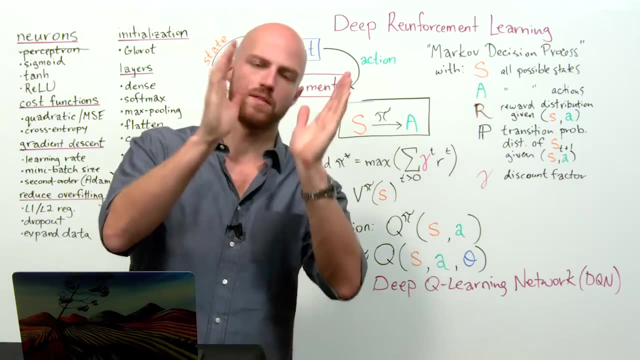 to 5,000.. So this means that if we manage to keep the poll alive, that the card poll doesn't tip too far, the poll doesn't tip too far off the card and the card doesn't veer off the screen. 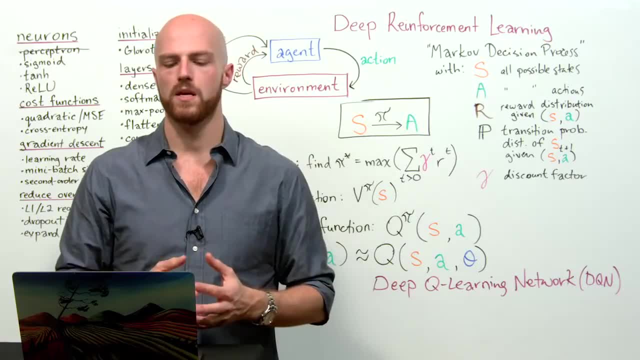 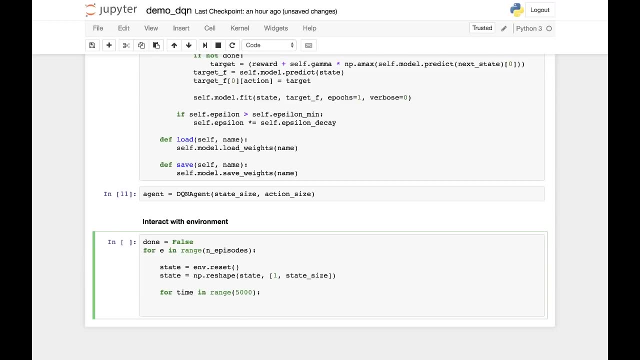 this means that the maximum game time is 5,000 time steps. Once we've reached that 5,000 time steps, we call it quits. anyway, The game can't go on for eternity. Here there's an option, So there's this. 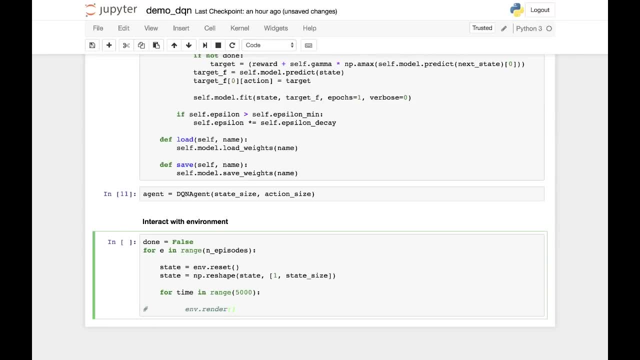 environment render function. I'm actually going to comment this out right now. So I'm running my Jupyter notebooks from within the Dockerized container environment on a cloud server, And that means that I can't render the OpenAI environment in the default way. 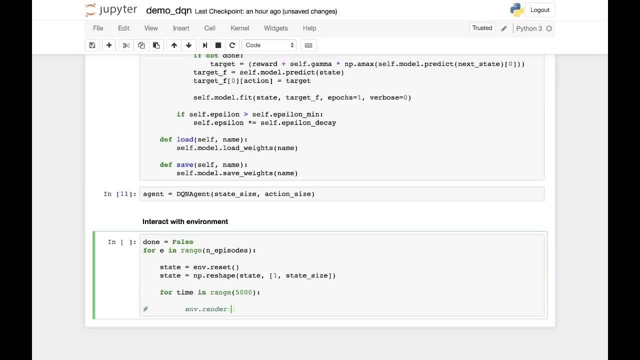 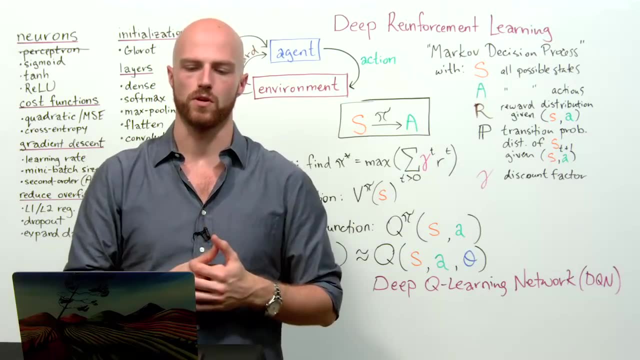 that it works. What it would want to do here is it would want to pop off a little Python video of the game in action, So it would render the game to our screen. But that doesn't happen in the Jupyter notebook. It happens externally. 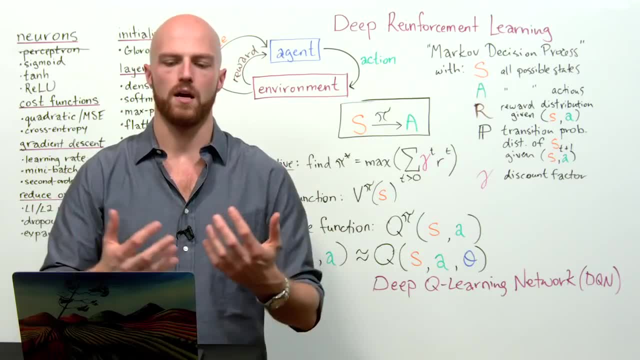 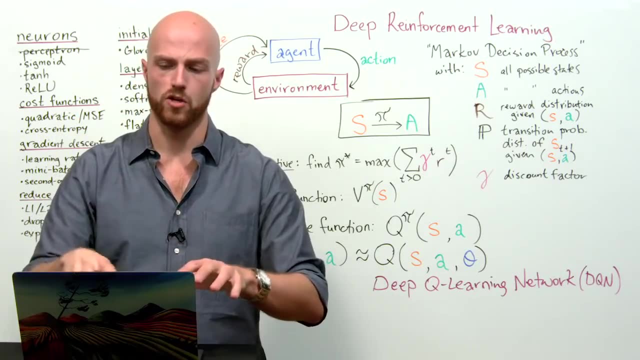 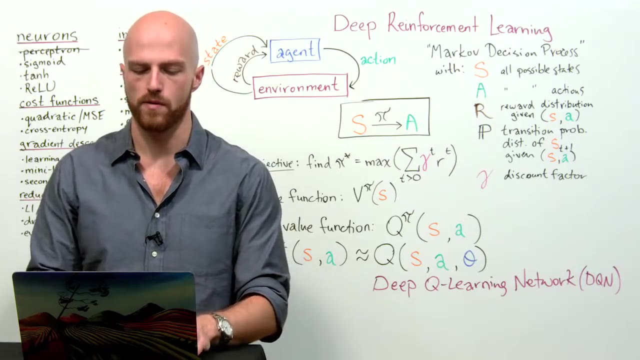 in this pop-out window, which isn't possible in this Docker container remote server situation. As soon as we get through this notebook, I will show you how I would do this on my local machine so that I could see the environment render. But for now, 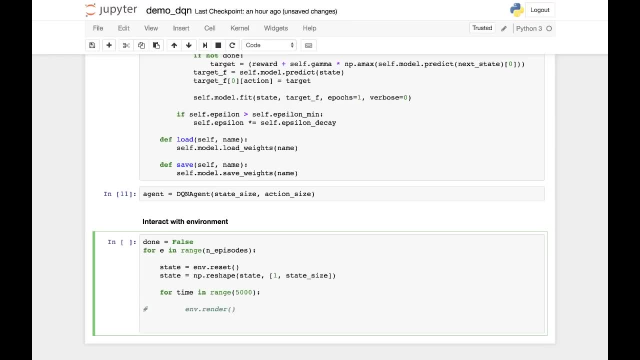 we'll just comment it out. So the next real step for us is setting. I'm just going to move this comment to a different spot here so that every time I press Enter I end up at the right indent- The first step in interacting. 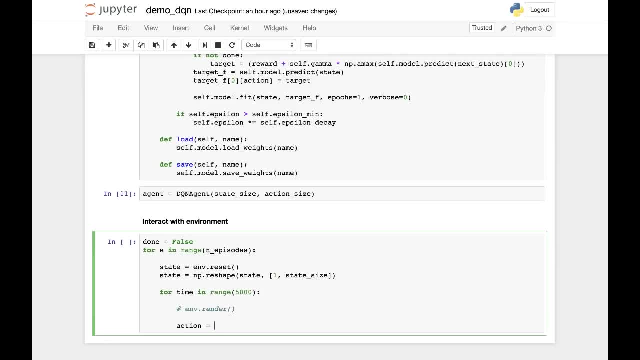 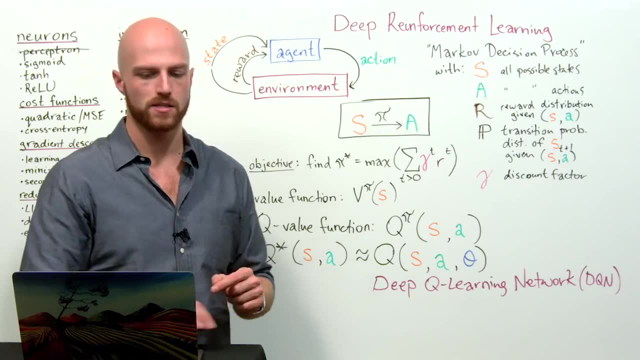 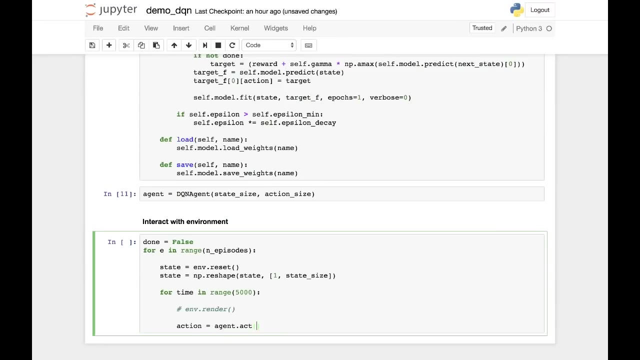 with our environment is to pass the current state. So we've initialized with a random starting state here And then we want to pass that starting state into our agent so they can take some initial action. So here we are. The action is going to be. 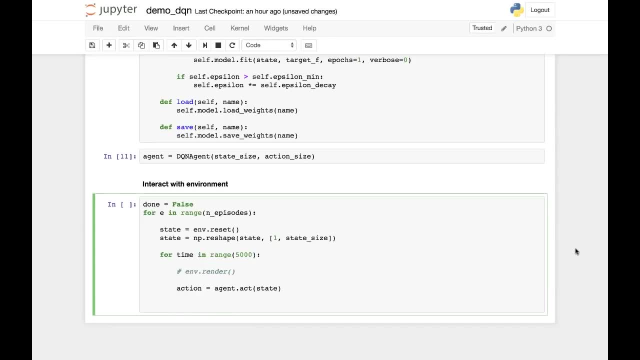 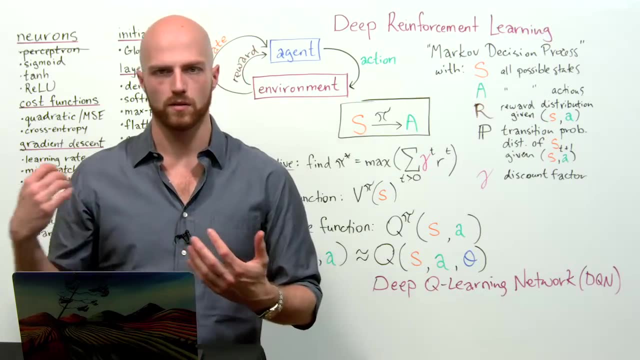 either a 0 or a 1, so it's going to be either move left or right At the beginning of the game. it's mostly going to be random guesses. It's just going to be exploring, But as it learns from its memories, 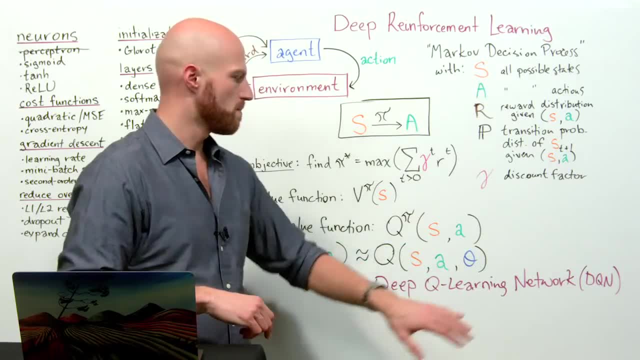 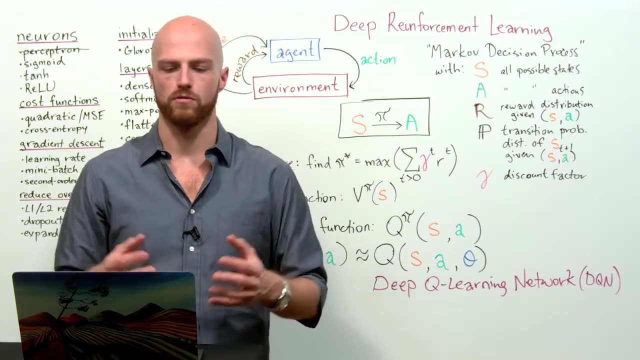 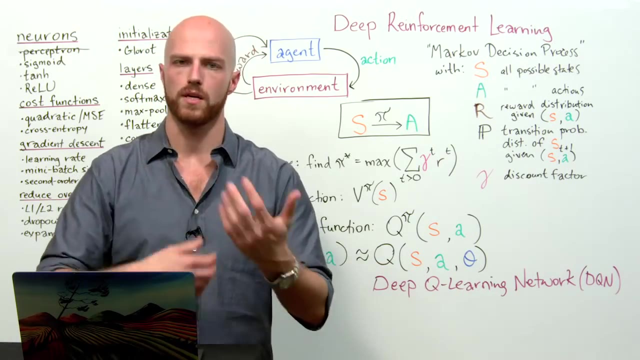 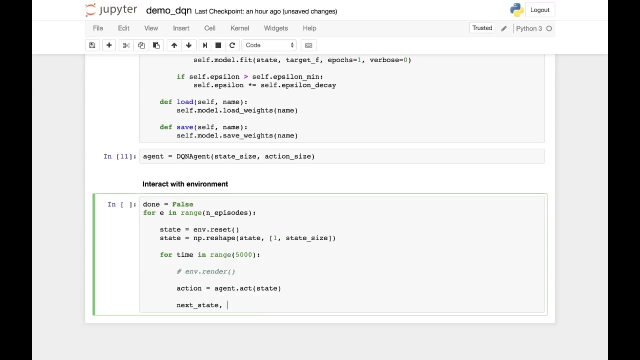 and these theta weights in our deep learning network become better and better at approximating Q star and optimizing our future reward. we will move towards exploiting that theta relationship that we're going to model and improve. So that's how this thing works. After our agent. 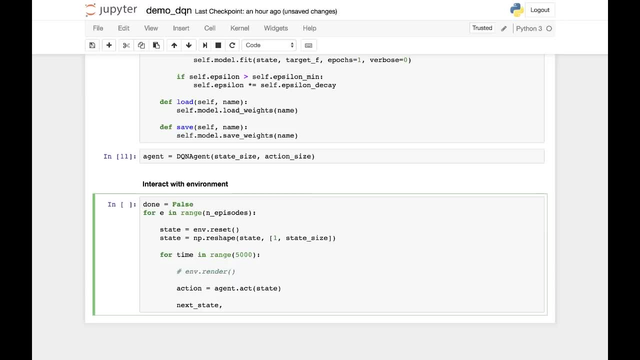 has taken an action, then we can use that action to pass to the environment and get our next state and our next reward from the environment. So let's do that with this step. So our next state, our reward, and whether the game is done or not, 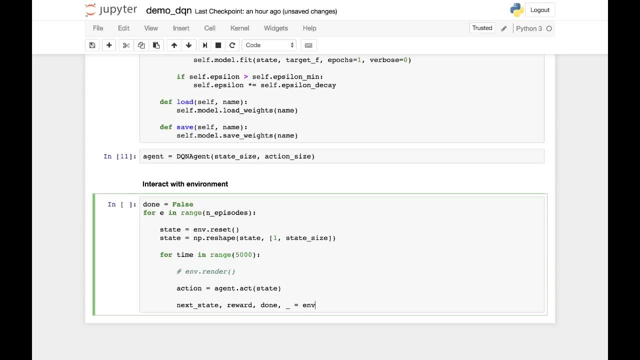 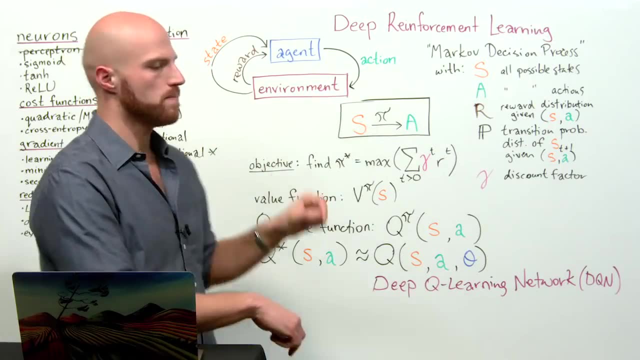 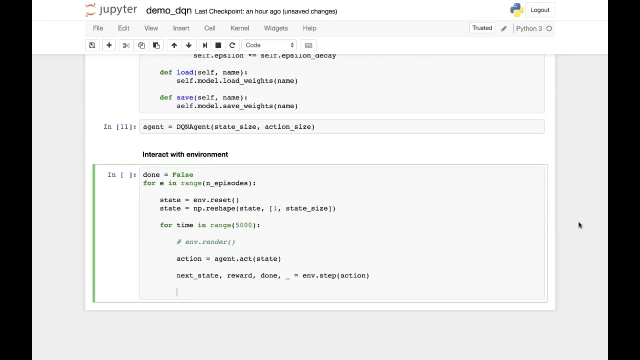 we take that out of the environment by taking a step forward. So we pass in the action into the environment. We get back the next state, our reward, and an indicator, a Boolean, as to whether the game is done or not. The next step: 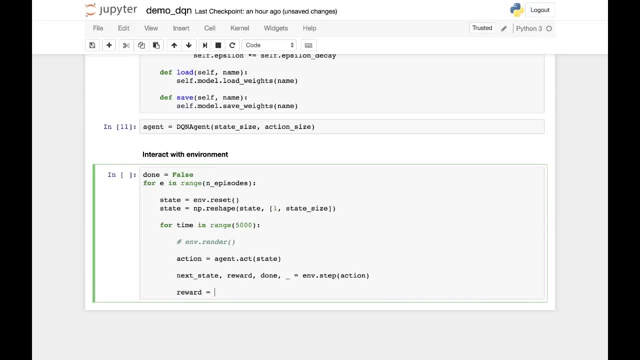 is to calculate our reward, So we can define this ourselves. So our reward is just going to be equal to the reward that the environment pops out as long as we're not done. Otherwise it's going to be a negative 10. So you get a penalty. 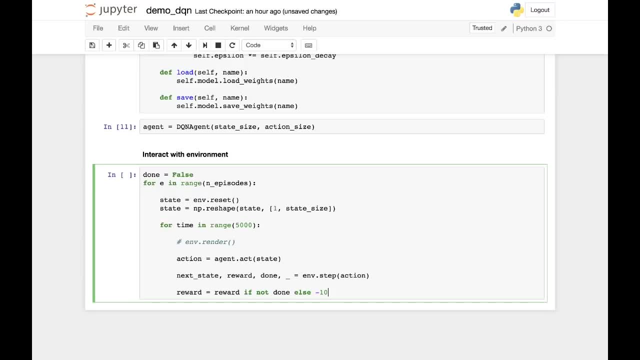 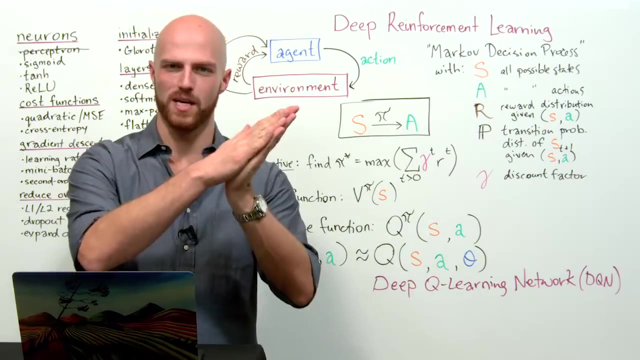 So if we manage to get to the 5,000 time step, our reward is related to the number of time steps that we were able to get through the game. But if we die, if the pole tips or if our cart goes off the screen, 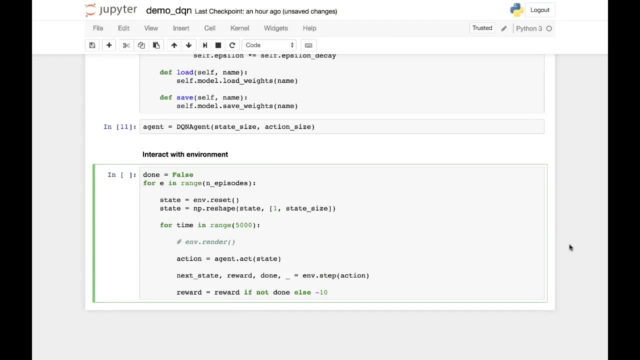 then the reward is negative 10.. So we penalize poor actions. In the next line of code, we're simply going to reshape our next state in the same way as we did above here, So I'm actually just going to copy and paste that code. 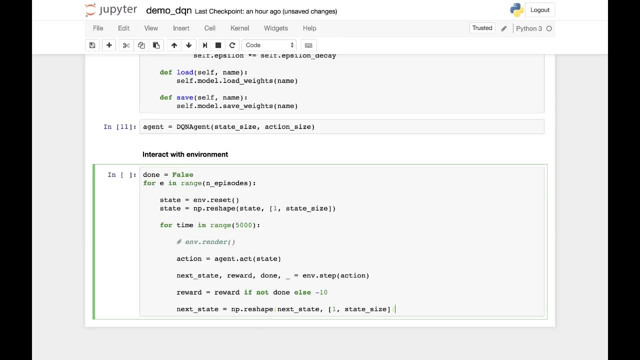 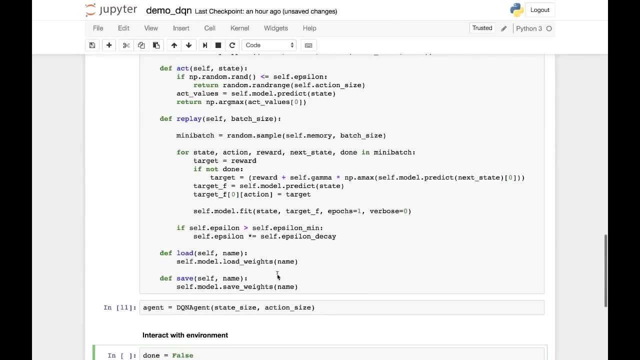 but it's going to be next state instead of state, And then we're going to use the remember method to remember the previous time, steps, state, the actions, the reward, all of the environmental stuff that we want to remember. So I'm actually just going to 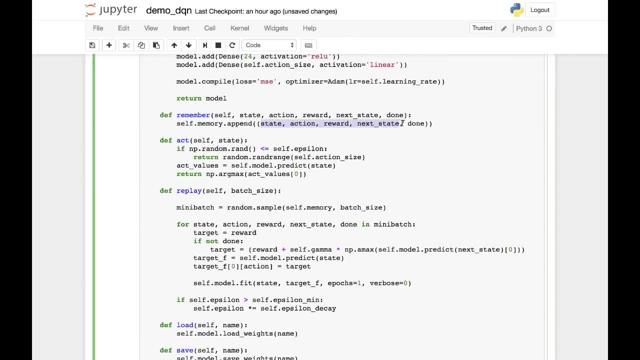 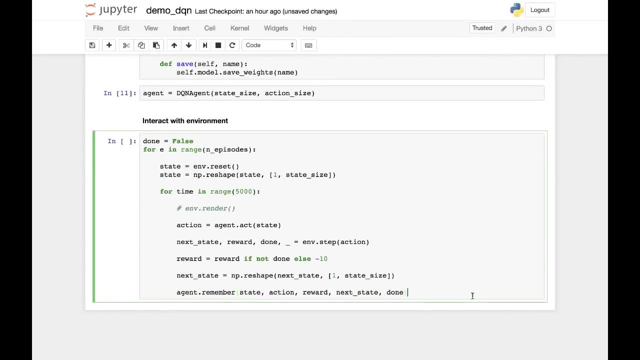 copy and paste that stuff: State action reward, next state done. Those are what we want to remember, So copy and paste them in there And then for the subsequent iteration, our state is going to be equal to what the next state was. 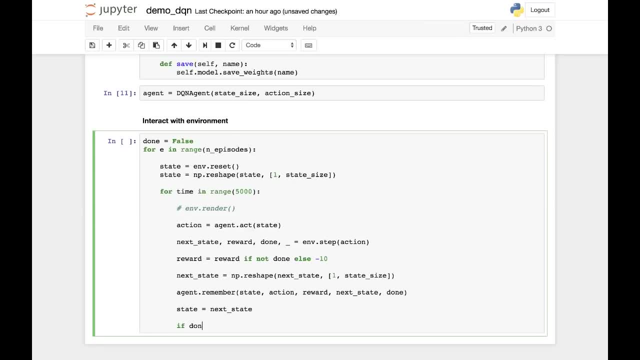 in the previous iteration. If we're done so, if the episode has ended, either because we've gotten to 5,000 times or because our agent has dropped the poll, then we're going to print out some metrics as to how the agent performed. 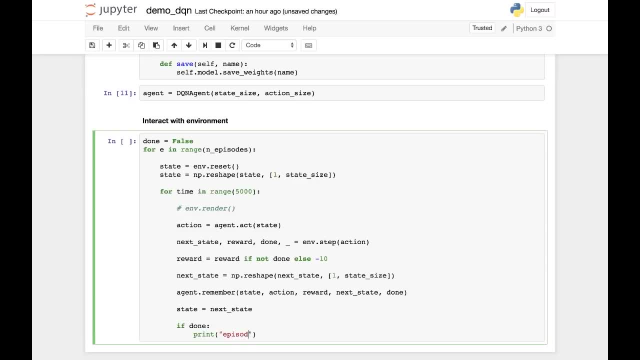 So we're going to print out the episode that we are at so we know how things are ticking along. out of all of the episodes- the 1,000 episodes that we're going to run this for, We're going to see our score and we're going to 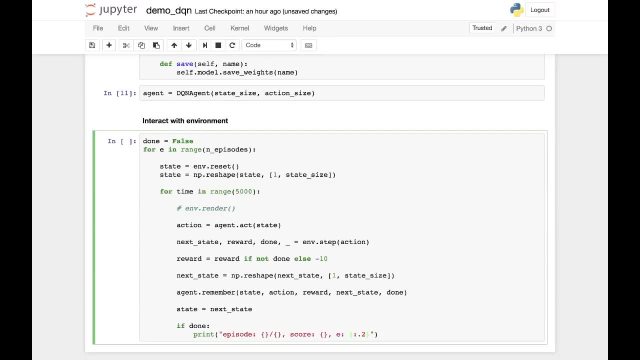 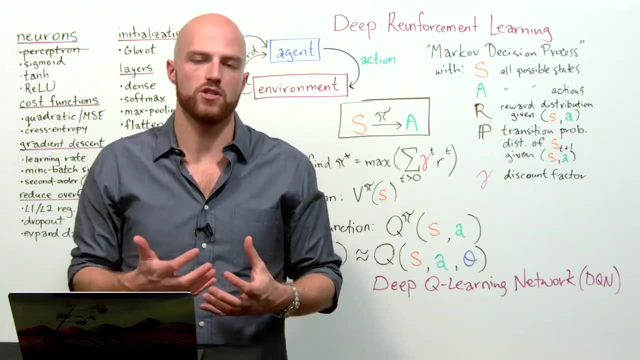 output the epsilon as well, so we can keep track of how the agent's exploration versus exploitation rate is changing over time. If we see that our agent is not performing very well, a good place to look for the problem is the epsilon, And so if we ran into issues here, 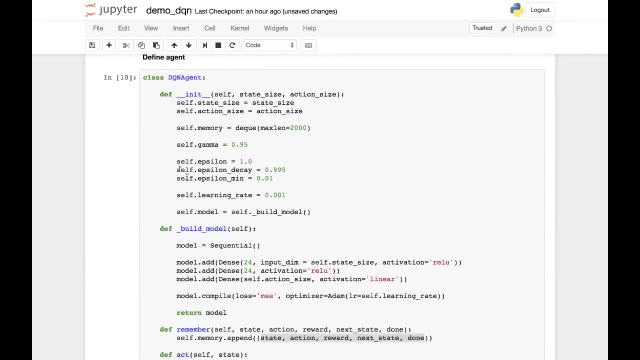 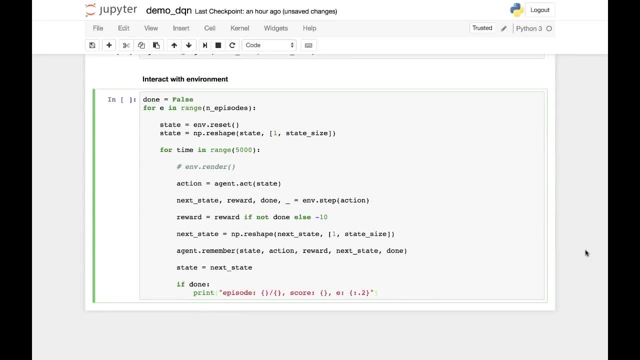 we could go back up and change aspects of our epsilon, maybe decaying more slowly or more quickly. But we're going to do this to improve our agent, And so this is just going to be outputting the episode. number of episodes, total time. 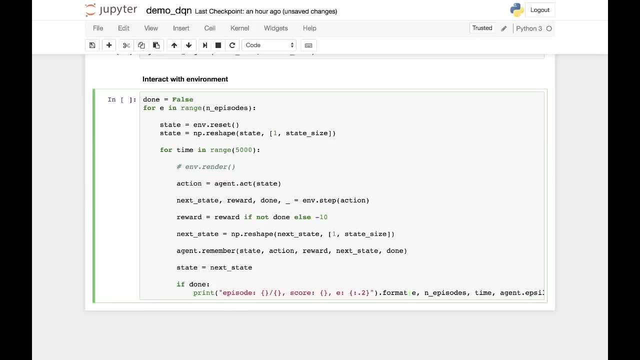 and the agent's epsilon, And then we exit the loop. The final step here is to actually train our theta. So we set up methods for doing that in the agent, but now, when we're actually interacting with our environment, we need to take some time. 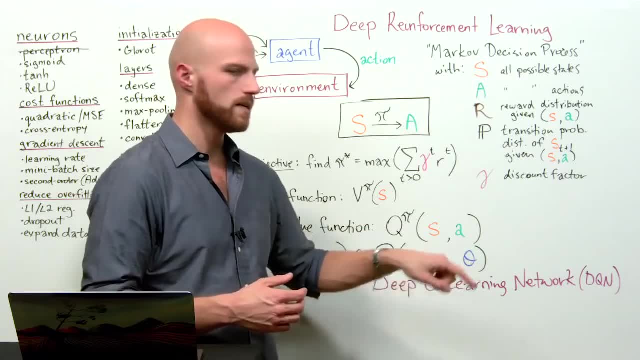 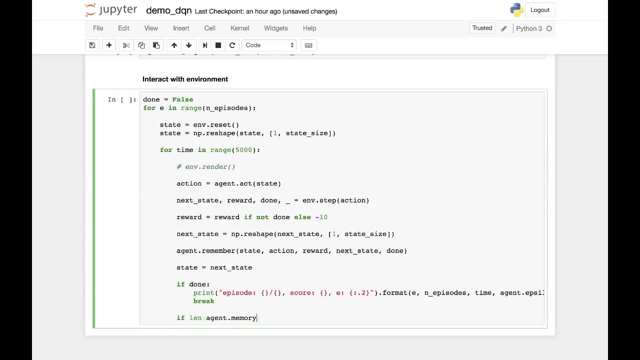 to give the agent a chance to update its theta weights so that it can improve for future iterations. So what we're going to do is that if agent memory is greater than batch size, then we run the replay method to sample our memory and replay some experiences. 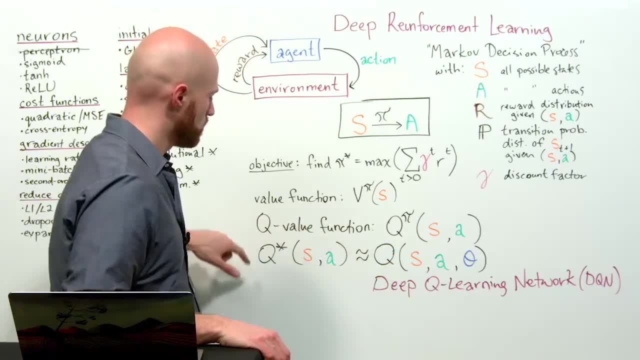 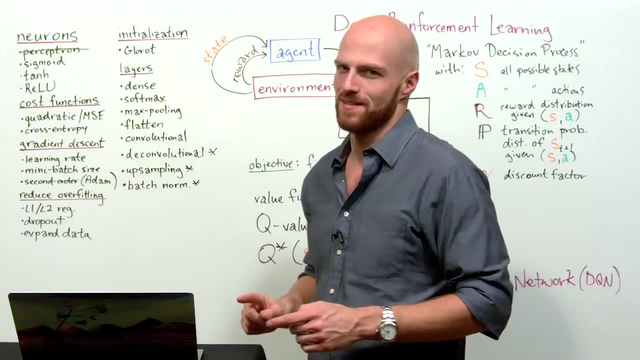 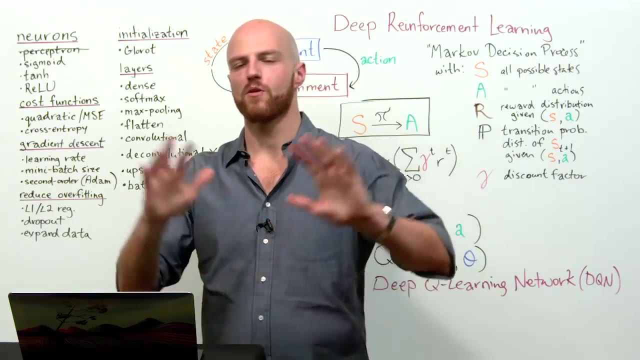 train our theta so that we can estimate q star and maximize a future reward more optimally. One interesting little side bit is that I've kept talking about throughout this example. I've been talking about gradient descent And throughout all of my live lessons. 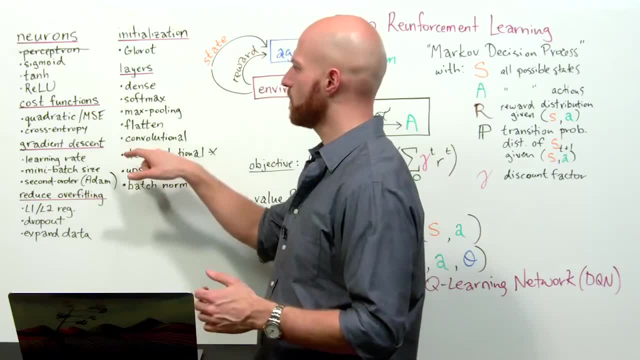 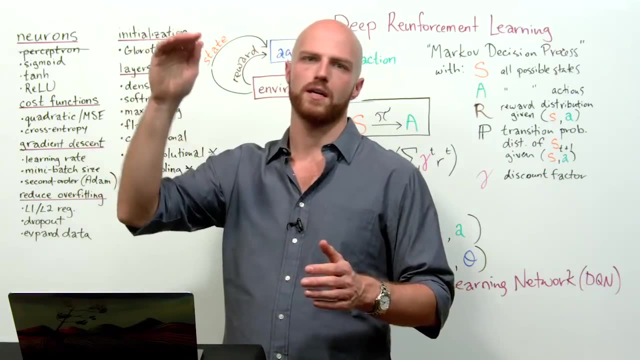 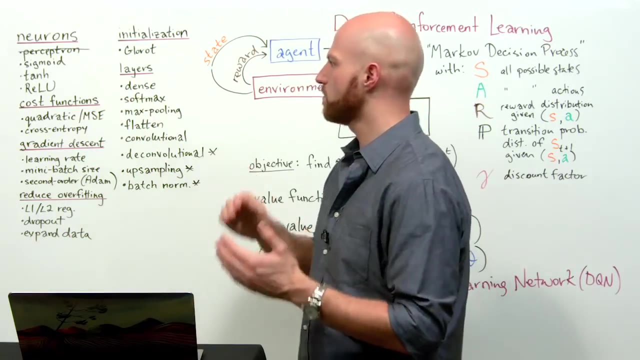 we talk about gradient descent. Now, interestingly, the reason why we call gradient descent descent is because we're typically talking about minimizing cost. So we're typically talking about finding a minimum value, a global minimum of cost that we're aiming to find. 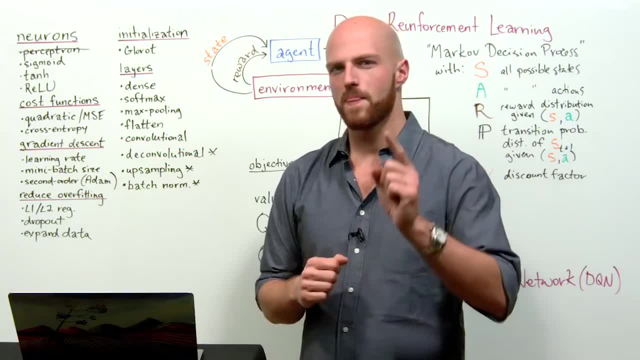 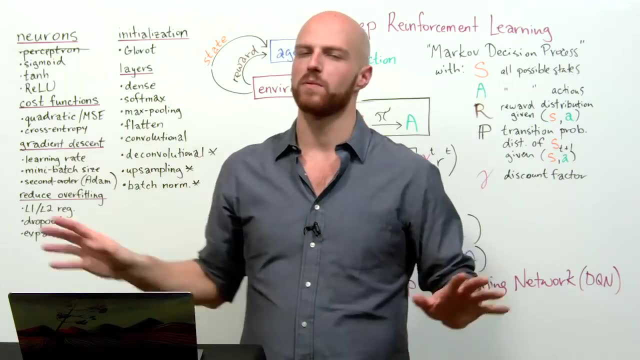 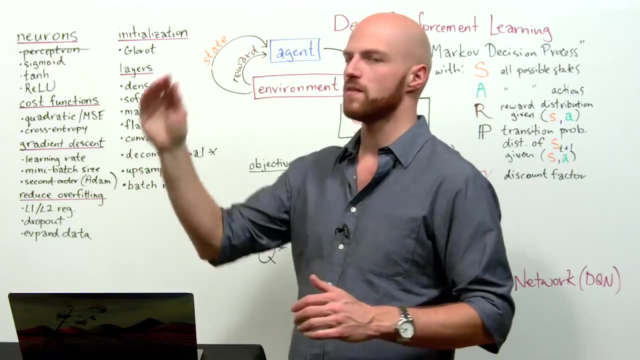 with our stochastic gradient descent. In this case, we're actually trying to maximize our reward, so the verbiage changes a little bit. Very few people are going to catch you out on this, but we're in fact using stochastic gradient ascent because we're trying to find 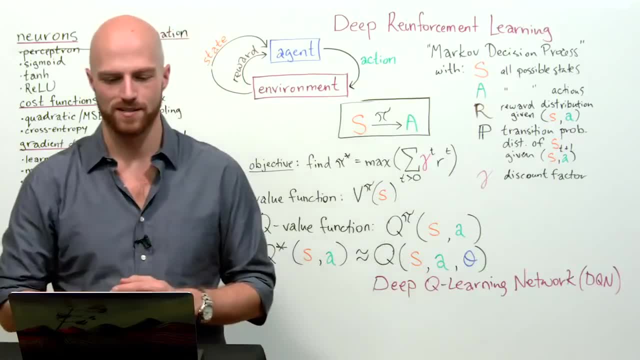 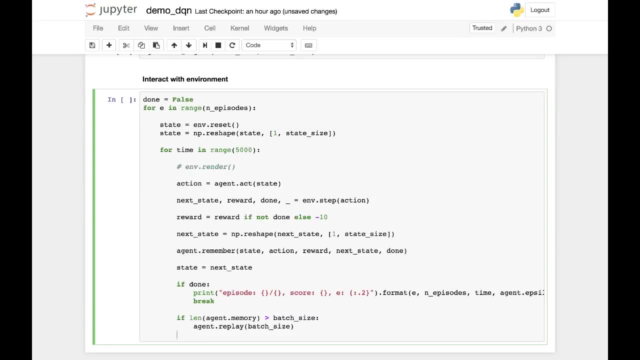 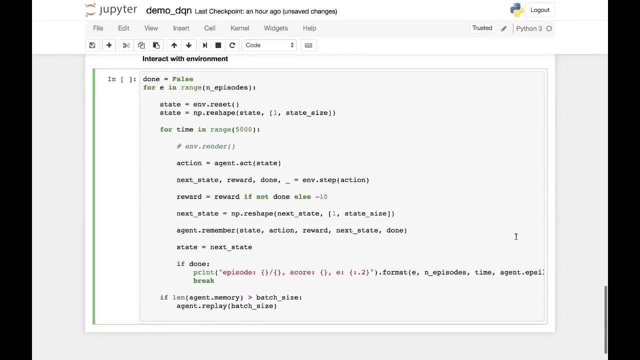 the optimal reward as opposed to the minimal cost. So just a tiny little piece of side information there, All right now. one last step that I want to take here is we need to drop the indent of this replay memory. We don't want that to happen. 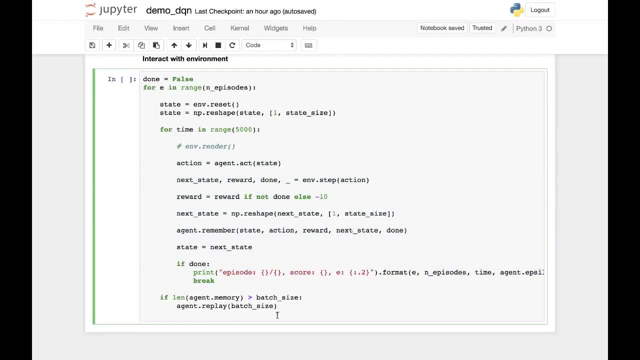 in this for loop, in the inner for loop, And the final thing that we want to do is use a modulo operator here so that every 50th episode we save out our model parameters, so that if we decide after watching the agent train for a thousand episodes, 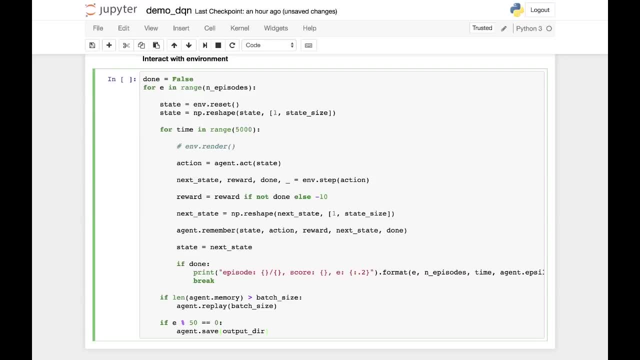 we might say. actually, you know what I didn't like: the model weights at the end of the thousand episodes. You know there was this part in the middle around episode 550 where the performance of the agent was best, And so those are the model weights. 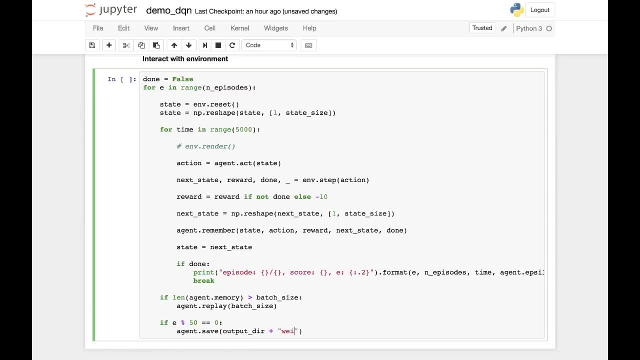 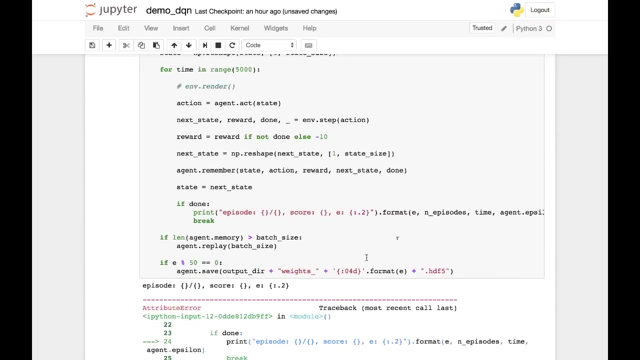 that I want to hold on to. So we're just going to output, specify the file name that we want and the kind of formatting that we want for that output. We're going to save it as an HGF5 file, All right. 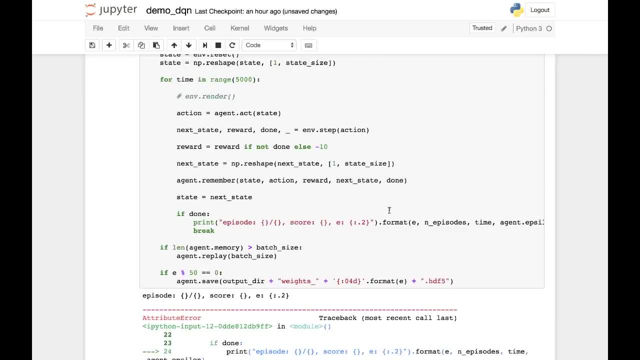 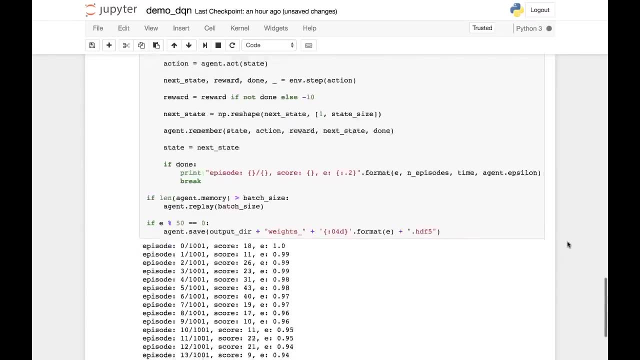 Of course I made some kind of typo here. Ah, my bracket is too soon, So there's no bracket here. The bracket happens at the end. Let's try to rerun that. There we go Now. everything runs perfectly. So we can see episode over episode. 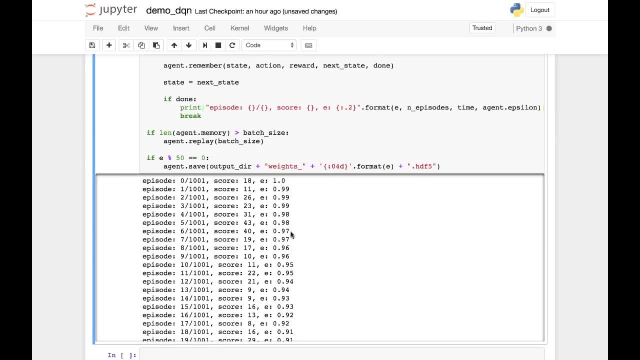 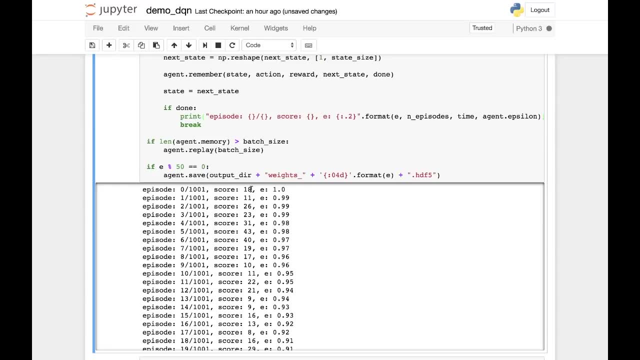 Our epsilon is decreasing, as we dictated it must, And we can see the score. So, on our very initial play of the game, the game went on for 18 time steps. We can see some slightly better performances here- 43. But in general we're mostly just exploring. 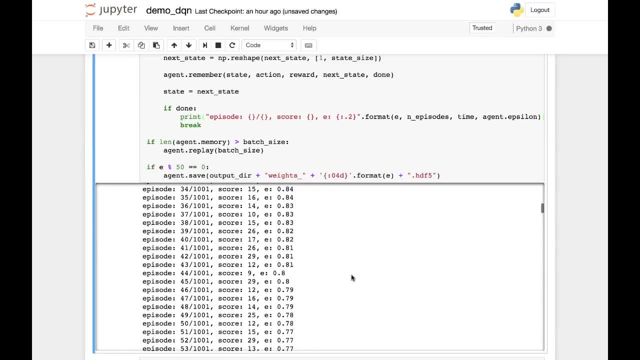 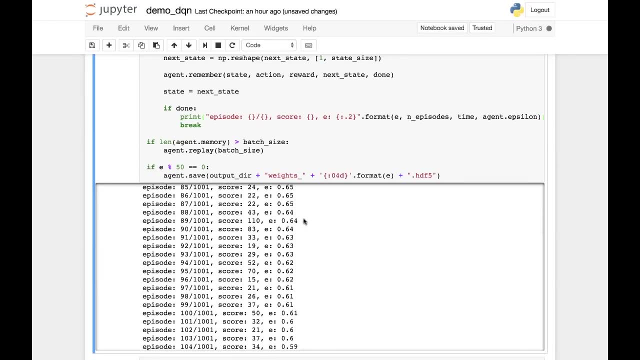 We expect in the beginning the agent not to perform very well. We're just using these opportunities to build up memories and to learn from those memories, But every once in a while. so here is an instance of the agent starting to perform relatively well. 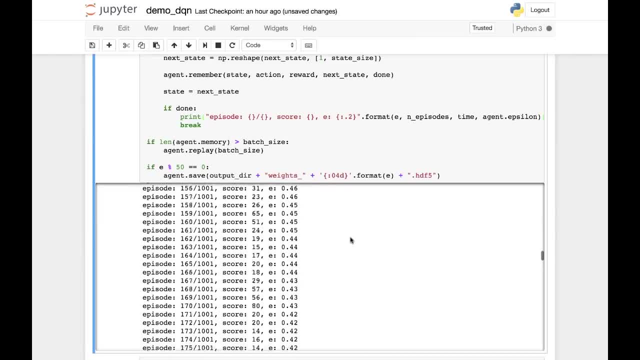 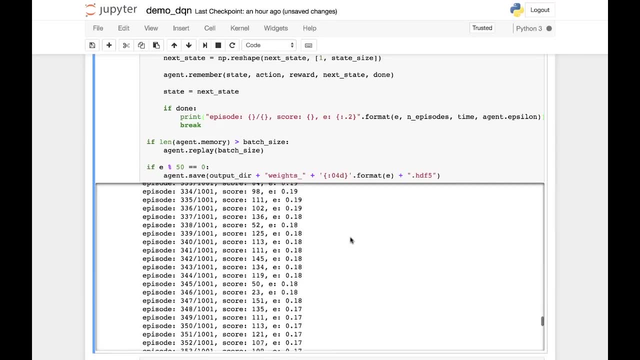 keeping the pole balanced for 110 time steps. And as we go on, we start to see that these numbers are generally now starting to be larger, And now, as we get into the kind of 300th episode, we're generally seeing almost all of the episodes. 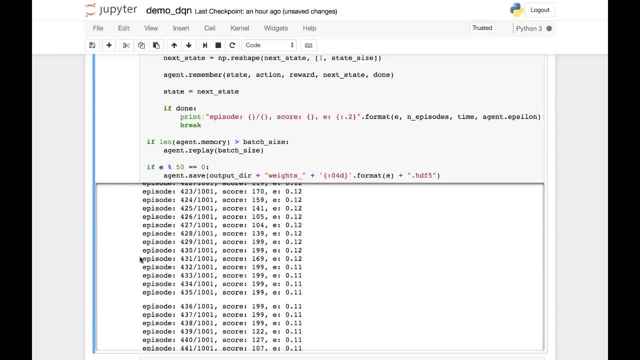 are lasting at least 100 time steps. And here we go. We can see we have this constraint. If you pick version zero of the cart pole game, there is this additional constraint that the game can only go on for 200 time steps. 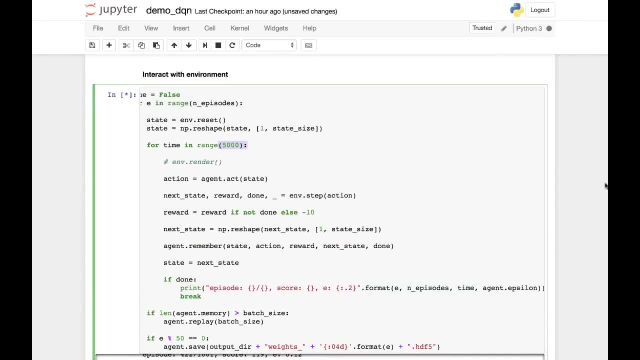 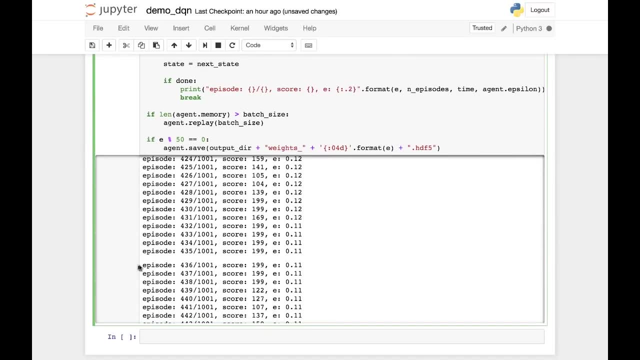 So it actually didn't even matter that I set this range to 5,000 up here. If you use version one of the game, the ceiling is higher, But so 199 is the best we can do, And so I think it's pretty safe to say. 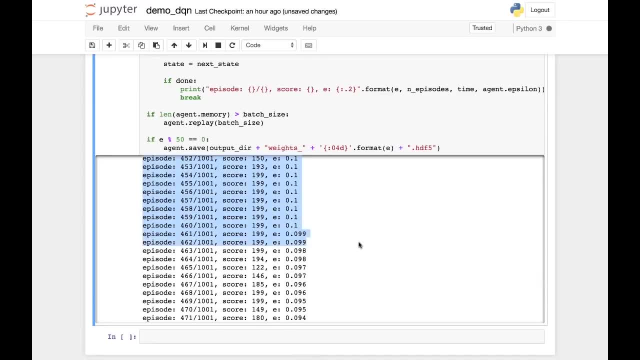 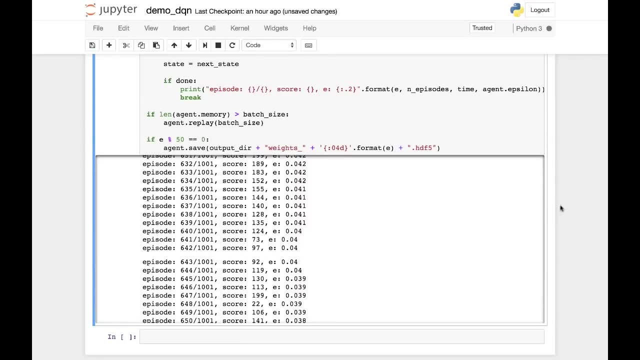 we have mastered the cart pole game here with this algorithm. Check this out. These guys are doing really well. Now there's one last remaining piece here that might be a little bit unsettling, which is that we might want to render the game and actually watch it in action. 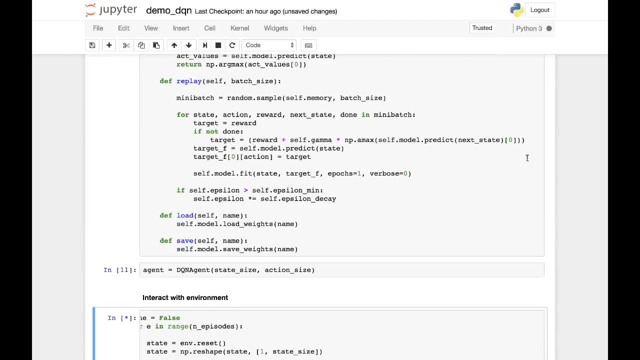 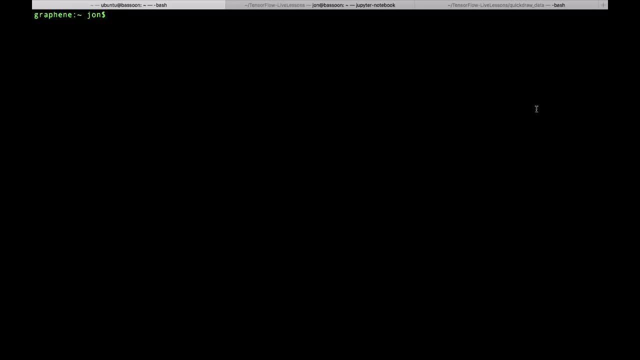 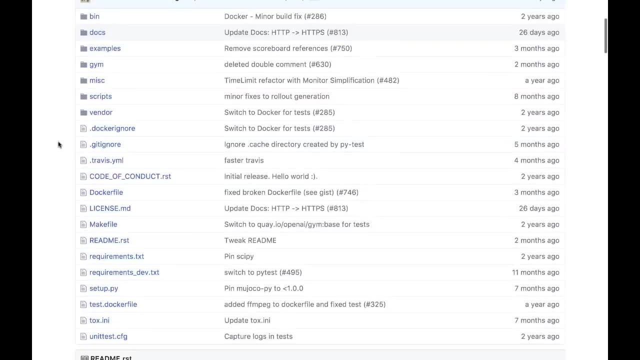 So to do that? that doesn't work within this Docker container environment as it's set up, but it can be done. So the way that we can do it is by installing on your machine the OpenAI GIM. So this involves following the installation instructions here. 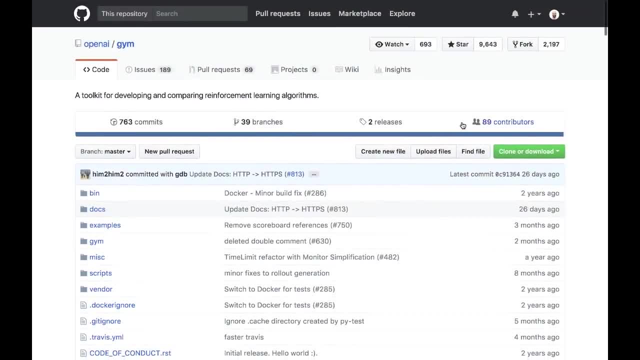 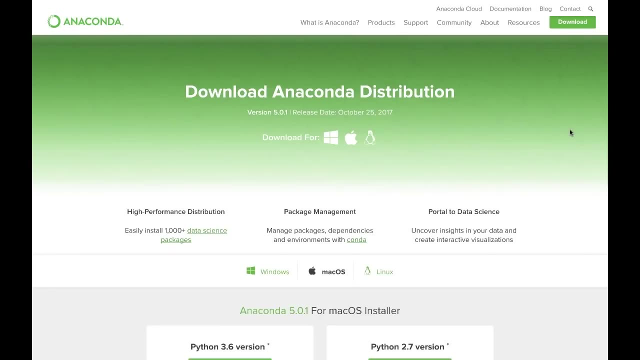 I believe, at least at time of recording, this will only work on Unix-based machines like Linux and Mac OS. I don't think you can do this natively on Windows. So after you've installed the OpenAI GIM, then you also need to install. 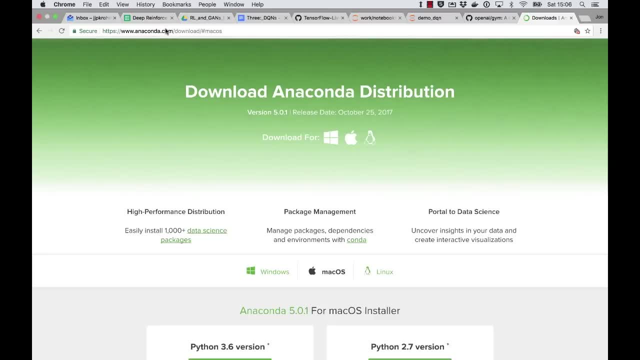 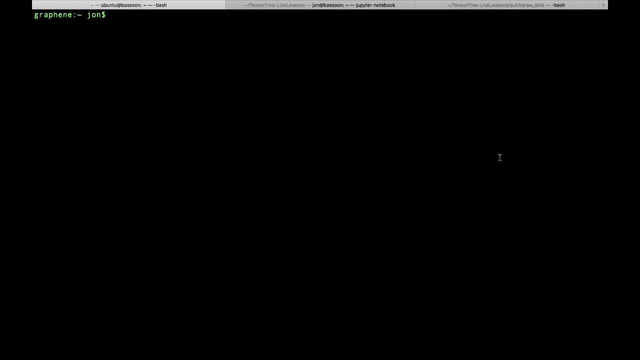 Anaconda, So anacondacom slash download. And then there were a couple little finicky bits, at least at the time of recording, related to the particular versions being used here. So I had to pip install the particular GIM that you want to use. 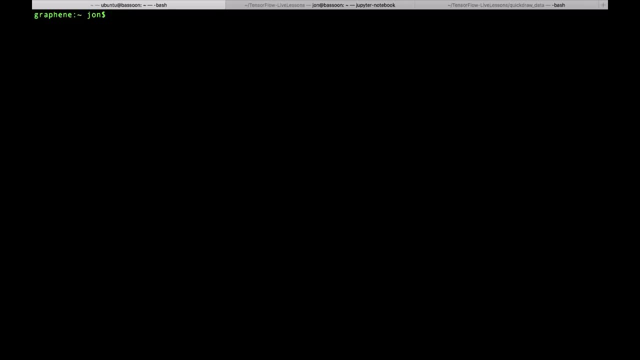 so like the Atari aspect of GIM and execute that. I'm just showing you the commands. I don't want to take the time of watching this install happen. And then the most unusual thing that I had to do was I had to pip uninstall. 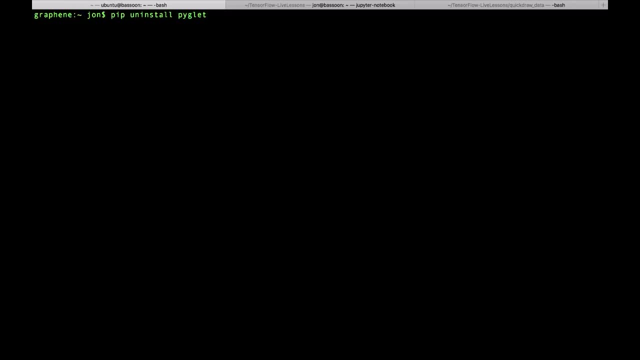 something called Piglet, which is used for rendering graphics, and then install an older version of it. So for me, the version that worked was this old version. 1.24 enabled me to render the OpenAI GIM environment And then so when I navigate. 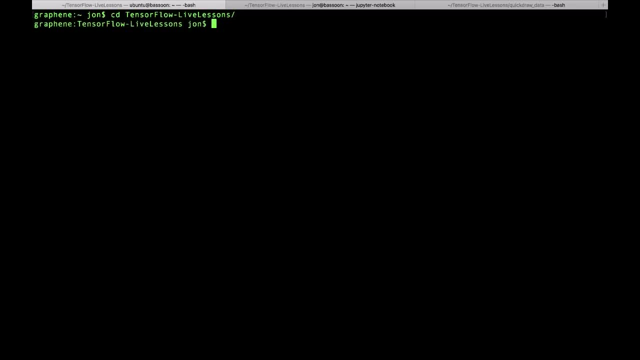 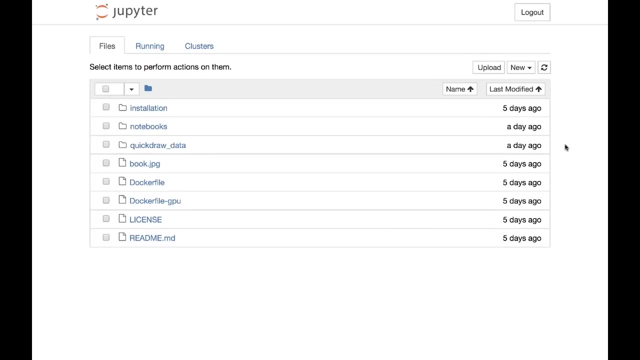 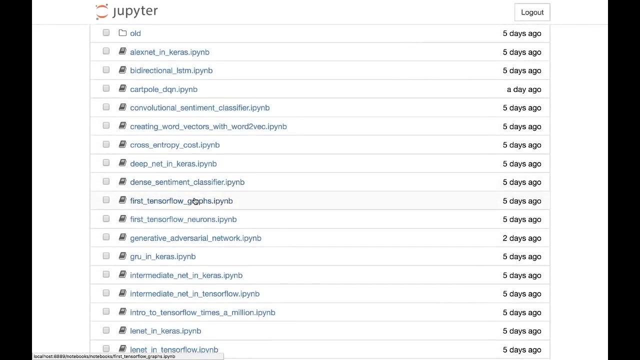 into the TensorFlow live lessons directory, I'm able to run the Jupyter notebook command which gives me a local version of this environment, And then in here we can pop into the completed code, the CartPol DQN code We can see in here: 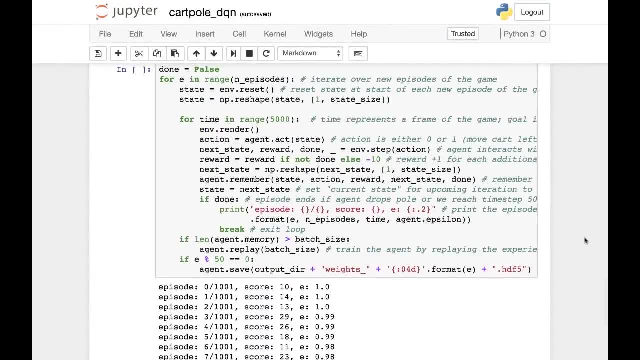 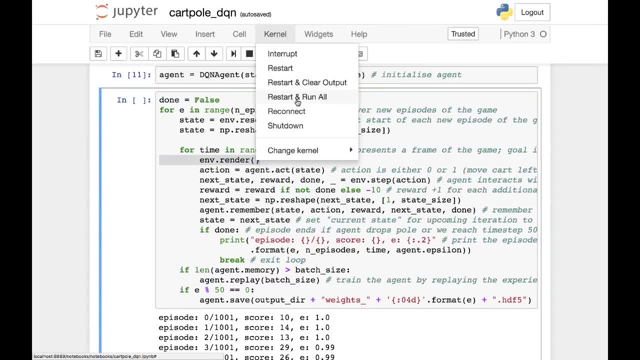 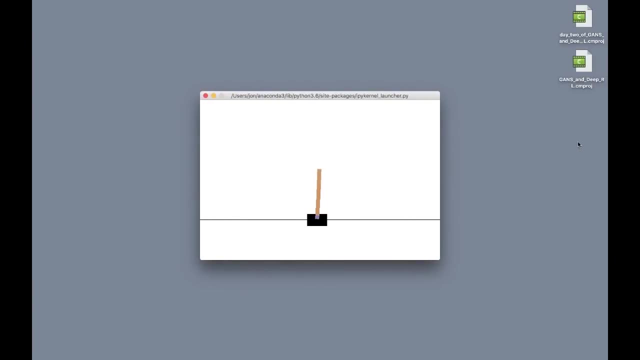 this is the same as the code that we just created for ourselves, except that the environment render is now uncommented, And so we can run this code now, And the Jupyter session pops us out into this IPython kernel and we can actually watch. 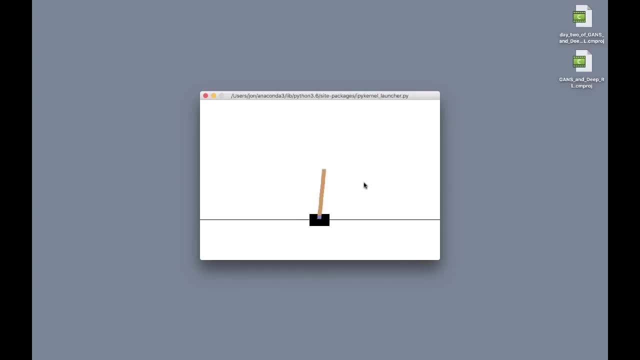 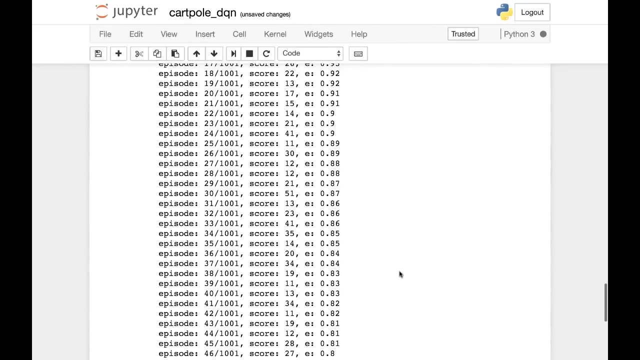 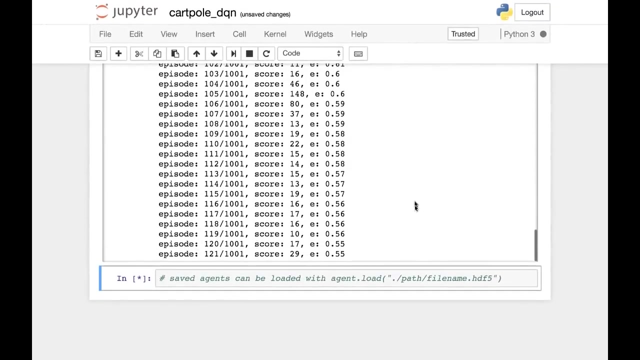 the algorithm now train. So you can see that as the algorithm gets better and better, as our deep learning agent gets better and better at performing in the environment, over time you'll start to see the poll be balanced for longer and longer sessions Here at the beginning.